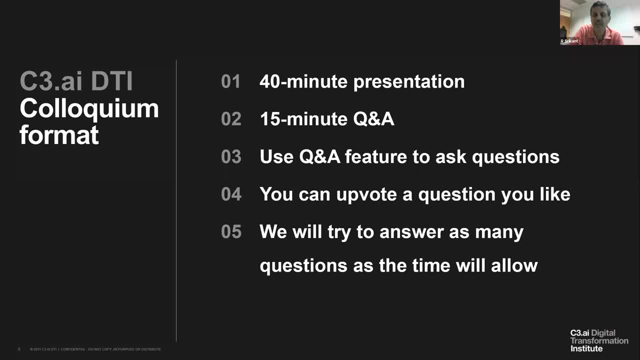 briefly talk about the format. We're changing the format a little bit for today, so the speaker would like to have questions during the presentation. So if you have any questions, please put them in the Q&A feature and I will read it out to. 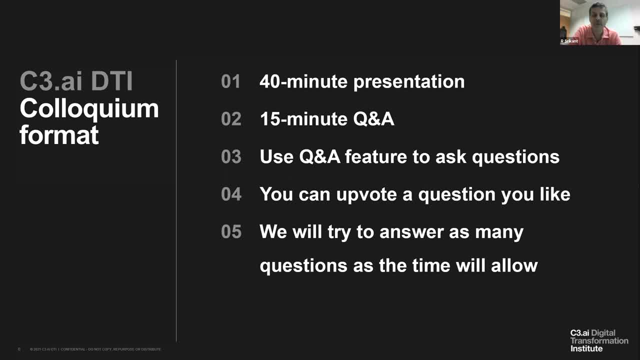 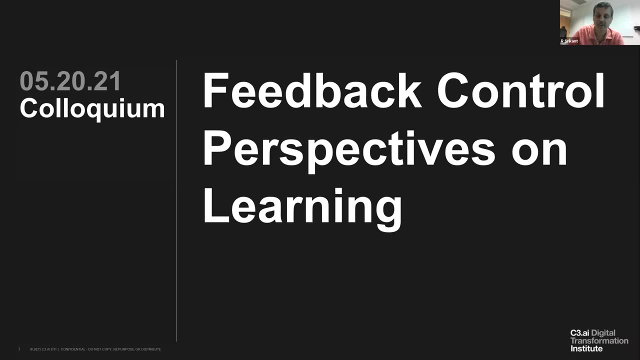 him whenever there's a pause in his talk. You can upload a question if you like, and we'll try to answer as many questions as time permits, but we'll ask the ones that are uploaded first. So today's talk is on feedback control: perspectives on learning. 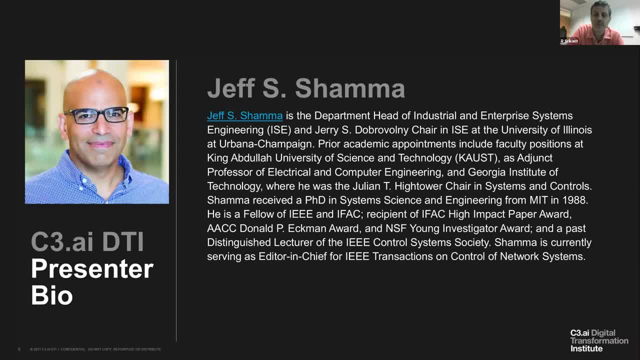 And the speaker is one of my distinguished colleagues, Jeff Schama, who is a very well-known control theorist, who is the department head of industrial and enterprise systems engineering here at the University of Illinois and he also holds the Jerry S Dobrowolny Chair in. 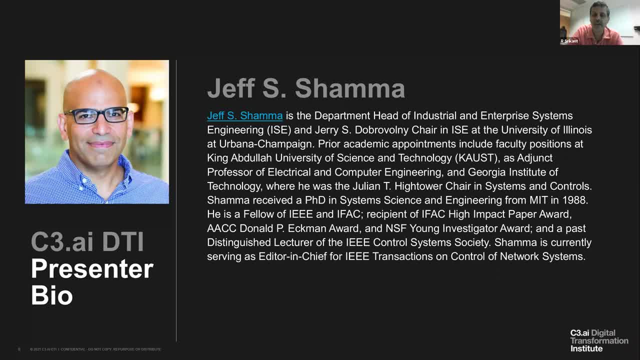 ISC. He has been a faculty member at a number of places, most recently at KAUST and before that at Georgia Tech and then at UCLA and so on. He received his PhD in system science and engineering from MIT in 1988. 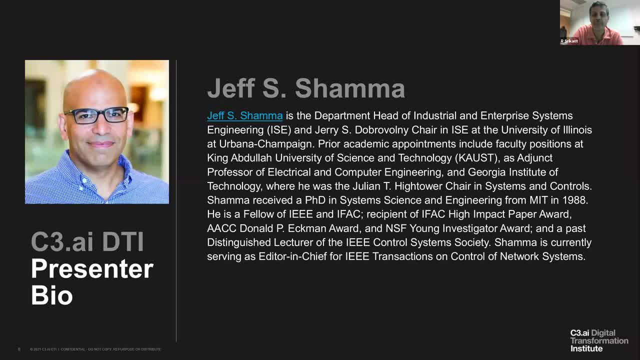 He's a fellow of the IEEE and IFAC. he's a recipient of the IFAC High Impact Paper Award, the prestigious Donald Ekman Award, the NSF Young Investigator Award, and he has been a past distinguished lecturer of the IEEE Control Systems Society. 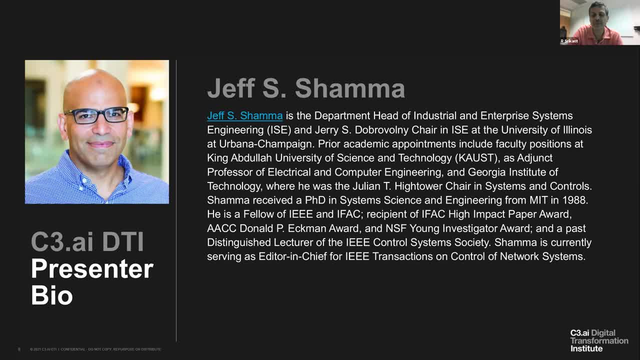 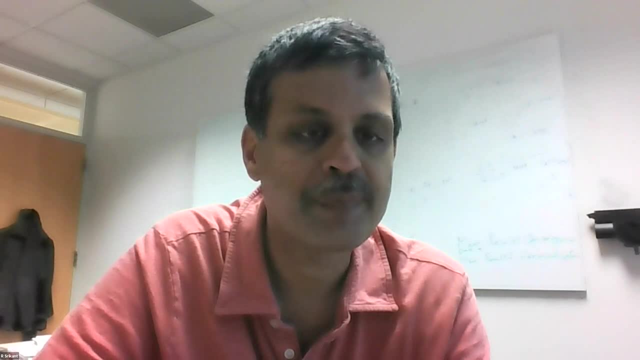 Jeff currently serves as the director of the IEEE Control Systems Society. He serves as the editor-in-chief of one of the two flagship journals of the Control Systems Society: the IEEE Transactions and Control of Network Systems. Jeff, without further ado, I'd like you to take the stage. 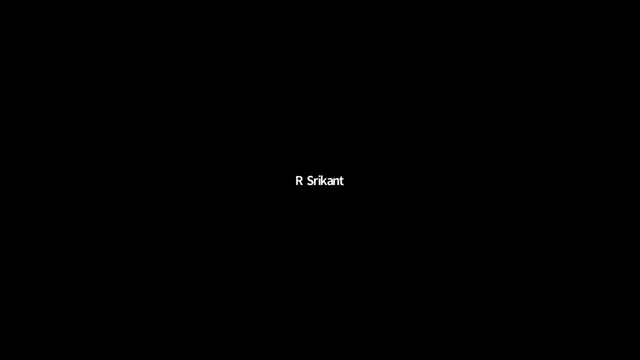 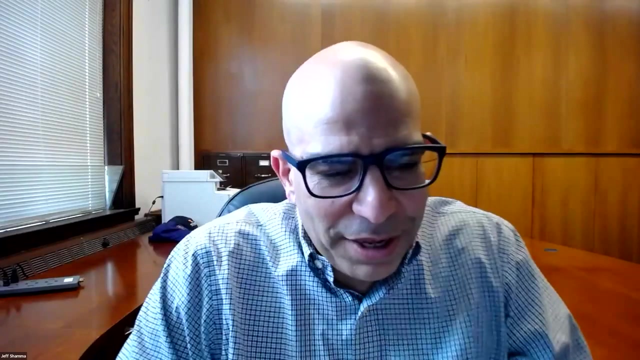 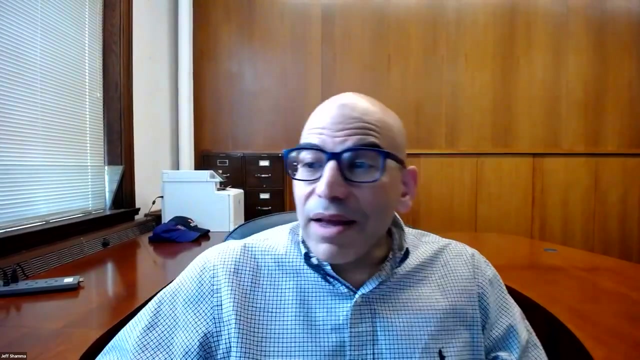 JEFF SCHAMA. IEEE Control Systems Society. IEEE Control Systems Society. IEEE Control Systems Society. Commander. Ok, thank you, Shrikant, for the invitation and the opportunity to participate in this colloquium. Did I share the right screen Or not yet? 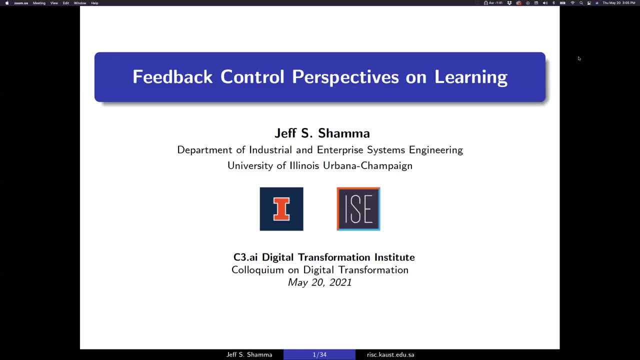 SHRIKANTYA MOHANDANI. Yes, Here we are Alright, very good. And yes, I'm glad to be a part of a colloquium and I look forward to the interactions. and, as Shrikant mentioned, yes, I'll welcome questions throughout the talk. 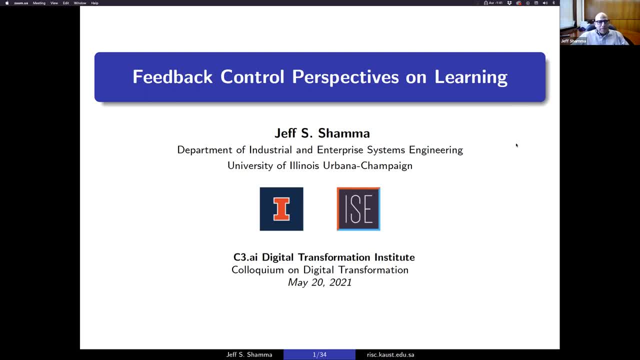 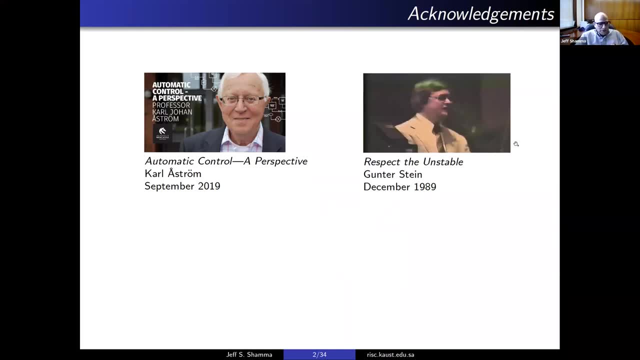 Here we go with the Jason Jr Episode Large in Time with Keith Ungerich. �uh Okay, so the title of the talk is Feedback Control: Perspectives on Learning, and first I'd like to start with a couple of acknowledgements, and these acknowledgements are pointers to videos that you can find online. 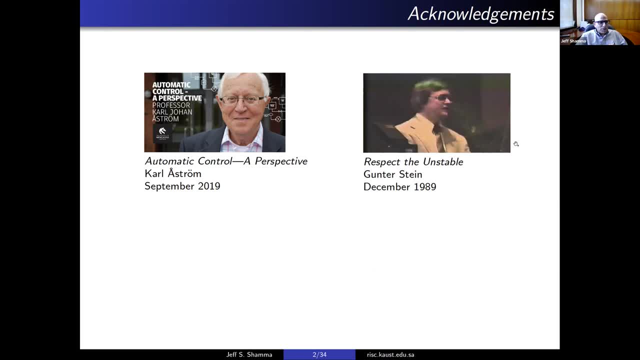 One of them is Automatic Controls of Perspective by Carl Ostrom, and this particular video is from September of 2019, and the other video is called Respect the Unstable, from Gunther Stein, and that's from way back in December of 1989. 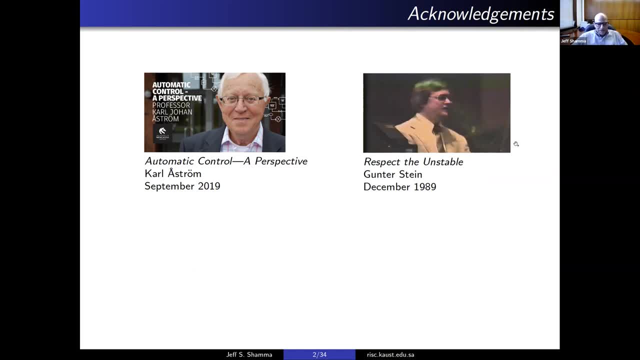 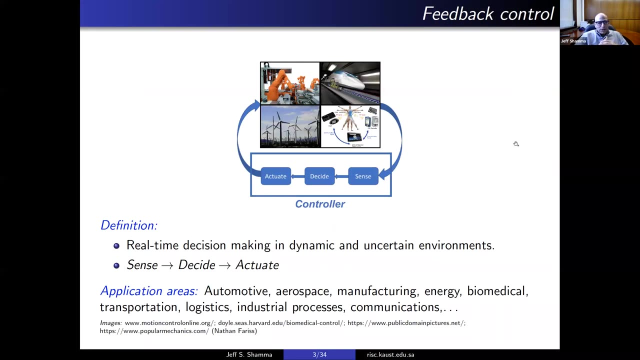 Again, both are excellent and highly recommended, and they've influenced today's slides Also. I'd like to acknowledge a handful of folks who helped give valuable comments to put together the talk as well. All right, so the title of the talk is Feedback Control- Perspectives on Learning, and so I'd like to first start with grounding my view of feedback control. 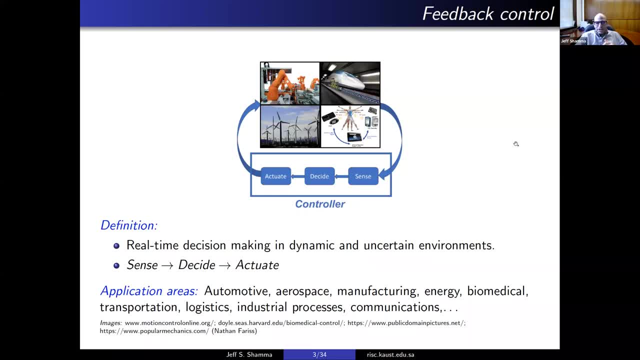 And so if I had to give it my own definition, I would call it decision-making In dynamic and uncertain environments, or interacting with a particular environment. we'd like to this environment to behave in a certain way to realize a desired effect. And so what we do? we measure what the environment is doing, take a decision on what to do and then actuate on that act on that decision, using our different ways to influence this environment. 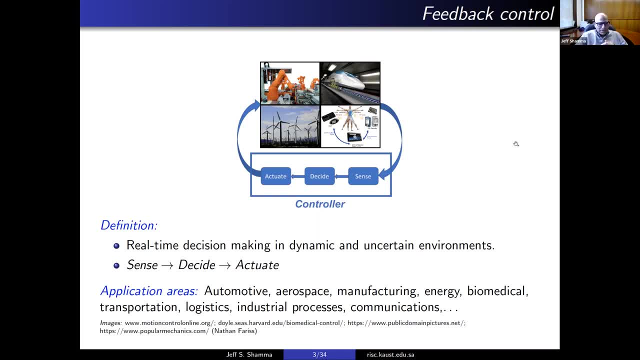 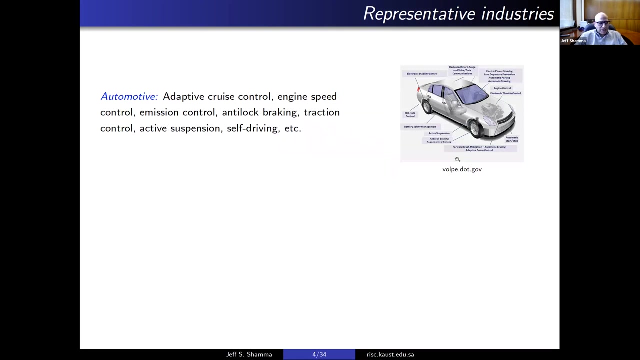 And so there's feedback control everywhere around us, and it's been applied in a whole variety of application domains: Automotive, Aerospace, Manufacturing, Energy, Logistics, Processes, Communications, You name it. feedback control has been applied. Two industries where it has had a lot of interaction is: one is the automotive industry. 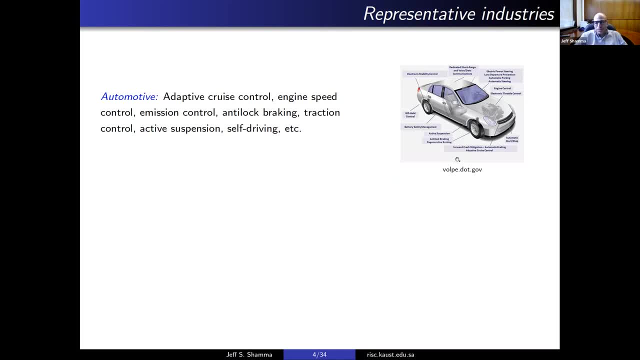 And so here I'm showing a picture of a car, a vehicle, but actually there's many, many feedback control mechanisms in any individual vehicle. So we're probably all familiar with cruise control, And now it's adaptive cruise control which will modulate the distance between your vehicle and the vehicle in front of you. 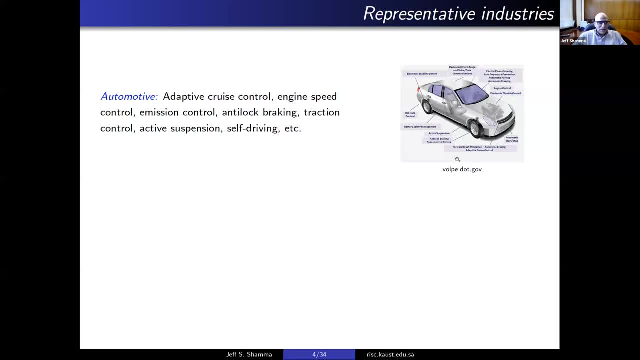 But there's actually control, feedback, control throughout a vehicle, controlling various aspects of suspension and engine and idling and braking and traction, and what have you? Another industry where feedback control has played a major role is in the aerospace industry, And so here I have a picture of the X-29 aircraft. 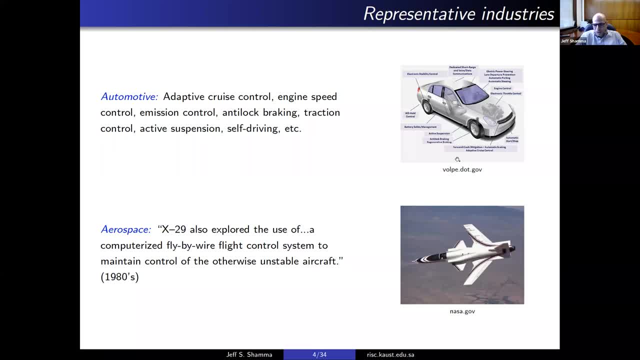 It was an experimental aircraft, And you'll notice that The wings are swept forward in this aircraft, And so here's a quote from the NASA website: The X-29 explored the use of computerized fly-by-wire flight control to maintain control of an otherwise unstable aircraft. 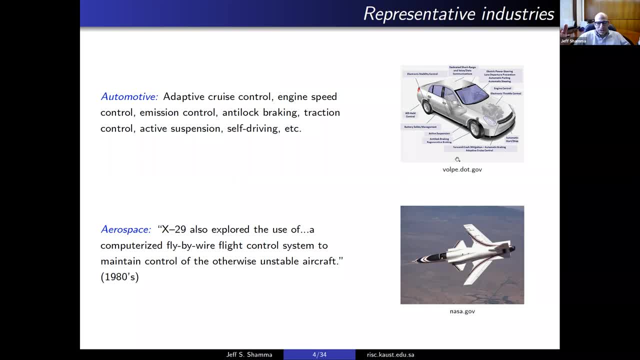 The idea was that by having forward swept wings, that induces an instability in the aircraft, but that instability would also bring in higher maneuverability. What was meant by fly-by-wire? fly-by-wire is something we take for granted now. It's that. 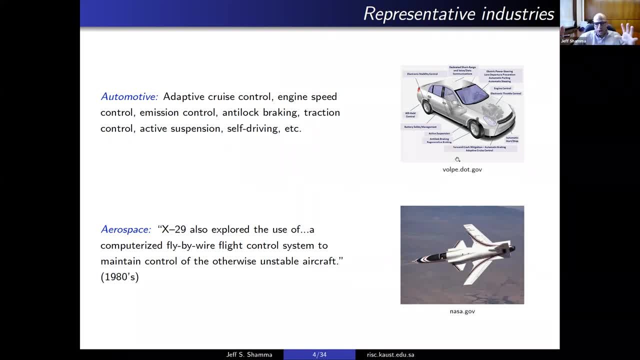 The pilot doesn't physically control the surfaces of the aircraft, but rather the pilot gives high-level commands to a computer which then controls the surfaces of the aircraft to do flight control, And that's hence the terminology fly-by-wire. Also a point to make here is that a human pilot cannot fly this aircraft. 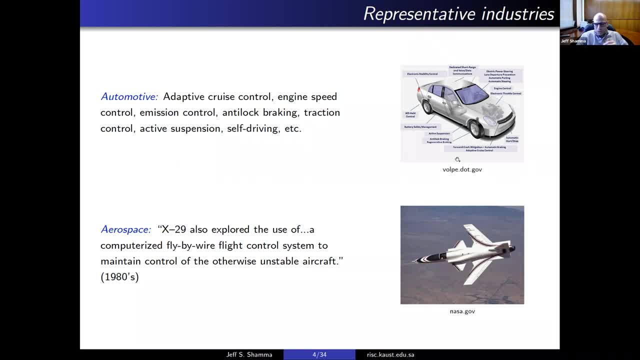 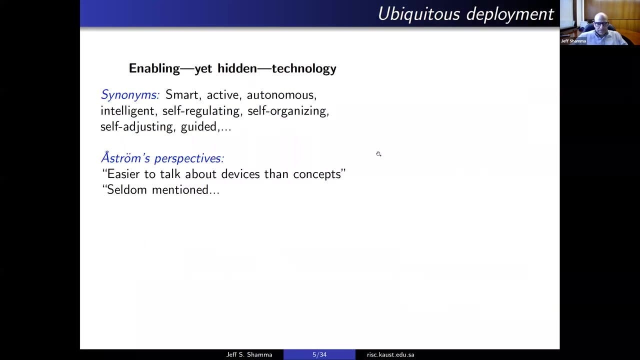 It had to at the time have been flown by a computer. So when we talk about superhuman performance, at least for this kind of flight control, Traditional controls approaches have had superhuman performance for decades. So I mentioned that. controls is everywhere and it's not talked about a lot. 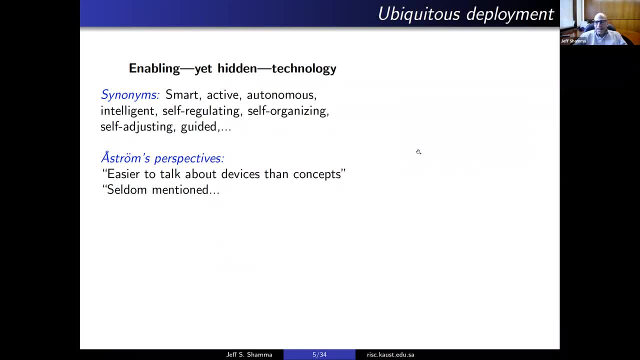 And so you'll find various synonyms, if you will, that indicate a feedback control loop, of sense decide and actuate is present. So, whether it's smart, active, autonomous, intelligent, self-guiding, self-regulating, self-adjusting, 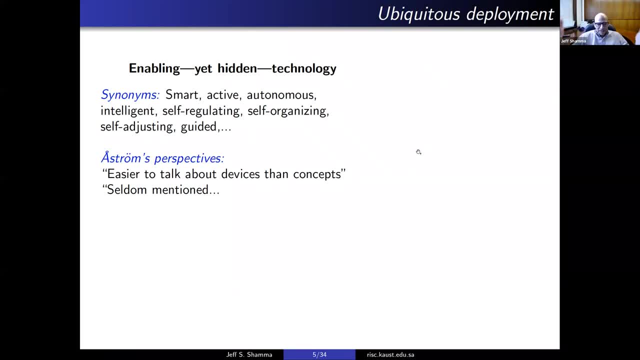 These are all ways that reflect that there is a feedback control loop that's active. And, referencing Astrum's lecture, he mentions that it's easier to talk about devices than concepts. So it could be that feedback control enabled a particular application, but it's easier to talk about the robot or the vehicle or the rocket than it is to talk about the enabling concepts behind what made that device work. 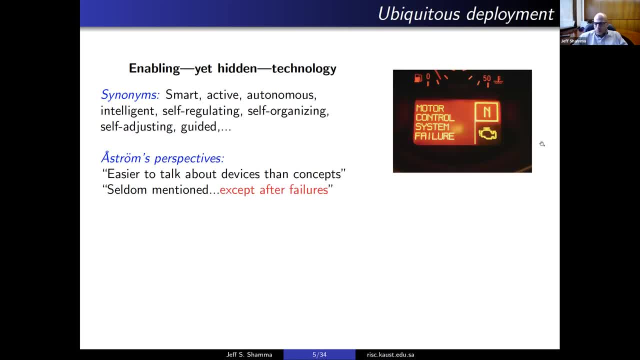 So feedback, So feedback control is seldom mentioned explicitly, except when there's a failure. And so now here is a screenshot of a dashboard of a commercial vehicle And it says motor control system failure. This might be the very first time the driver saw the words control system and it's next to the word failure. 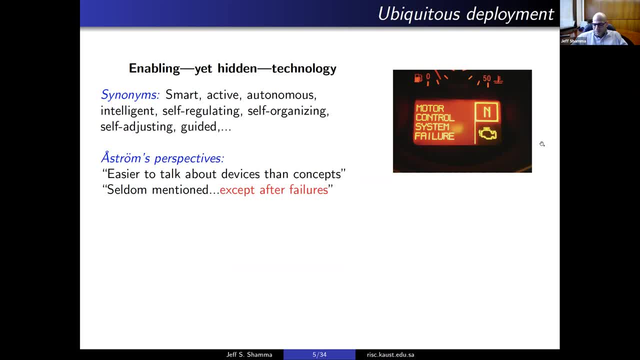 So when it was working, control systems weren't mentioned, And then when it fails, then now control systems take the headline, And so this is a lighthearted illustration, but actually for safety critical systems, When control systems fail, there's costly and tragic consequences of these failures. 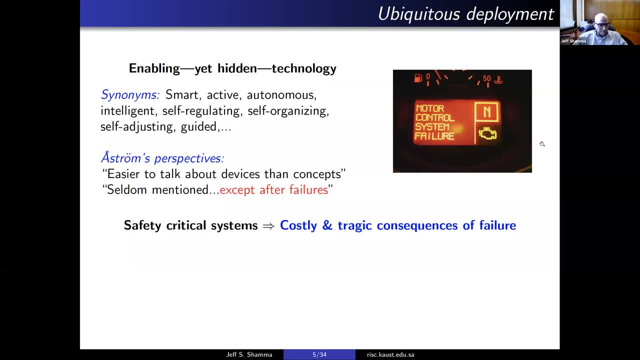 And you can do this about any time in the year. Earlier today, I just did a search, a web search, with the keywords control system and crash, And this is what came up. So here's one headline: the reason behind pilot deaths. 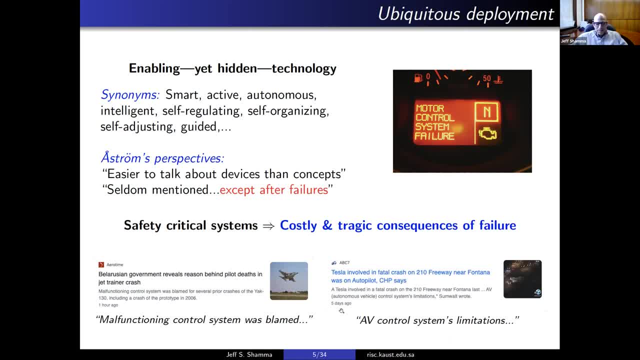 And it mentions malfunctioning control system was blamed. Here's something We're a lot regarding: test driving of a Tesla and the. it brings forward the the autonomous vehicle control systems limitations. here They weren't so much blaming the control system, but rather talking about testing outside of the capabilities of a control system, hence the control systems limitations. 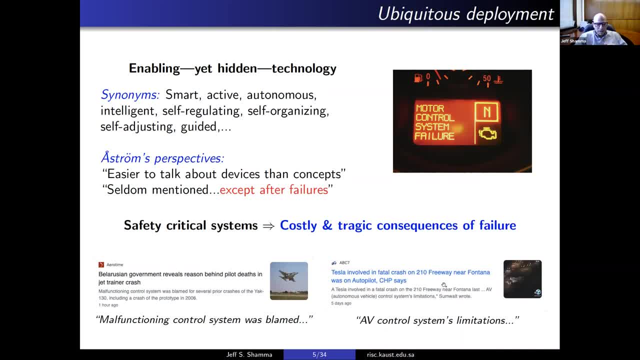 And that's something that we're actually we're going to talk about later on in the talk. but yeah, any time of the year, just put in the search control system and crash and you'll get some, some pointers into, uh, into what happens when control systems fail. 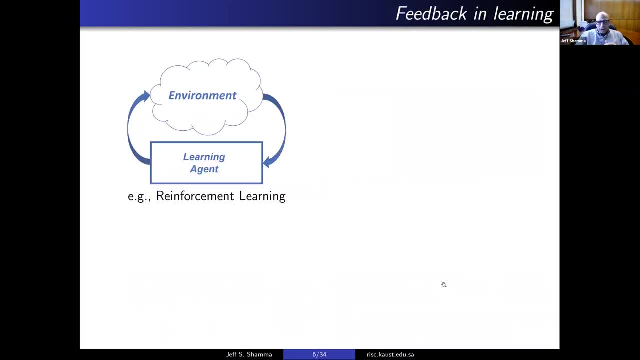 So that's feedback, control this loop of sense, decide and actuate. And now, what's the relationship to learning? Well, in reinforcement learning, you have a learning agent that's also interacting with an environment And the uh. through those interactions, the learning agents senses what's happening. 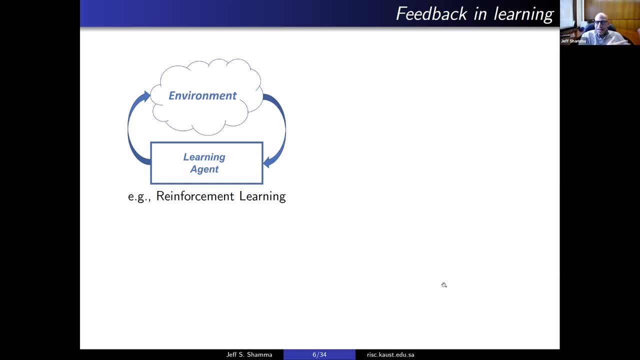 Does some uh adjustments to their decision process And then actuates. that actuate may be for the sake of performance, might be for the sake of- Okay, Of Experimentation, but the point is that there's a feedback loop present in in reinforcement learning, also in multi-agent learning. 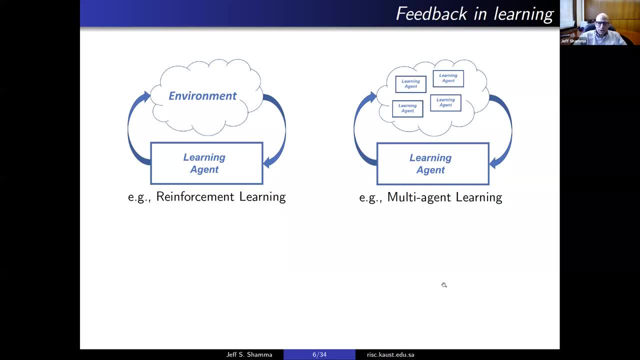 So multi-agent learning- and we'll talk about this mostly during the talk- is learning in the presence of other learners, So the environment is actually other learning agents. while I'm trying to figure you out, you're trying to figure me out, And that again creates a feedback loop. 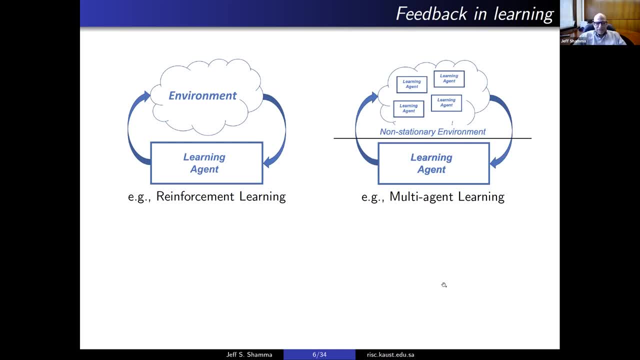 And one thing that makes it different from the picture on the left and say, in reinforcement Learning, is that the environment from the perspective of any single learning agent is actually a non-stationary environment. Uh, what do I mean by that? And the picture on the left? if I do an experiment yesterday and I do the same experiment today, then the outcome is going to be the same. 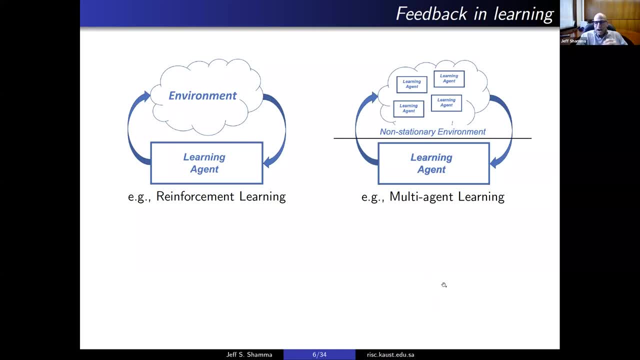 There might be some statistical variations, but it's the same environment And so I expect the same outcome, whereas on the picture on the right, if I do an experiment yesterday and do the same experiment today, the outcome might be different. Why not? 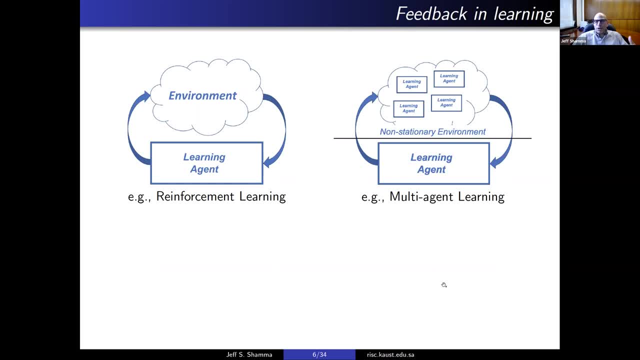 Because the experiment changed, but because The environment, the other learning agents have changed. they're in the process of learning and adjusting And so this uh taking it's. it's not so simple as taking a a single agent learning approach and popping it into a multi-agent learning scenario because of this feature of a non-stationary environments. 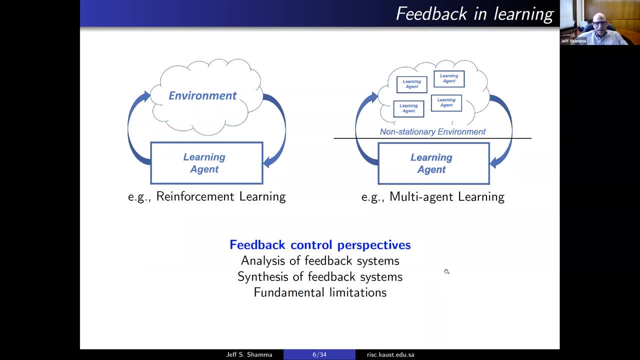 So what's the value, now that we see that we have feedback loops, the value of bringing in feedback control perspectives, that we can use some tools on analyzing feedback systems? Uh, we can use some concepts on how to design, synthesize feedback systems. 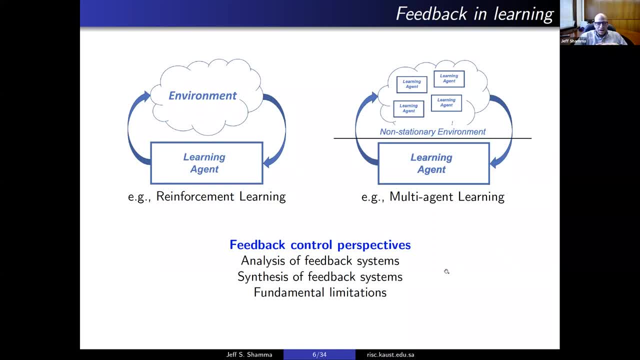 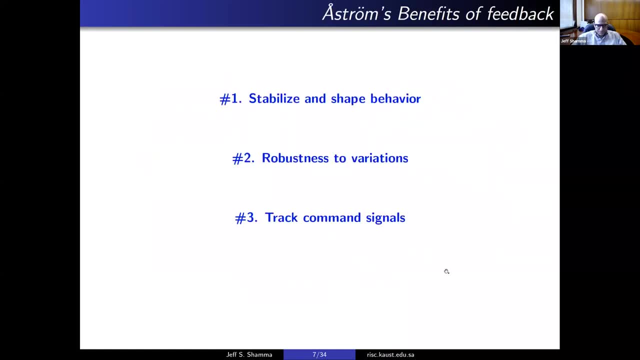 And then, as I mentioned, we also can understand not just what can be done but also what cannot be done, What are the limitations of feedback systems. And I hope to touch on all of these. And so, again, referencing uh Astrum's uh lecture on the benefits of feedback, he lists three benefits: uh stabilize and shape behavior, robustness to variations and tracking command signals. 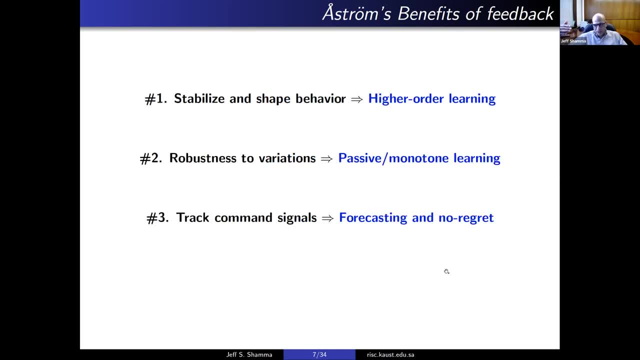 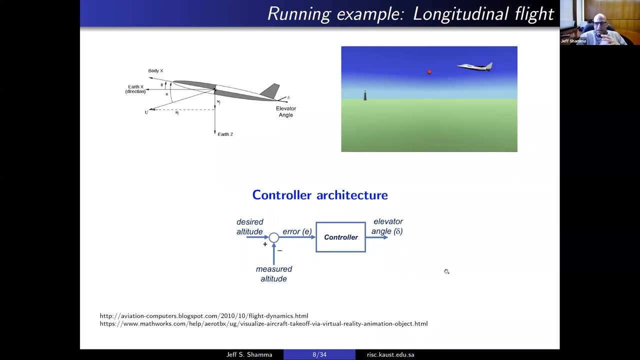 And we're going to translate- Translate these benefits to three learning scenarios. We're going to talk about something called higher order learning, passive and monotone learning and forecasting. and, and no regret, And we'll elaborate on these uh one by one and part of uh the discussion. we're going to use this running example: uh in terms of longitudinal flight. 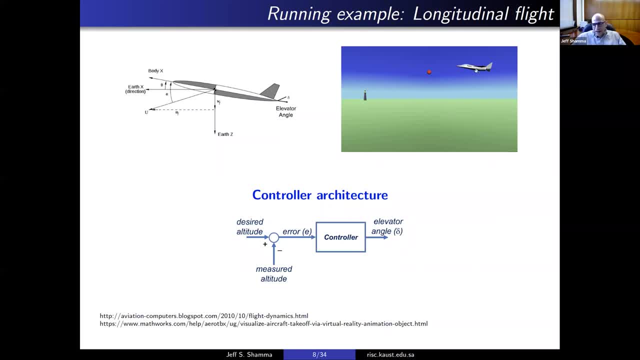 And so I'll first show the video. and the task of this uh aircraft is a simplified flight control example. It just needs to follow the bouncing ball, And so that is the Feedback loop. the ball's going up and down and the aircraft is moving its control surfaces, uh, so that it can follow the trajectory, uh altitude, of this uh ball. 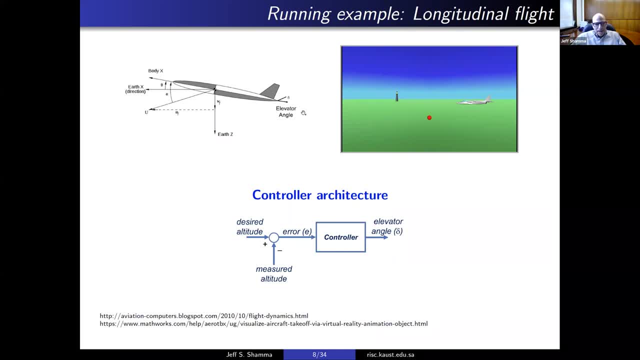 What are the control services that I just mentioned? The aircraft here in the back has what's called elevator angle. It is just going to move this surface, uh, up and down, and that will impact the trajectory of the aircraft, And we're looking at a very simple control architecture as well. 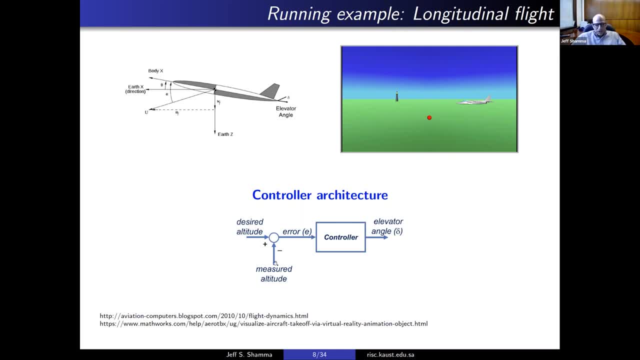 There's desired altitude, which is the bouncing ball, the measured altitude, which The actual altitude, uh, of the aircraft that produces an error, the controller. that's the sense. the controller decides what to do and then acts on the environment by changing this uh, this angle. 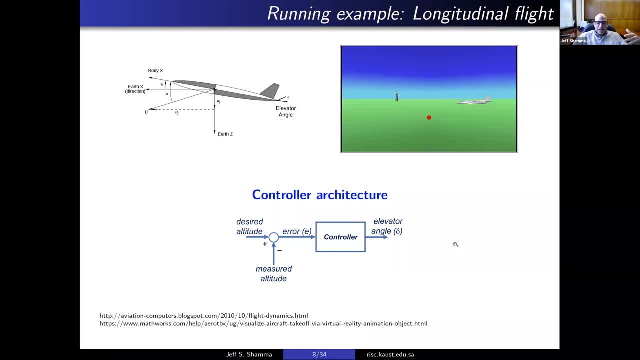 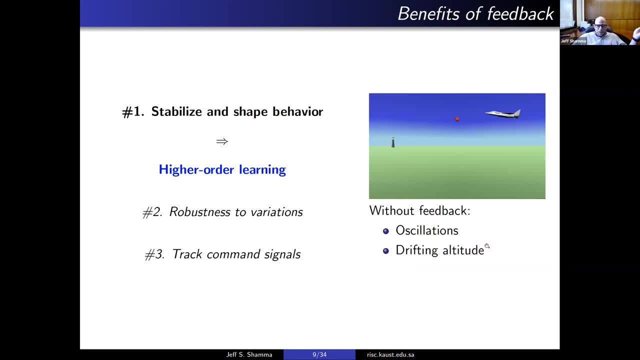 So we're going to use this example throughout to show the benefits of feedback and then how they apply to learning, And so the very first one is, uh, stabilize and shape behavior, And uh, so let me, let's show what happens if we don't. 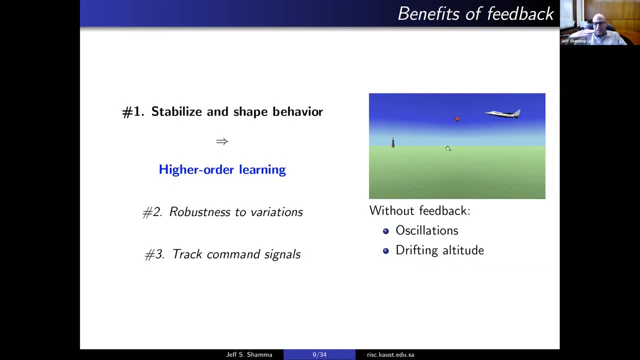 Use a controller to control altitude and just leave the elevator angle. fix this control surface in the back, the tail angle, uh, fixed. What we're going to see is that there's some oscillations and then eventually the aircraft drifts away. 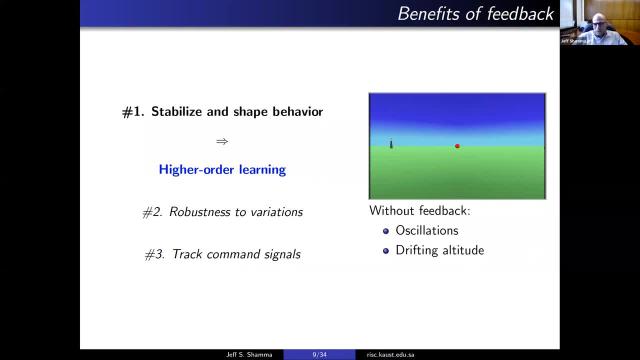 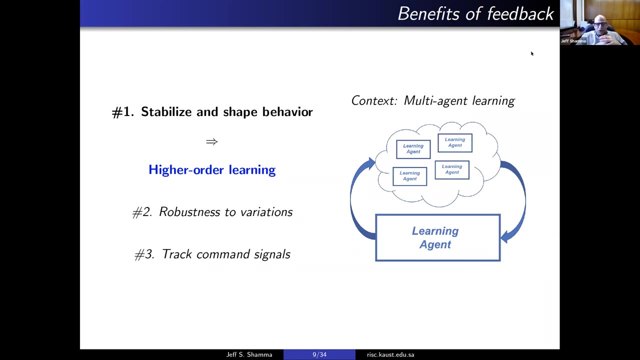 So without feedback, without actively measuring the altitude, it's doesn't stay at a level altitude by itself, Uh, and so we need uh feedback to be able to maintain altitude, And so that's going to lead us to talking about multi-agent learning. 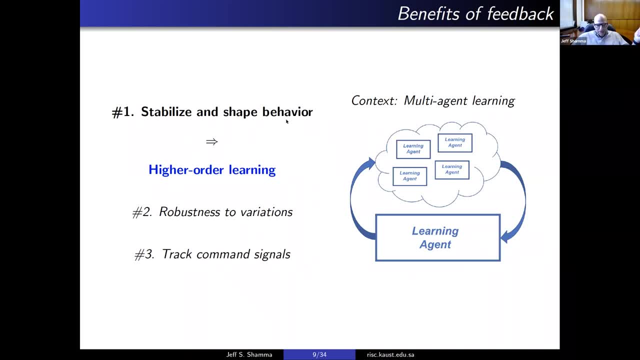 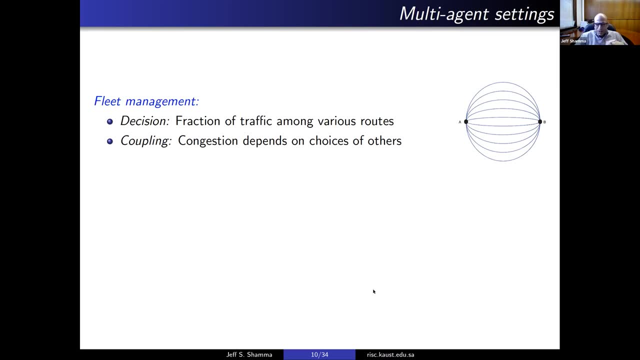 And uh, that will be the first context of of uh stabilizing and shape uh shaping behavior. So we haven't started yet. We're about to talk about these three settings. I can take a brief pause here. 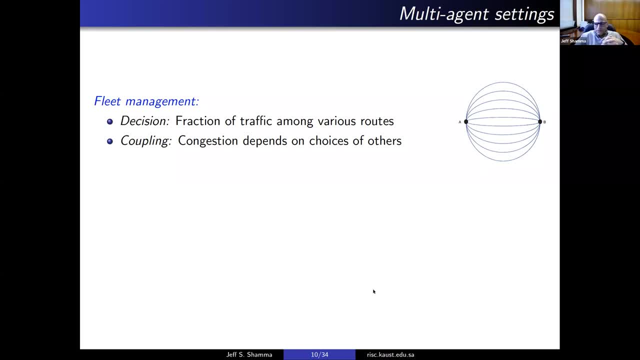 If there's any questions on feedback control before we migrate to uh, uh, feedback control, uh, perspectives on learning. So that's where we've just talked about feedback control. Uh, if you have any questions, please post them. on Q and a, let me ask a question, Jeff. maybe it's a clarification question for the audience. perhaps 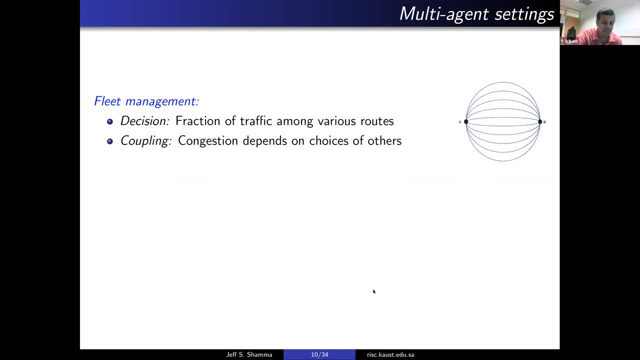 Uh, um. so if you think of multi-agent learning, if you think of the vector of all the control actions of all the agents- and I guess you could just think of it as a single agent learning- So I guess what you're saying here is that you're interested in situations where each agent is making its decision based on some local information. 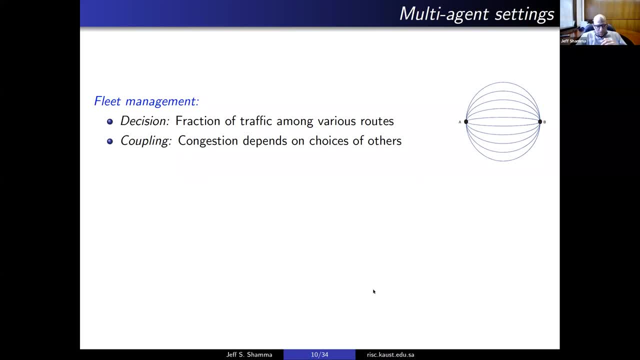 Is that why it's different? So maybe it will highlight that what makes multi-agent learning in particular different, uh, from single agent learning? but but you're right in that you know it's. it's based on local information. 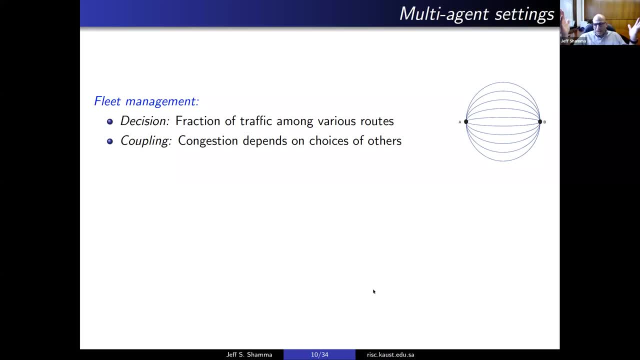 If somehow this information got disseminated to everyone, then it would look like a centralized uh uh uh setting. but also there's authority, uh, that we cannot dictate, uh, what the agents will do in terms of their learning algorithms as well. 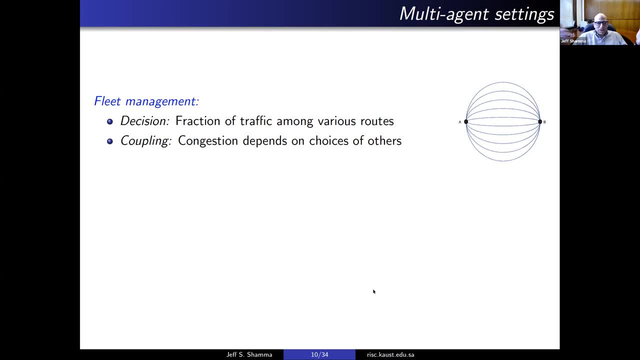 If it was centralized, then you can share information And then you can specify how the different agents will update and uh. but now each agent is independent on how we can update its uh or do its learning at its own pace, its own style. 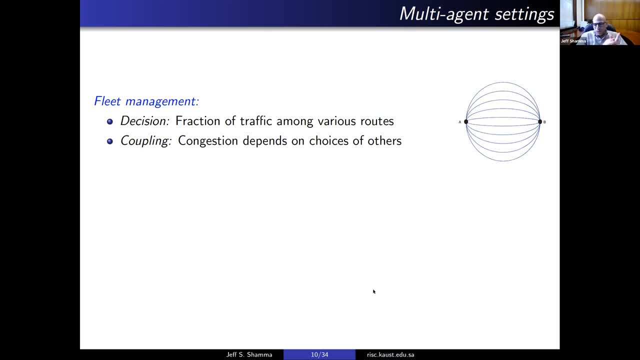 So that's another distinction. Even if this information was shared, we don't have the authority to tell the agents what to do and how to learn. Okay, Thanks, And there's a question in the Q and a. any thoughts? I guess two questions. 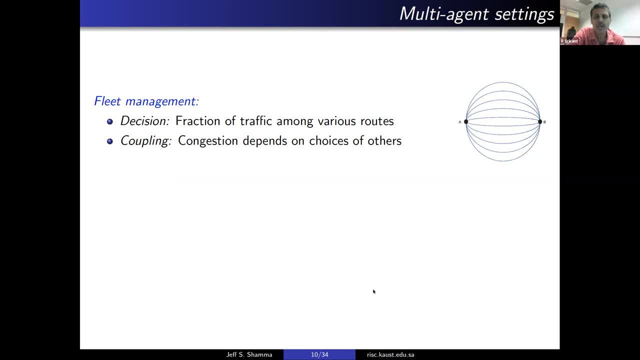 Uh, the first one's from Daryl Farber. Any thoughts about why concepts are less discussed than devices? I guess that's Uh referring to Carla's from school. I'll just speaking for myself. That's not as cool, Okay. 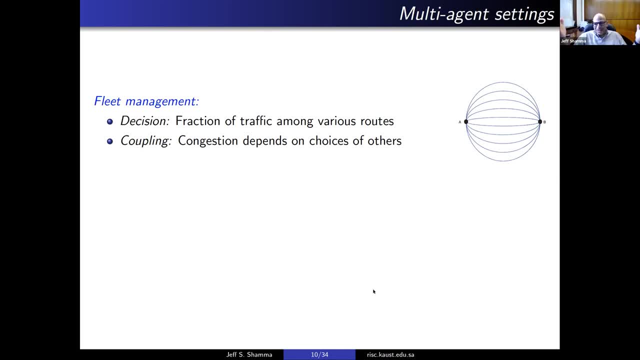 If it doesn't have the same broad appeal. uh, you know we how many videos, you know how many times we watched the video of the Boston dynamics robot doing a flip. But you know we didn't really talk about. you know what. you know all of the things, not just feedback control, but all of the things that went into that, it's, it's, that's that gets the headlines. uh, as I said, until it, until it fails. 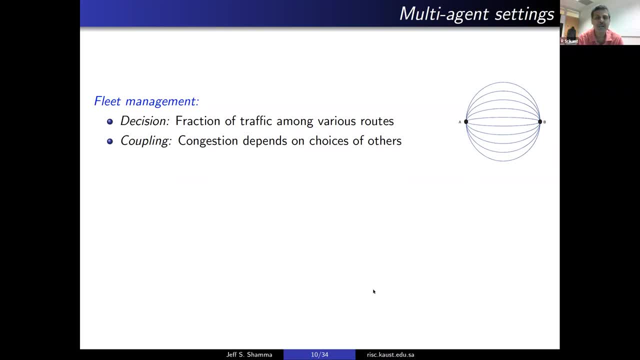 And uh, the second question is by William Sullivan: uh, in your model, can humans be agents or are they just control systems or a few months? So actually we're going to uh, I think it's important that they are uh humans and that. and back to uh Shrikant's comment: is that okay? even if we shared uh information, we cannot dictate how the agents will learn. 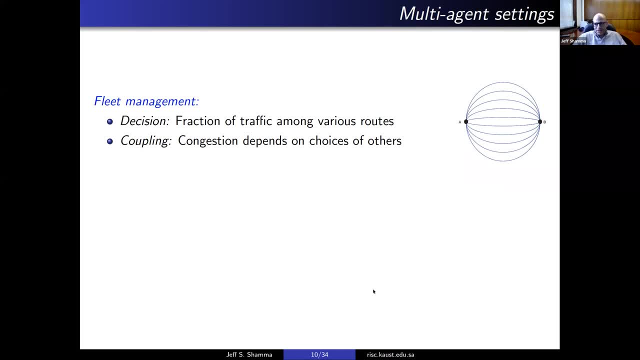 If these were programmable devices, then we could dictate how the agents will learn and try to program. For example. uh, if this was a multi-robot system, uh, setting aside the issue of information, we can program them to learn in a certain way so that we can evoke a desired effect. 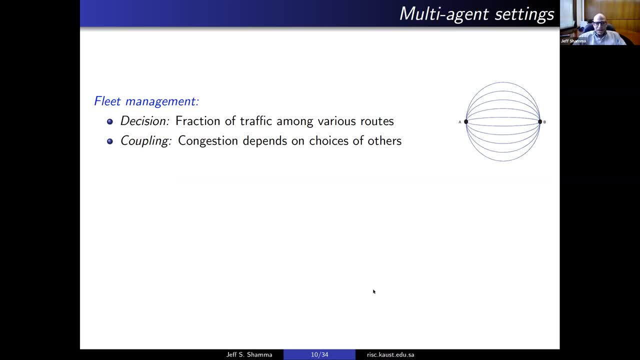 And that's, that's another field of of say, uh, a multi-agent learning where they're programmable devices. but we're going to take a lot of uh. what we talk about is actually motivated, uh, by game theory, where the intent is to model human decision-making, where we cannot dictate how the learning happens. 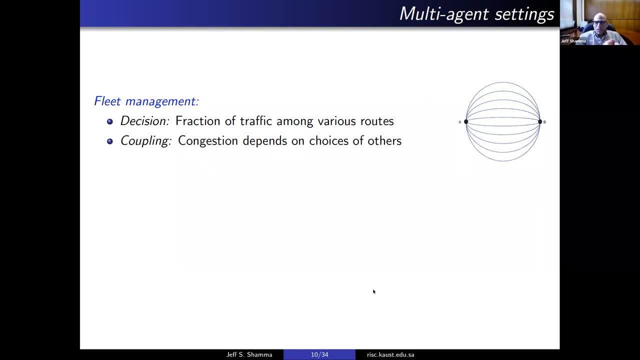 And one thing that we'll get to uh in a couple of slides: uh reflects that it's more of a a model of humans rather than uh engineered devices. Okay, So the next question is from Tim Doan. 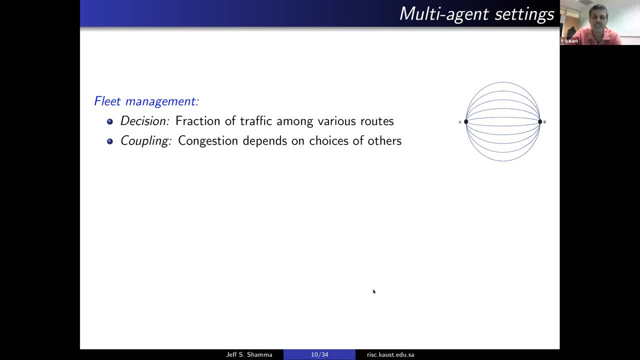 Uh, can you elaborate more on the non-stationary environment and multi-agent systems? I guess he wants to know why it is non-stationary. Okay, Let me get to this, uh, through this set of examples and and then come back to that question. 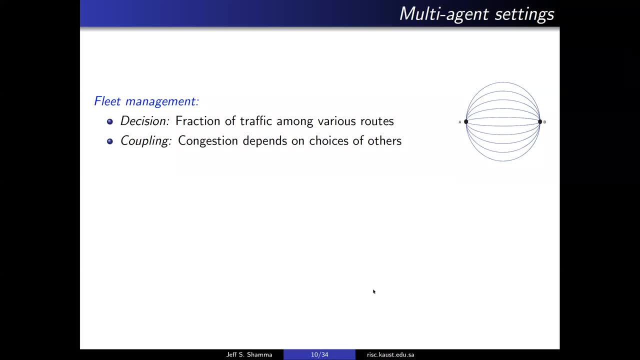 Okay, Great, Thank you, Okay. So what's a multi-agent setting? So here's a simple, uh a setting of, say, fleet management. you operate a hundred vehicles, There's a handful of routes and you need to determine how many vehicles go on each route. 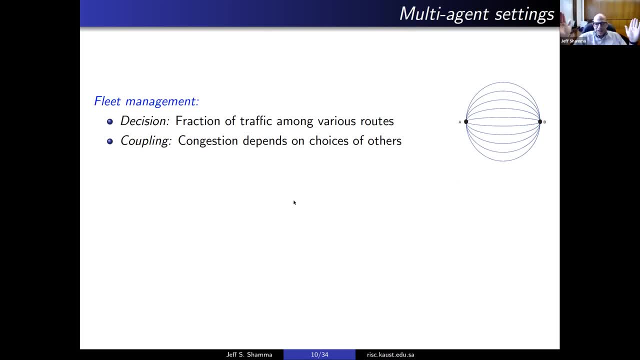 every day to get them from A to B. That's your only task. Get your vehicles from A to B with minimum congestion. The issue is that the congestion that your vehicles experience uh are a function of the uh, the decisions, the choices of other users of those routes. 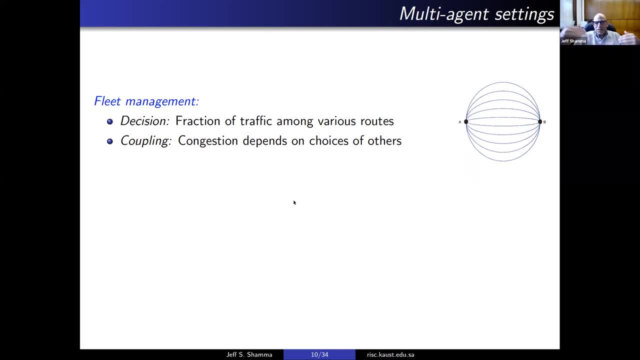 And so, uh, you have a coupling in these decisions. If there's another fleet manager, then they're also going to be deploying their, their vehicles, on these routes, and the congestion that you experience depends on the routes you've selected and also the routes that, uh, others have selected. 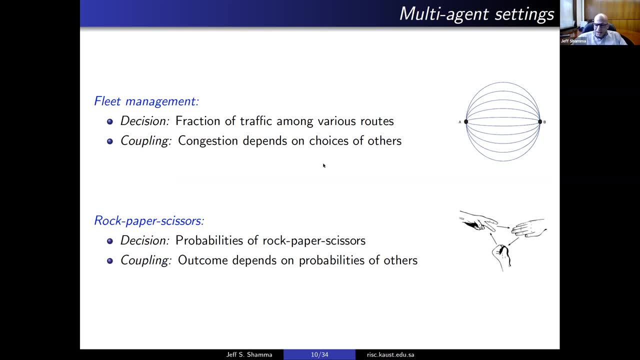 So that is a multi-agent setting. Another one is a common one, that, uh, that we may be familiar with, and that kind of captures. although it's very, very simple, it captures a lot of what we're talking about. Uh, so in rock paper scissors- let's say that you don't decide rock paper scissors- 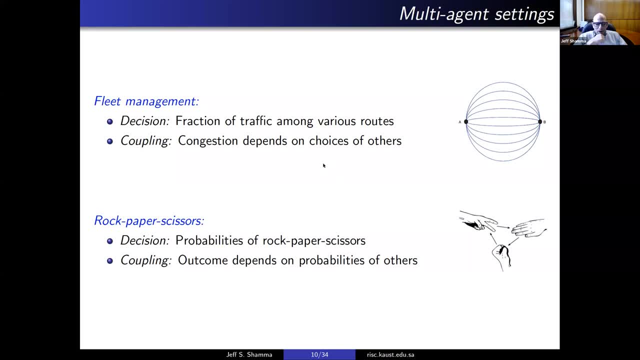 but rather you decide With what probability you're going to play rock paper or scissors, but the outcome depends on the probability of your opponent, And so you pick your probability, they pick their probabilities, And so the outcome doesn't depend just as a function of your own decision, but as a 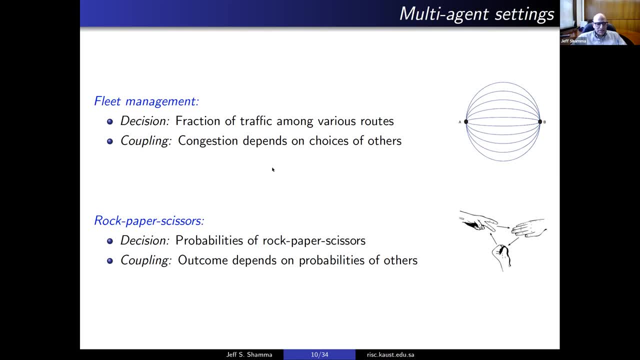 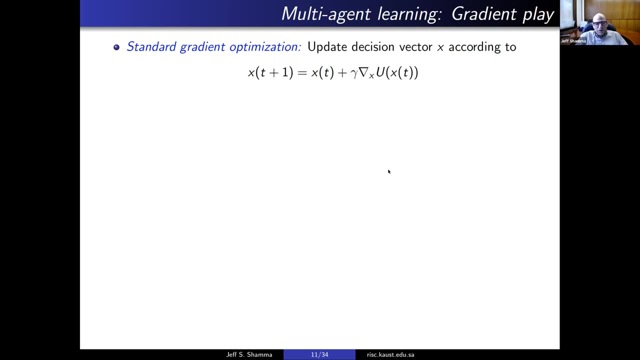 function of the decisions of others. These are multi-agent settings. And so now, what does multi-agent learning look like? Uh well, let's look at single agent learning first, And here I have a representation of gradient descent, uh, where I have a decision that 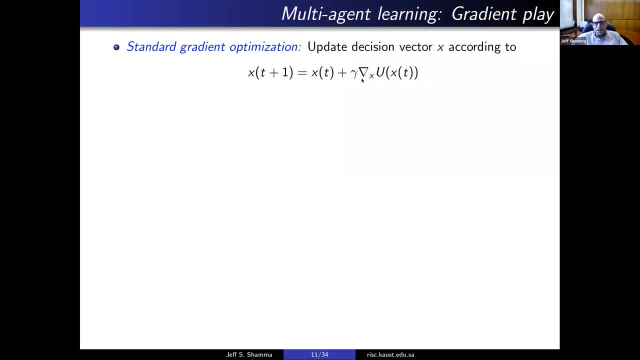 I'm going to use for my decision vector And my new decision vector is my old decision vector plus some upward hill climbing. That's depends on how I score my decision- my own utility function. So in standard gradient optimization I just try to move uphill. 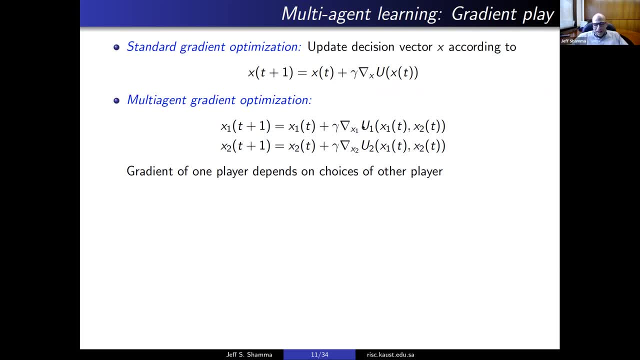 And now here's the non-stationary environment. My gradient is not just the function of my own decision, but also the decisions of others, And the decisions of others is also being updated according to a gradients- uh hill climbing rule of someone else. 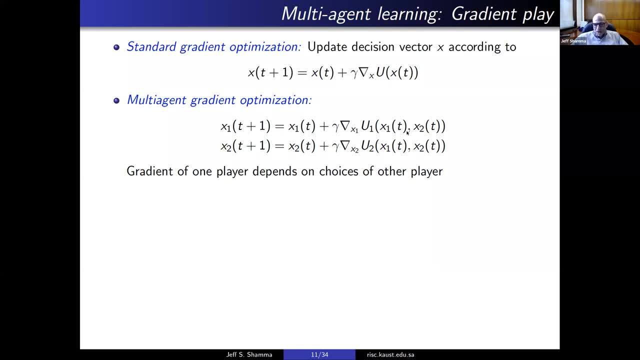 And so now the gradient of one player depends on their own decision, but it also depends on decision of someone else, And the decision of someone else is evolving on its own, according to its own needs. And so from the perspective, you can compare these two from the perspective of any single. 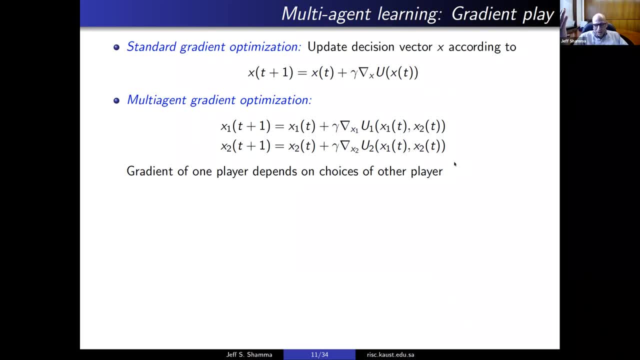 agent their gradients. even if you don't change your decision vector, your gradient is changing. Why? Because someone else is changing, And so you can kind of visualize this in terms of a, a, uh. you know, I typically picture for gradient descent here. 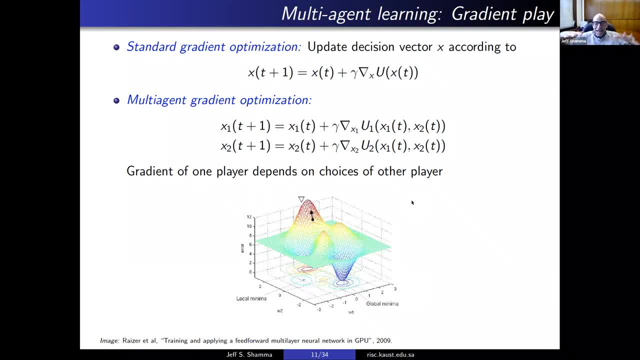 I want to walk uphill in this environment, but the landscape is changing. Why is the landscape changing? And is because this landscape depends on the decisions of others, And and so now, what used to be uphill might not be as uphill anymore, or it actually might. 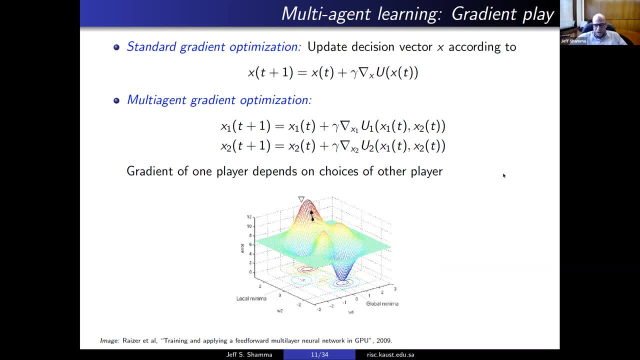 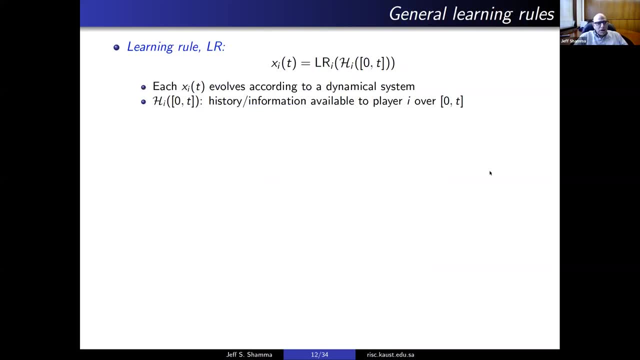 be downhill because others have changed and that's the non-stationarity. So a learning role. I showed a gradient updating but a learning rule. pretty much, we're going to have this, uh, this very generic uh, representation of learning. 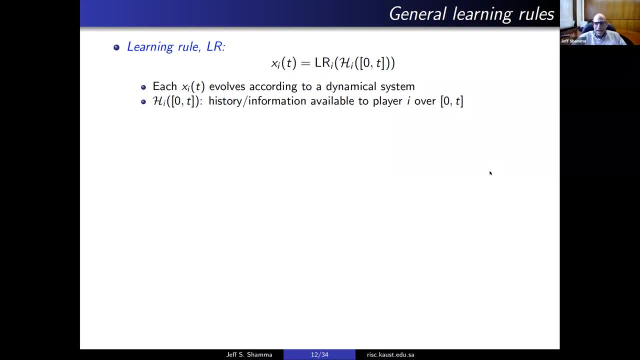 My decision vector is updated according to the information that I have from the time we started. Okay, That's a placeholder for a general, a learning rule, And then we want to ask questions such as: how does a learning rule behave with different environments? 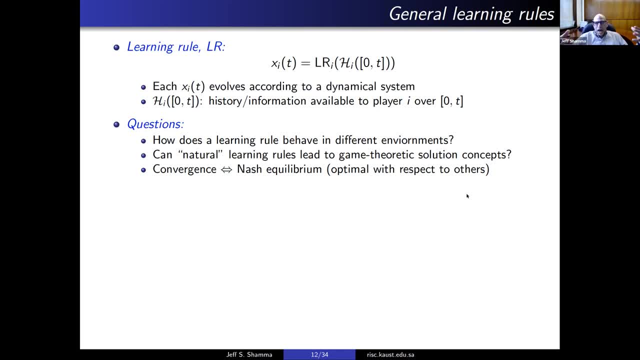 What learning rules are natural and and how do natural learning rules uh result in various solution concepts. one solution concept that you've may Come across is that of Nash equilibrium. When would we stop learning is when we're all satisfied with our decision. 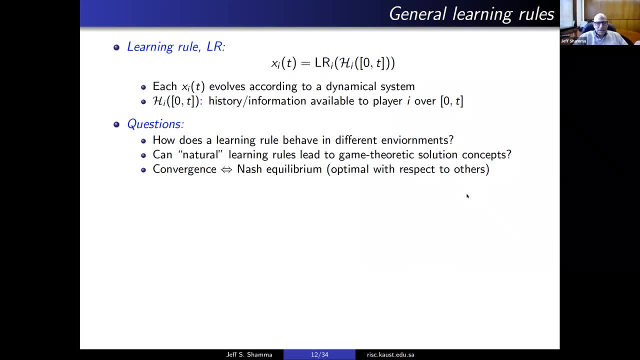 And that's what a Nash equilibrium is: that my decision, given my decision, given the decision of others, is what I would like to do. It's optimal with respect to the decisions of others. So these learning rules will eventually converge when they reach a Nash equilibrium. 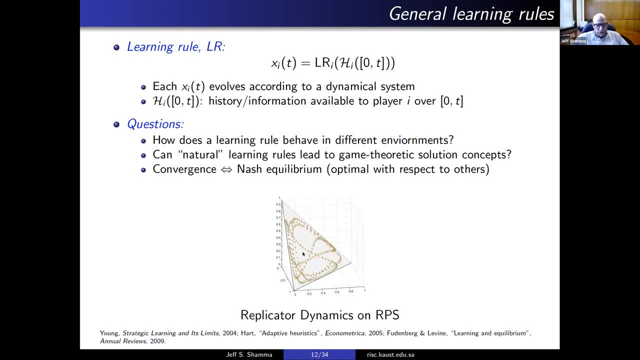 And we'd like to know when that happens or when it doesn't happen. And so here's a illustration of something very similar to reinforcement learning. It's It's called replicator dynamics, And what we have here is replicator dynamics, which is like reinforcement learning on rock. 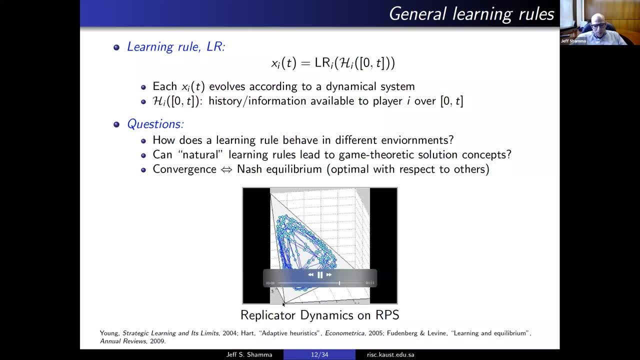 paper, scissors. This picture is showing the probability of rock, probability of papers, probability of scissors. Uh and, and one agent is using replicator dynamics or reinforcement learning to learn whether they should play rock, paper or scissors. But the issue is that the other player is also using reinforcement learning to play rock. 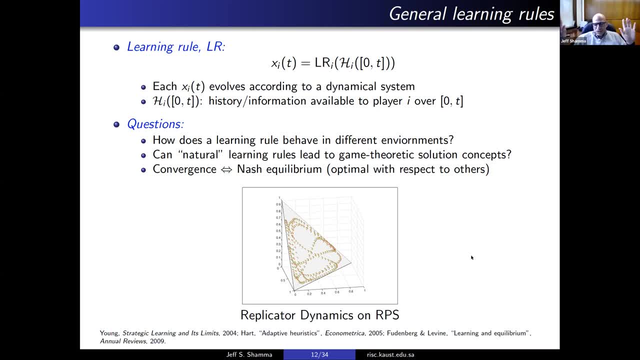 paper or scissors. If one of them was Fixed with a strategy, a decision, then one agent would learn how to optimally play. Well, when you put these two together, they end up chasing each other And in fact it can, uh, exhibit the chaotic behavior. 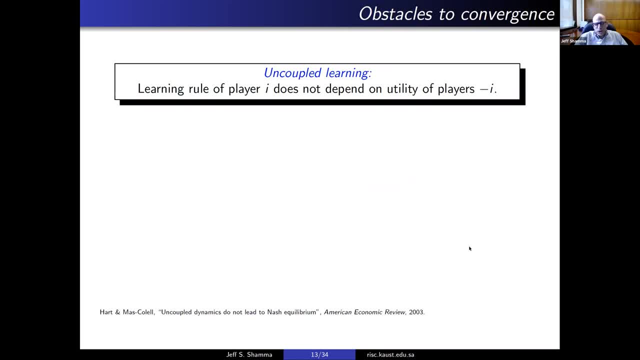 So now we're, we're coming to the concept of, say, modeling humans as decision makers, And one notion of learning- uh, that's natural, if you will- is what's been called uncoupled learning, And so an uncoupled learning. 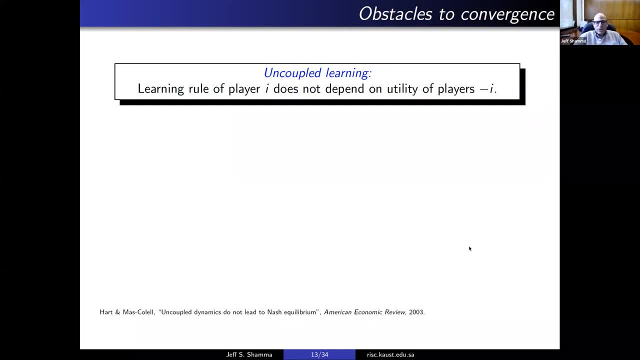 I can react To what you do, but I can't react to why you do it. You have some incentives. You have a reward function. I don't know what your reward function is If these were programmable robots, programmable devices. we can inform each device what the 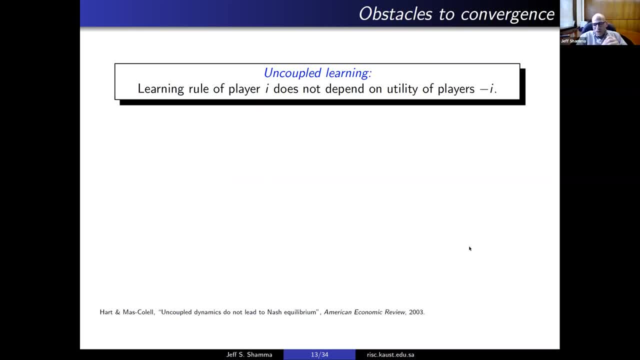 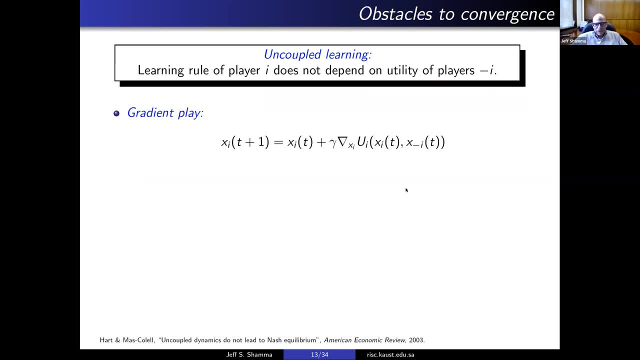 reward function is of the other devices, But if it's a human with another human, then I don't know what your your, why you do what you do, but I can observe what you do. So this is called uncoupled learning. 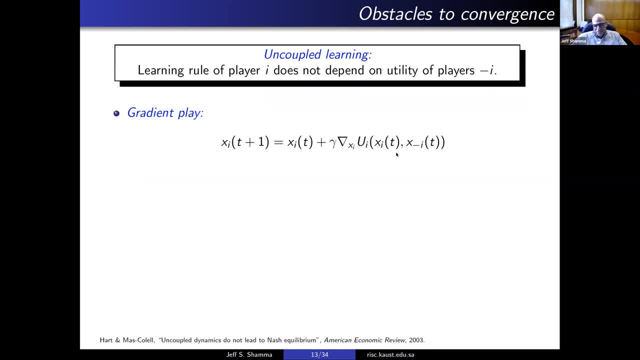 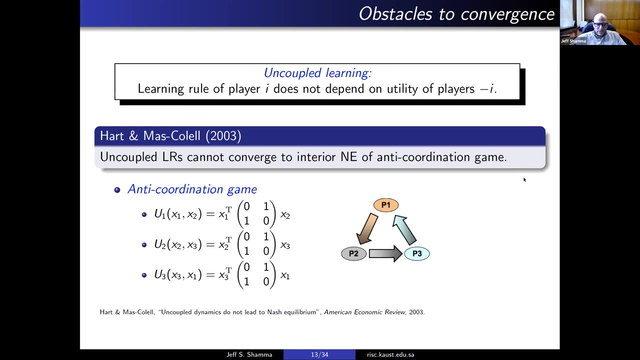 And we saw that this one example of gradient updates is Uncoupled. agents uses their own utility function while observing what others are doing. But an agent never uses in their update rule the utility function explicitly of what other agents are doing. And a paper came out a couple of decades ago that said that if you have an uncoupled learning 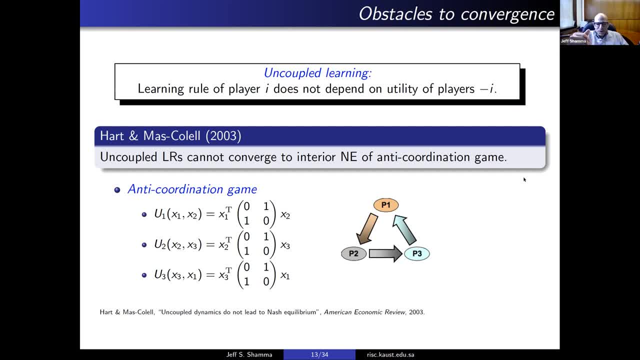 rule, then you cannot converge. These dynamics will never converge. in particular, They won't converge to a Nash equilibrium. And they used one environment, one game, uh, to illustrate that. So we have three players. player one wants to be different from player two, player two wants to be different from player three. player three wants to be different from player one, and they're just picking left, right, or actually more, uh, more precisely the probability of left and right. 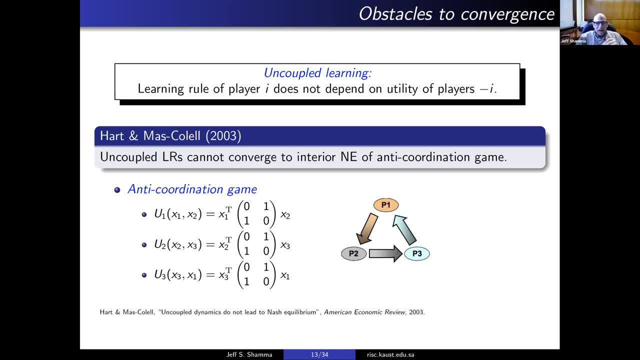 This does have a Nash equilibrium, but they showed that uncoupled learning rules which have this natural interpretation. I can see what you do, but I don't know why you do it. Uh, they will never converge to Nash equilibrium for this three player game. 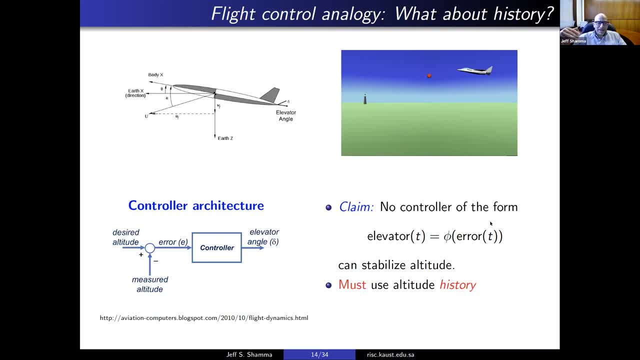 So now let's bring in uh, a, uh, a feedback control concept and it's going to be, uh, stabilizing and shaping behaviors. So again I'm going to show the aircraft following the bouncing ball. Remember this uh, tail angle reacts in, in, to the error in altitude, but actually it reacts into the error and altitude in a, in a uh, particularly kind of a little more sophisticated way than a naive way. 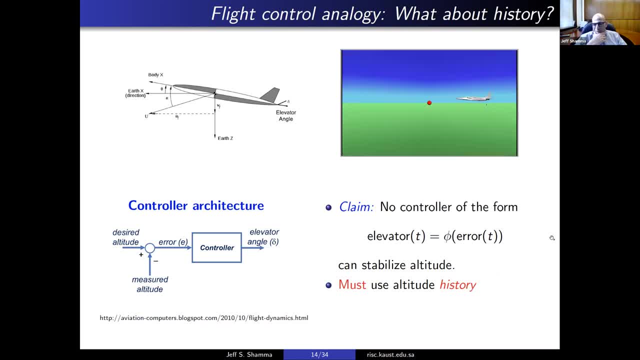 What if the angle was a function of Only the current error? So what's happening here is the angle is a function of the current error and it's unable to hold altitude. The way it's able to hold altitude before was that the angle was not just a function of the current error. 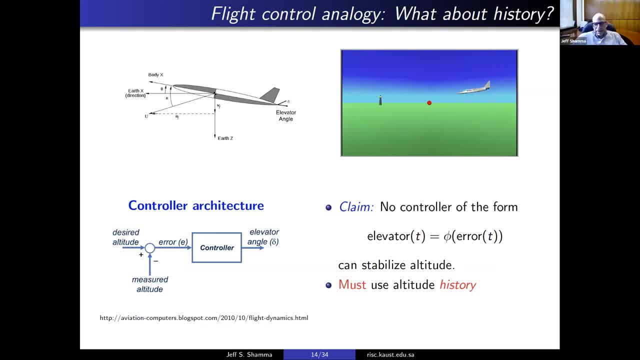 It's a function of the history of the error. Okay, And but if you have the angle of function of the current error, then you can show that it will never be able to hold altitude. You have to use history to be able to hold altitude. 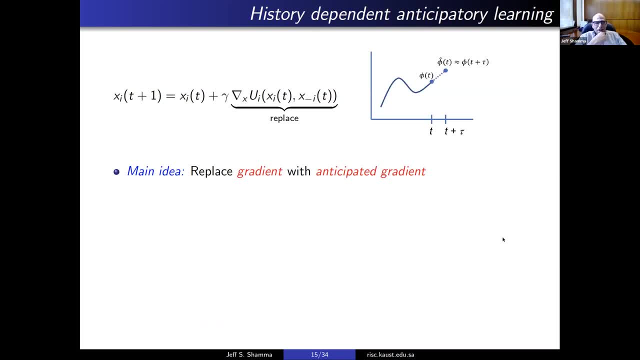 So what we're going to do is we're going to- We're going to use history in a very simple uh way. we're going to replace the gradients with an anticipated gradients. and how do we do this anticipation? Uh, this is just an illustration of the gradient. is has a recent trends. 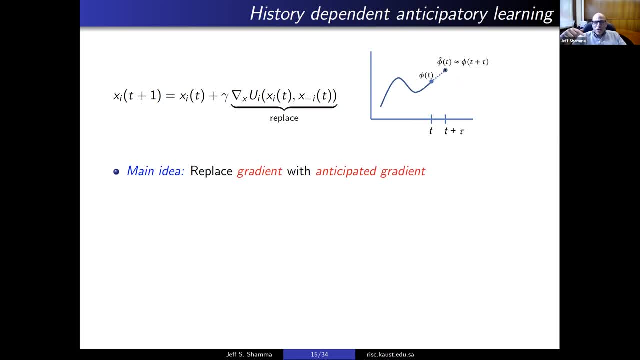 I'm going to do a bit of an extrapolation and not move my gradients and function. uh, not use my current gradient, but use the gradient where the gradient is trending. Okay, So we're going to replace the gradients with the trending gradients. 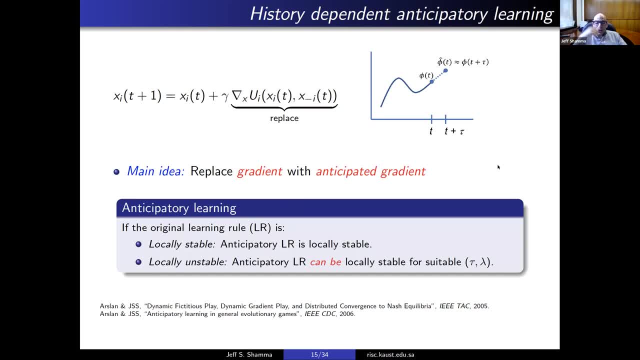 And in fact, This will uh enable convergence. So you see, it's still uncoupled. I'm not getting any extra information, I'm just using the information that I have in a uh slightly more sophisticated way, And so when uh learning is unstable, the anticipatory learning can be stable. 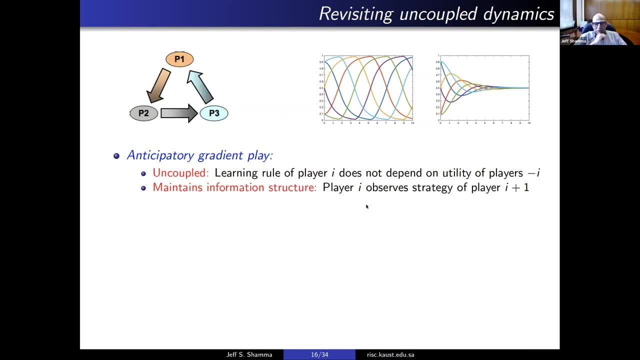 And in fact it is stable for this game. uh, where it was concluded that uncoupled- look on, coupling is uh, or uncoupled dynamics- was an obstacle to converging to Nash equilibrium. Actually, It's Not the uncoupling, it's because it was using its information in a uncoupled naive learning. 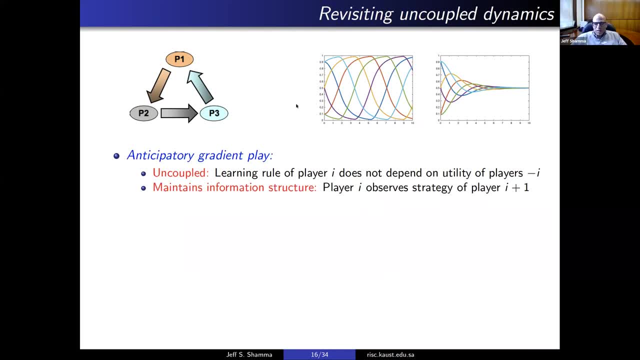 But if you allow the use of memory, then you can get convergence to Nash equilibrium, even in this counter example game. And there are other examples of, say, with replicator dynamics- I'm not really talking about replicator dynamics today- where you can turn chaos, the chaos picture that I showed you before. that chaos picture turns into convergence. 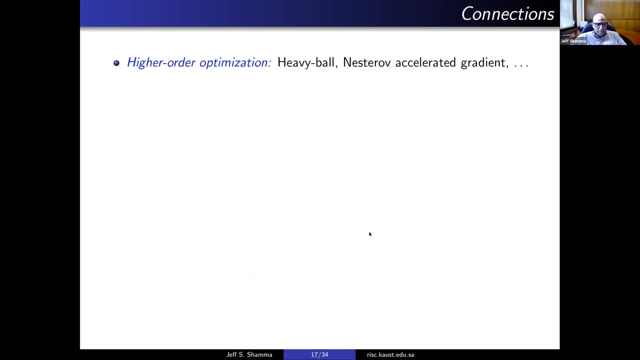 When you do anticipatory replicator dynamics, uh, whatever that. I'm not really talking about replicator dynamics today, where you can turn chaos, the chaos picture that I showed you before- that chaos picture turns into convergence. When you do anticipatory replicator dynamics, uh, whatever that. 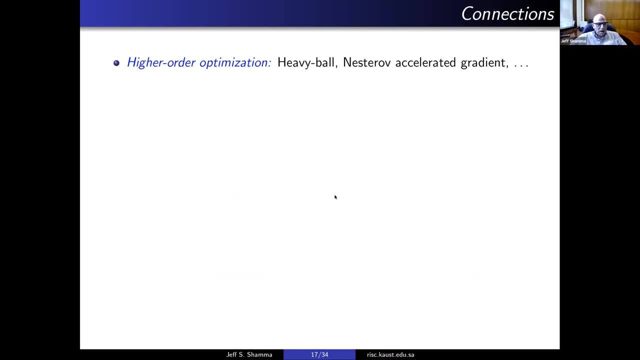 I'm not really talking about replicator dynamics, uh, whatever that, There are some connections to some ideas going on in uh in uh optimization these days. Uh, there's always been a kind of an interest in higher order methods using memory. 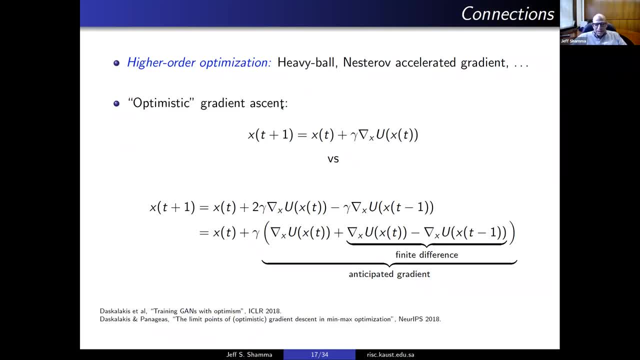 And in particular, there's something that's called optimistic gradient descent. Uh, this is a lot to take in in, in, in in a flash. but pretty much what optimistic gradient descent does is it takes the current gradient and uses a difference in gradients to create an anticipated gradient. 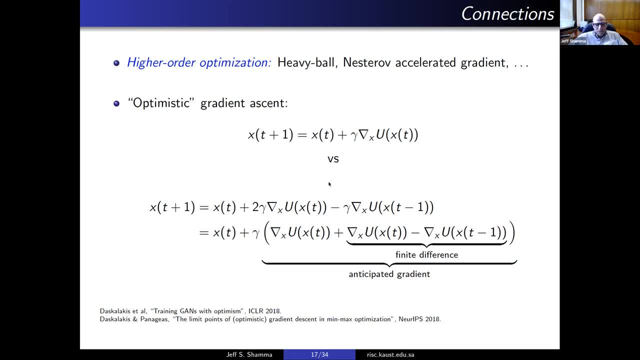 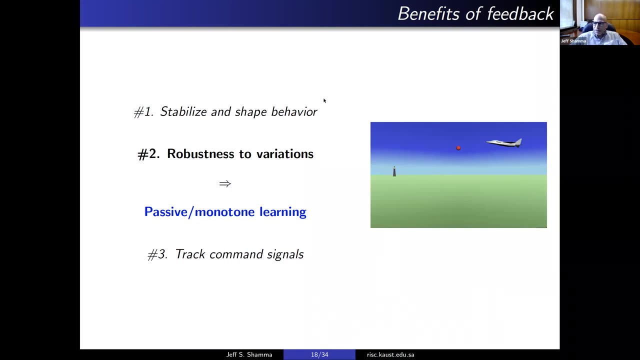 And so this idea Is indeed built into optimistic gradient descent, which is getting some uh new attention in min max learning. uh for uh for neural nets. Okay, So that's a natural breaking point. We talked about stabilizing and shaping behavior and we can take any questions here. 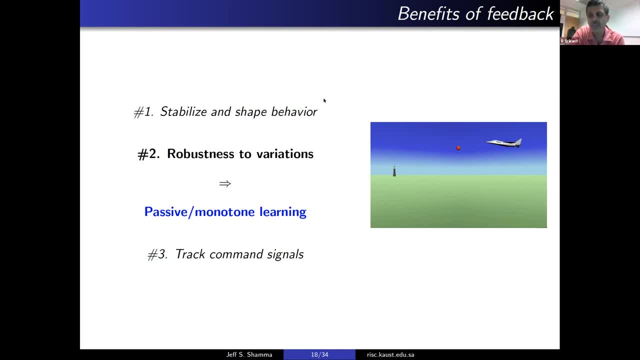 I think you already answered the question about the non-stationary environment when you're talking about gradient descent. Uh, so the next question, Okay, I can interpret: Can AI ML applications be used for the multi-agent learning system? I guess maybe. uh, the question- let me re rephrase it based on how I interpret the question, or or you can interpret it any way you want, but I guess, uh, beyond just gradient descent, are there other AI ML applications? uh, sort of naturally. 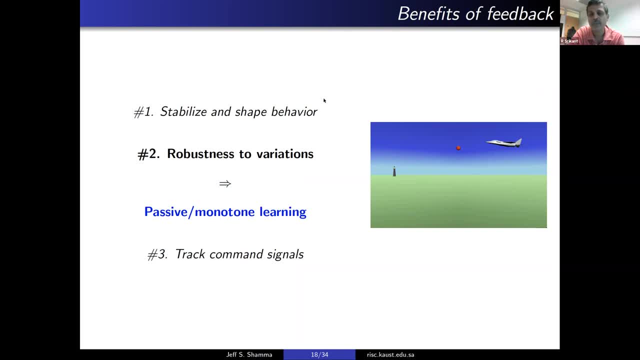 Uh, blend into multi-agent learning systems. I mean, for example, sensing could use neural networks. There could be other aspects of AI that are used not just in the gradient descent part, but maybe for the sensing part and so on. How does it work when all of them are integrated into a multi-agent learning system? 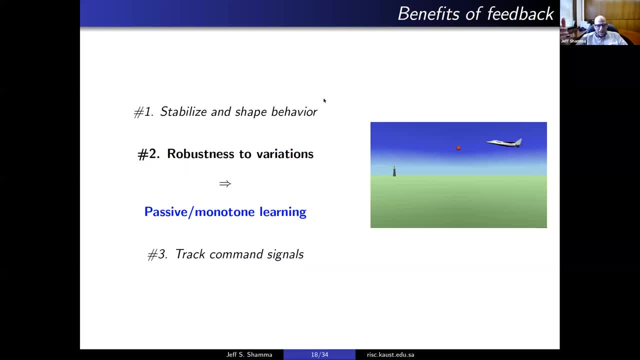 So there's one immediate connection is using two-agent learning for training neural nets, like in adversarial networks, And so that's kind of an offline training scenario. There can be now online scenarios where, say, you program a set of robots to do things like perimeter defense or to do a sensor- if you had mobile sensors- where the sensors should locate themselves? 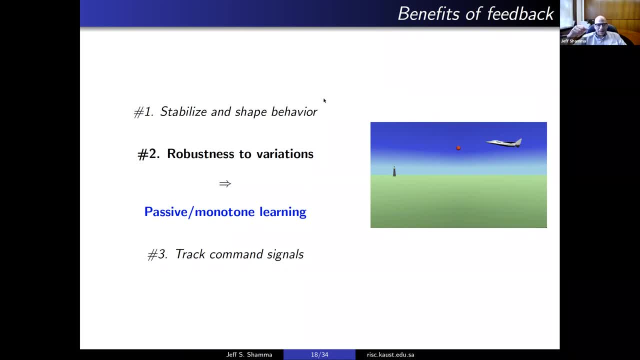 And sensor placement has that coupling. It has that effect that the value of putting a sensor at a particular location depends on where the other sensors are. And you can think about, say, deploying AI, You can think about deploying aerial vehicles to complement wireless coverage. 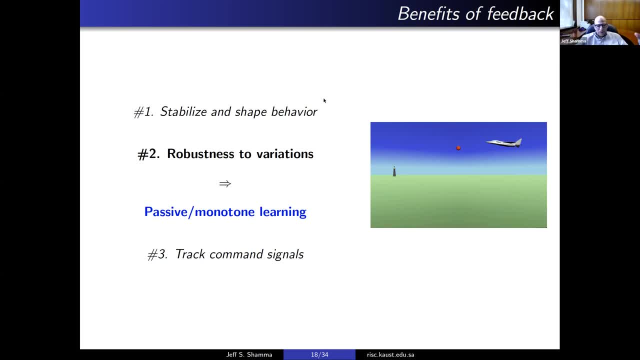 And so again, putting a drone to help, complement or support wireless coverage. its value depends on where you place it, And also, where you place it is going to cause interference with other communications as well. And why do this? in a learning approach? 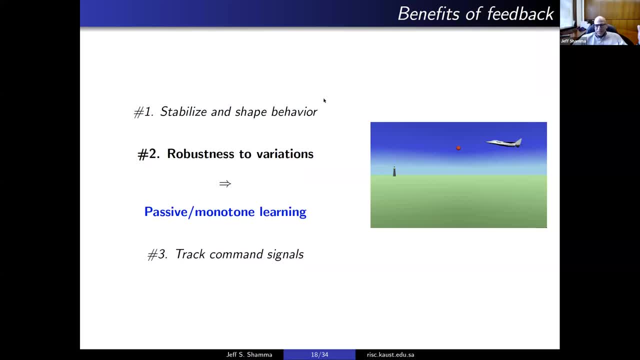 Because we don't know the environment beforehand. And so one approach would be to go out, figure out the environment Report, Report it to a centralized node, Compute an optimal deployment and then send things out. Or you say, just let them figure it out through a combination of exploration and exploitation. 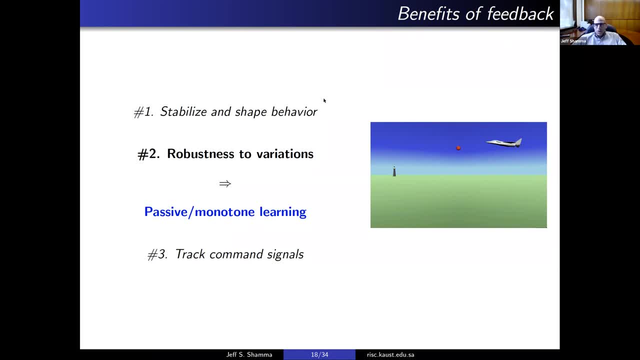 Figure out where to go based on the environment that's there without doing reconnaissance first and then deployment. So I'm showing gradient descent, but the really gradient descent is a placeholder. Let's take the key issue here was uncoupledness. Put as sophisticated of an algorithm that you want. 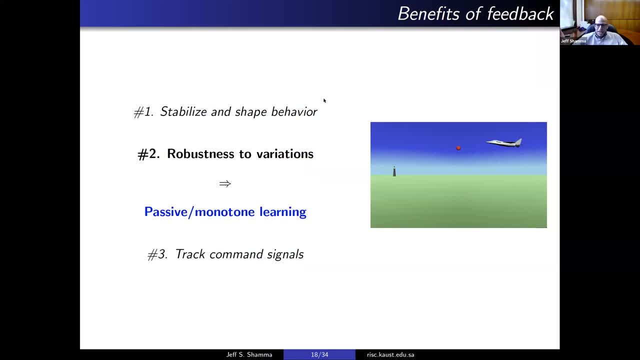 It's either going to be coupled or uncoupled. Either the learning neural nets or the simple gradient knows or doesn't know the incentives of other agents. Great, Thank you. So I guess I noticed somebody raised their hands. We can't call upon people. 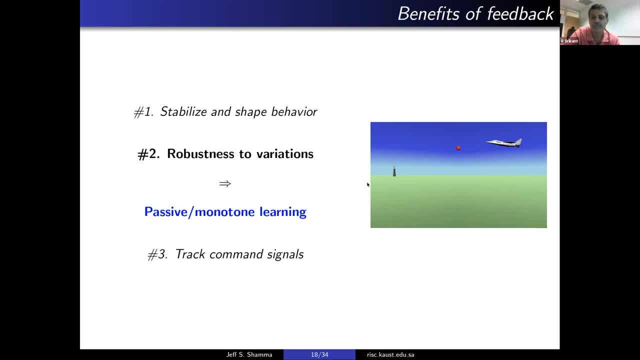 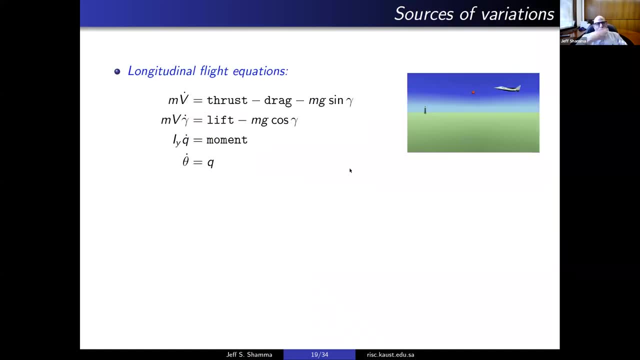 So if you have a question, please put them in the Q&A. Thank you, Please go ahead, Jeff. Okay, So we'll move on to a benefit to feedback. number two: robustness to variations. So feedback control is all about variation. 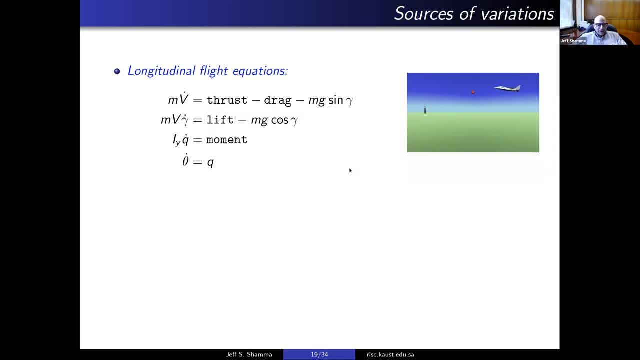 It's obsessed with variations, And what do we mean by that? And so here we have a kind of a flight control 101, a set of equations that represent longitudinal flights. And what are some possible variations in these equations? Well, there's external environmental effects, could be disturbances. 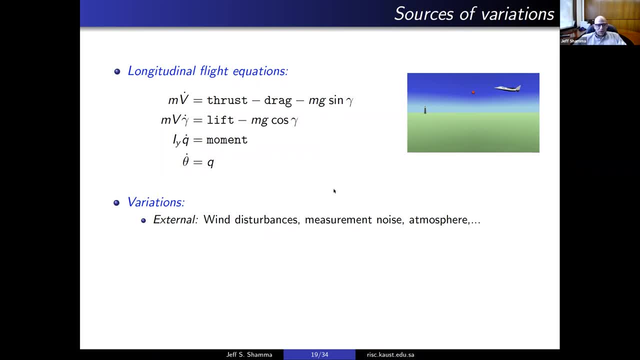 It could be that when we measure the altitude, it's a noisy measurement of altitude. It could be that the atmosphere is changing and then say that air density is changing, which impacts the various factors going into these equations, And it's helpful to distinguish two types of variations. 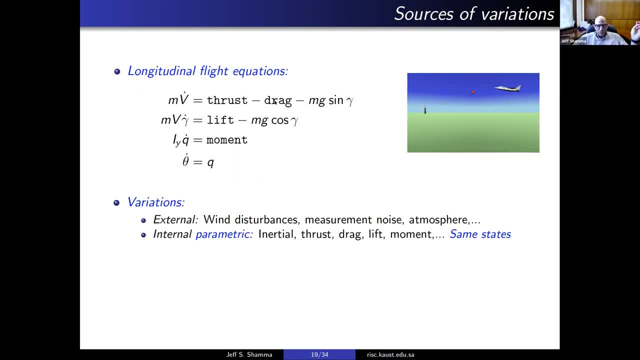 There might be something that's parametric. For example, here I have thrust, drag, lift, mass, various aspects of the airframe. These might be uncertain quantities, but they're not introducing new states. The set of states is fixed. 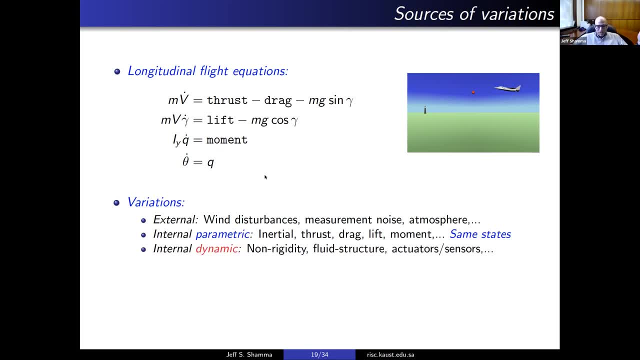 But there's other types of uncertainties- We can call them dynamic uncertainties- where you have to introduce new states. For example, say, the airframe Here might have been modeled as a rigid airframe, but actually it's a flexible airframe. 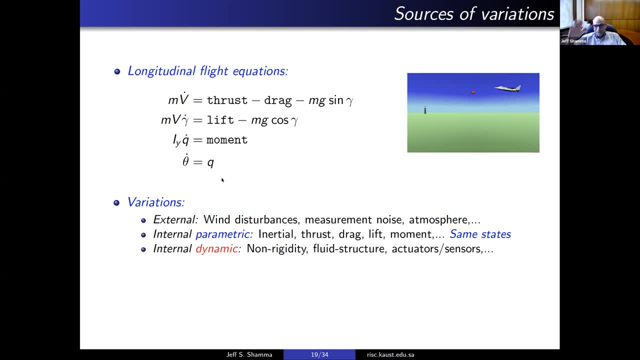 I'm sure we've sat in the window seats and seen the window look like it's flapping. It's not a rigid aircraft. If you want to model that rigidity, then you have to introduce new states. Okay, so we'll call these dynamic uncertainty. 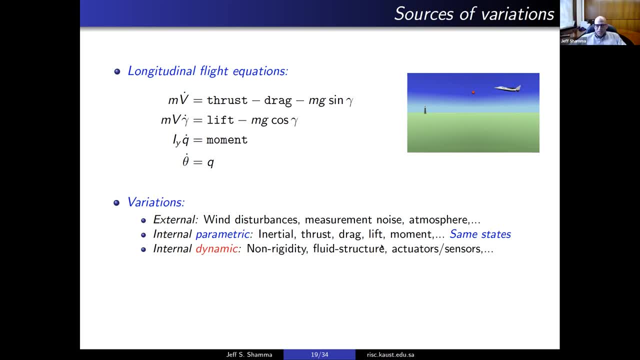 How many new states It could be arbitrarily, or an infinity of new states that will be introduced, And so how can we analyze systems Where we don't even specify the order or how many states there are? And so that is one of the things that is addressed in this literature of robust control. 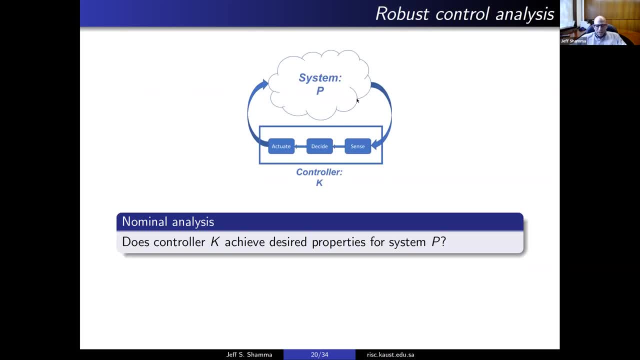 So in robust control, the questions go as follows: There's some system or other actually, So let's back up a bit and talk about nominal analysis. Does my controller work for a particular system? Robust analysis: Does my controller work for an entire family? 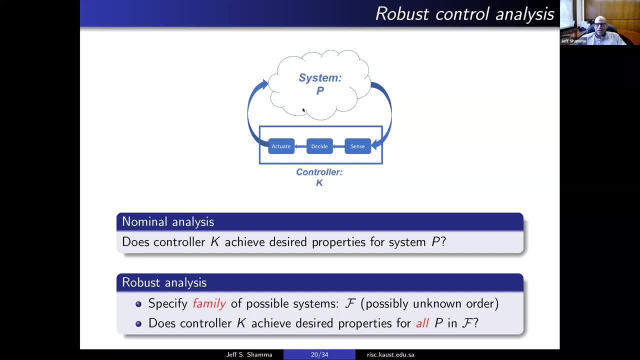 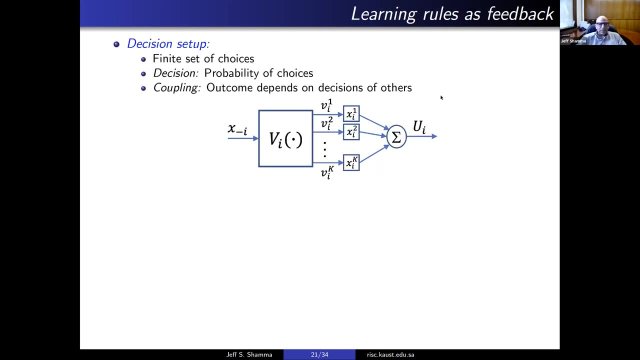 So this is a family of systems. where this family of systems might, it is characterized, but it does not necessarily have a fixed number of states. There's more to it than a model with perturbed parameters, And so now we're going to move to using robust control ideas for learning. 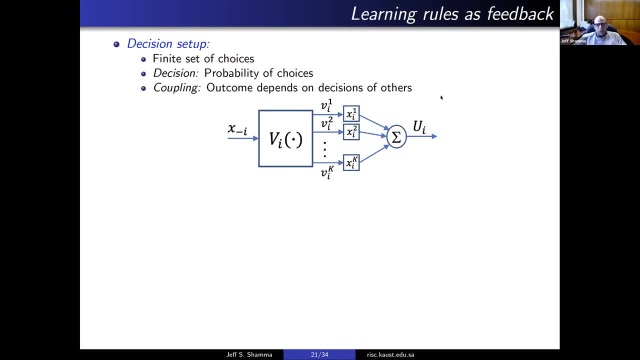 But first I want to make another connection. So what is the decision setup that we're using here? And because it's a simple decision setup that allows us to have this discussion, there's a set of channels, like rock paper or scissors. 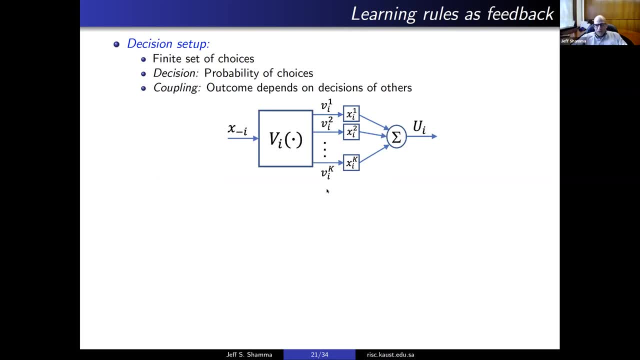 or the different roads in commuting. There's a finite set of channels and I need to allocate resources to these channels. It might be probability of rock, probability of paper, probability of scissors. That's going to be the resources that I allocate. 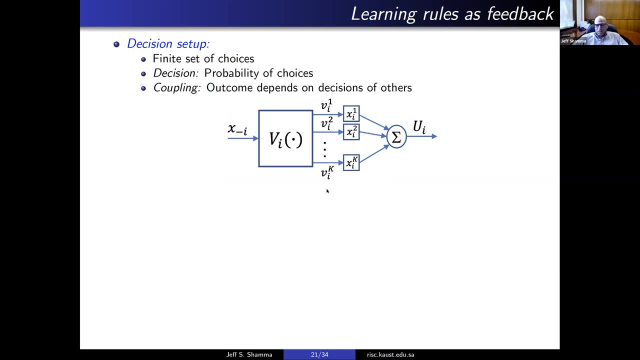 Or it might be: how much of my fleet do I put on each of these roads, Finite sets, and I need to allocate And there's going to be an outcome of that allocation. That outcome depends on the decisions of others. There's the coupling. 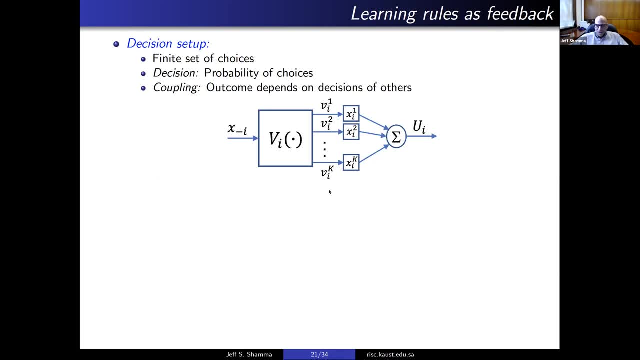 Okay, so this is the setting that we're looking at: A finite set of channels. deploy your resources. What's going to happen depends on how others have deployed their resources. And so now, what does learning look like? When I deploy resources and everyone else deploys resources, that gets processed. 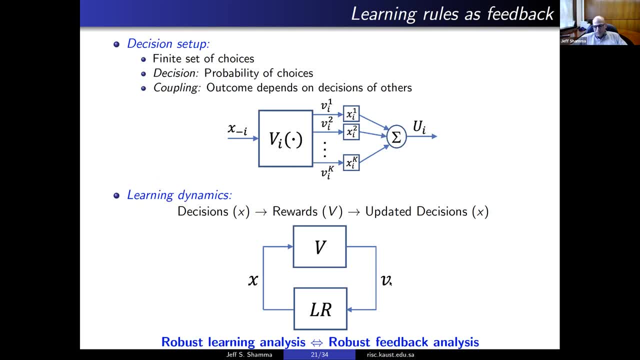 to get to the end of the day. That's when we give everyone rewards. Decisions impact the rewards, which then impact the outcomes, and this cycle continues. So you see that the learning is actually even more explicitly a feedback loop. 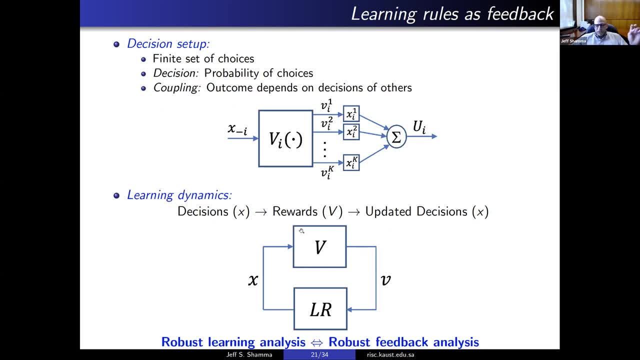 And if you want to make a controls researcher smile, just show them a loop that looks like this: Okay, now we feel that we have a home field advantage where we can now bring our tools to this, to this discussion. And so now, what is robust learning analysis? 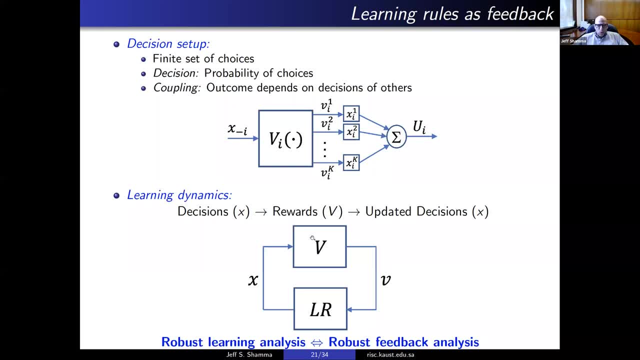 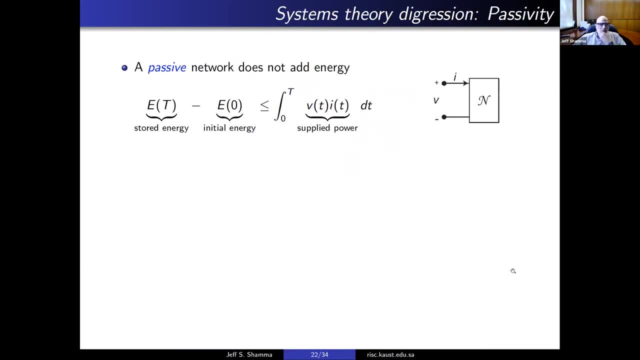 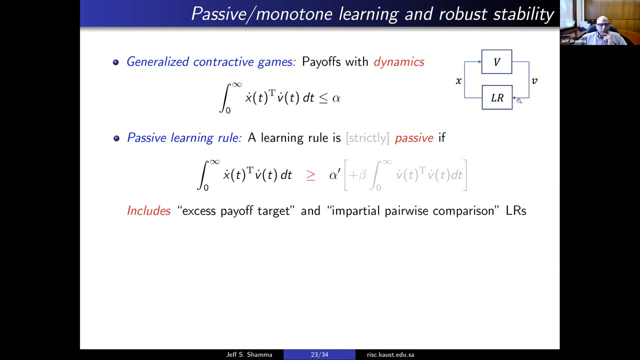 Robust learning analysis will be. when does our learning rule work with the whole family of reward systems or games? I'm going to skip this. where there's a connection to circuits, that I'll just skip And I'll talk about this setting as well. 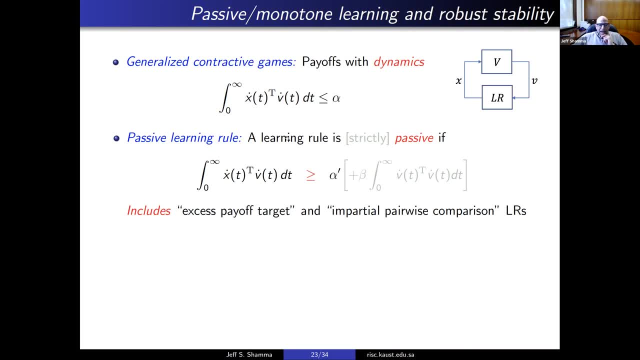 So if a learning rule has this property, okay, And what is this property? This property looks at the flow of resources and the flow of rewards. If the flow of resources and the flow of rewards are positively correlated in the long run and if the environment, it's called a contractive game formally. 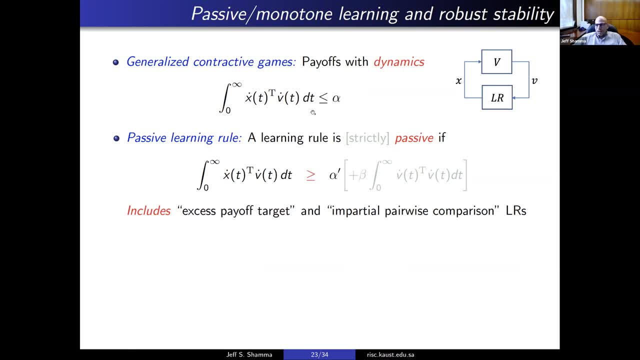 but if the environment has that opposite effect, then if you put these two together, they will result in a stable learning system, And so a passive learning rule comes combined with the anti-passive environment. put them together and they will be stable and they will converge. they will converge, in particular, with a little more analysis. 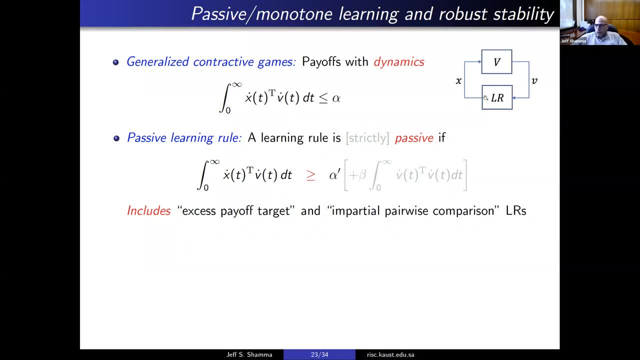 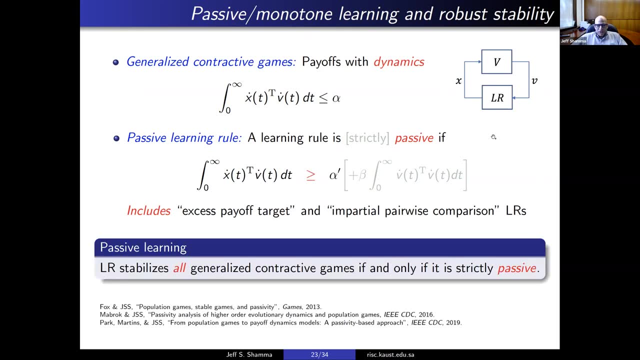 to Nash equilibrium and we haven't mentioned what is the order of the learning rule if it's high order, even we haven't mentioned what's the order of the game. It could be a high order game, but just put these two together and you have a learning scenario. 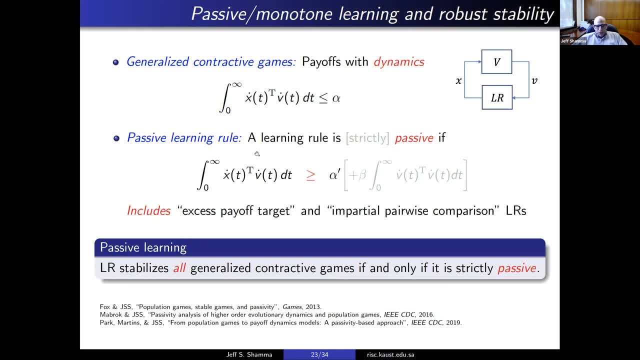 Actually, our result is a bit stronger If a learning rule has this kind of intuitive property that the flow of resources is aligned to the flow of payoffs. and if you want to stabilize all such games, all such environments, it has to be actually, this is a necessary condition. 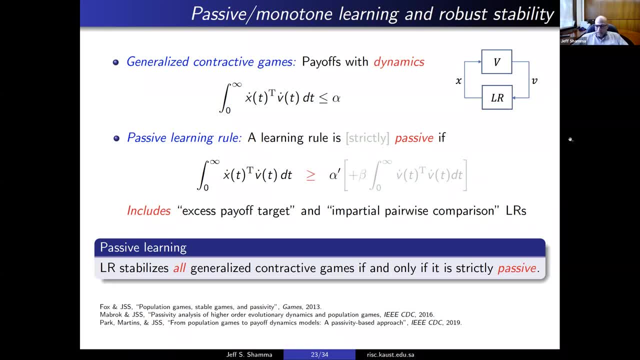 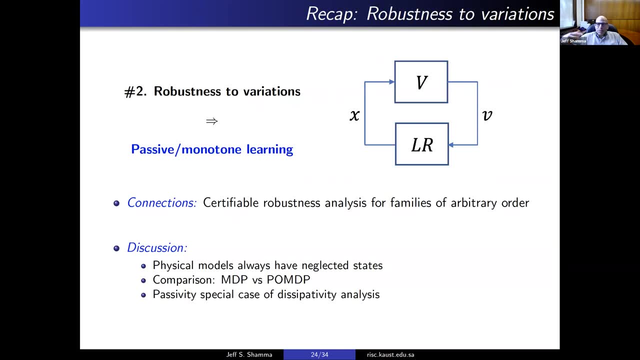 it has to be a passive learning rule, otherwise it can be destabilized. So now we're bringing in tools that allow us to talk about convergence without specifying the order of the learning rule or the order of the environment which with with which the agents are interacting. 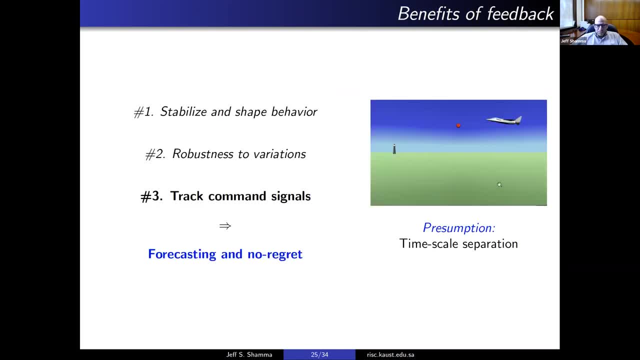 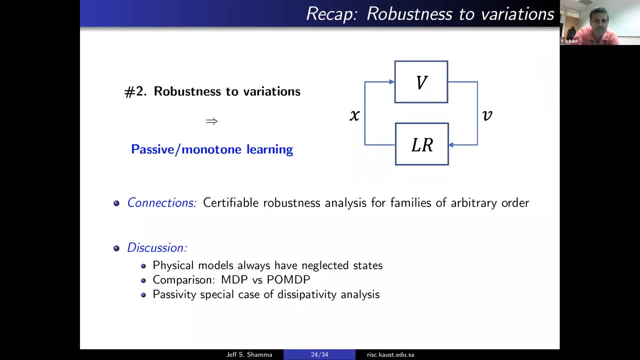 And that is another breaking point, so we can take any questions here. So I'm curious about the comparison between MDP and POMDP. so are you saying that you could think of a POMDP as a perturbation of an MDP? 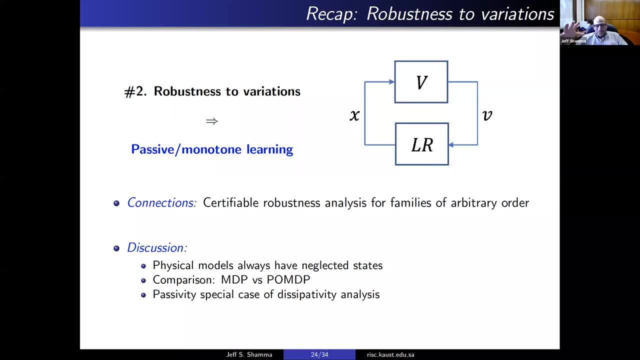 That's what I'm saying, that any MDP. so, if I want to, the comparison is that there's these neglected dynamics such as the aircraft being, Oh yeah, rigid versus flexible. So then I think that, in the continuous state terminology, I think I have 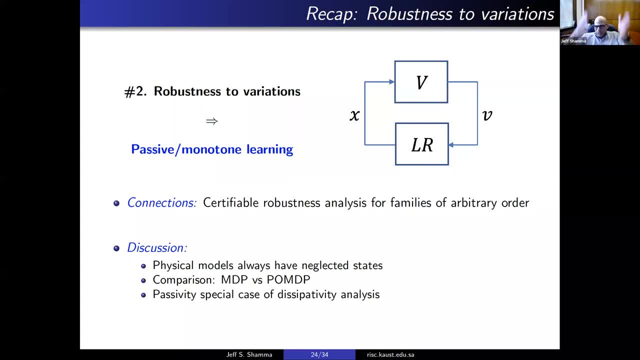 the state but I don't. So it's not actually Markovian in that short list of states And similarly, if there may be parasitic dynamics, so it's not Markovian in the set of states that I've chosen to represent, the states there are parasitic states, states that I haven't modeled. 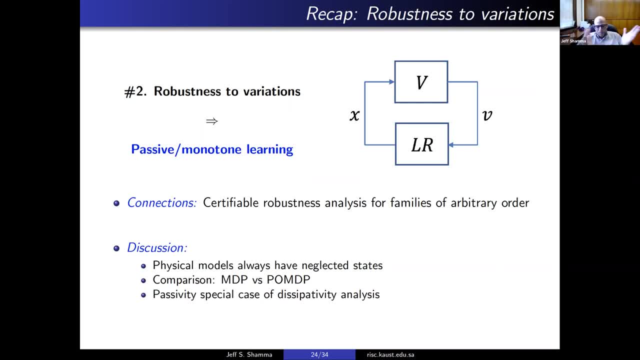 that makes this violate my Markovian assumption. That's a very interesting perspective, because I guess most of reinforcement learning assumes that there's an underlying MDP. What you're saying is that if you make sure that the controller ticket is robust, then it would also be able to handle. 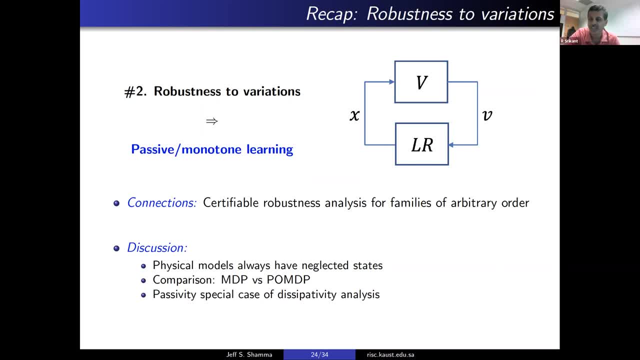 if the states are not what you think they are. I mean there's some other hidden states, Okay. So it would be interesting to look at things, even tabular Q learning, and just say what happens when I'm applying tabular Q learning when it's not Markovian in the set of states that I've assumed. 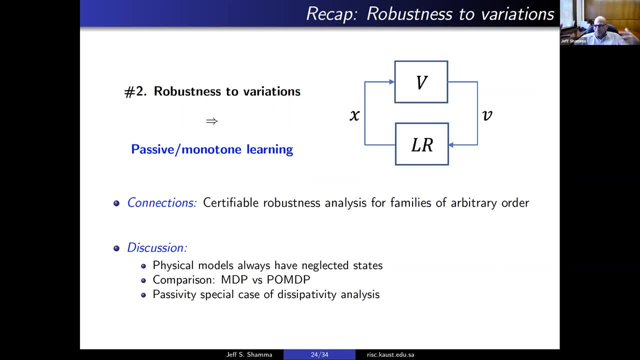 where you'd have to now introduce what you mean by a perturbation, and is there a graceful degradation of performance? That's a great point. There's one more question here. Natural systems tend to handle complex challenges in very smart ways. There's an emerging field of study called 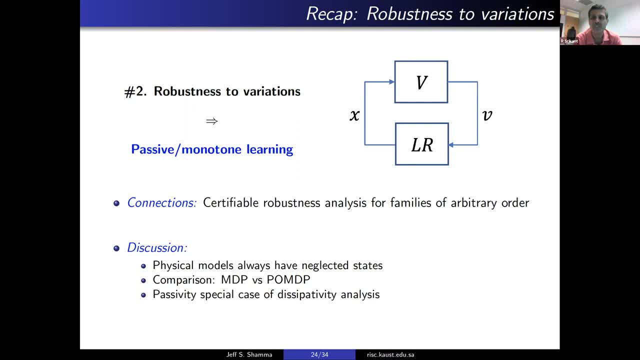 biomimetics. Do you see opportunities in learning from nature and how? I would say that even the anticipatory learning, that is learning in nature. I said that we can't stabilize the aircraft with using the current error. We couldn't stand upright without using the history of say. 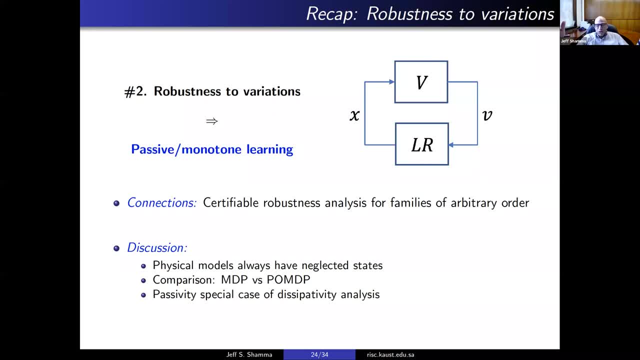 our measurements of trying to stand, And so the learning algorithms that I presented, that use history, are actually very, very intuitive ones and can be confounded in nature, if you will. Great Thanks, Okay. So now we'll talk about tracking command signals, the third in Astrum's list of benefits. 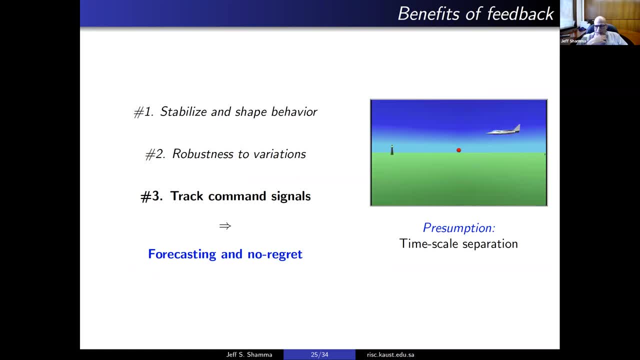 So here's the altitude. We want to follow the bouncing ball, and we can follow the bouncing ball when it's slow, but when the ball starts moving too quickly, we find that we get out of phase and we're unable to follow it, And so tracking a command signal has implicitly that. 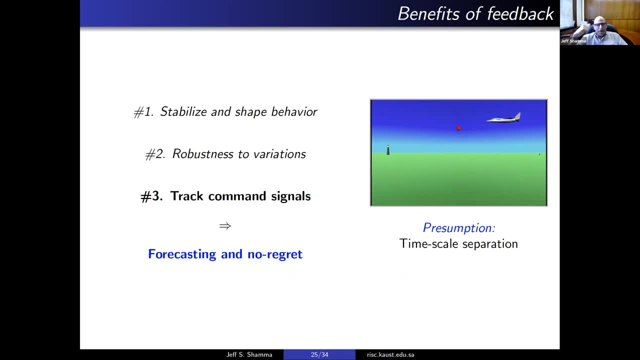 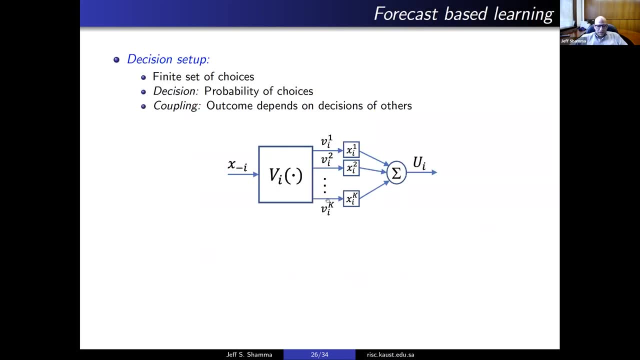 this underlying command signal is slow and we can move it, And so we can move it, And so we can move faster than the command signal. Otherwise we cannot track the command signal, And let's see how this can manifest itself or impact learning. So let's recall our decision setup. There's a set 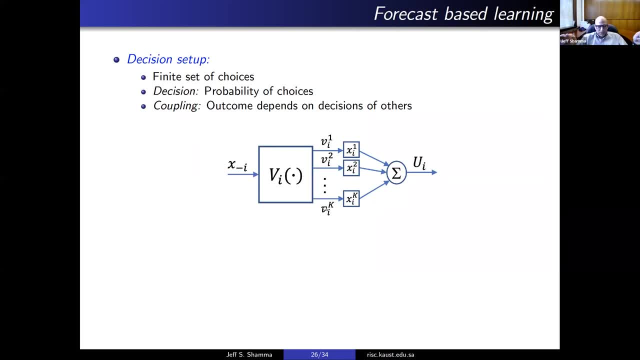 of channels and I want to know how much resource to apply to each channel. Well, if somehow I was able to forecast what's going to be the payoff- yes, it's changing because others are changing, But if I could forecast what is going to be the payoff, 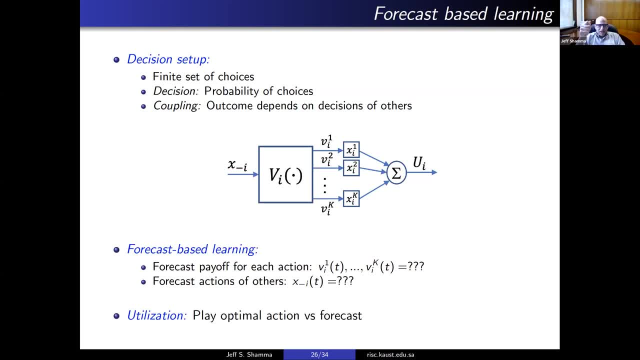 then I can exploit that knowledge and assign my resources according to a forecasted outcome. So either I can try to forecast the consequences of my actions or, if I have the luxury of observing what others are doing, I can try to forecast what they're about to do and then pass that through. 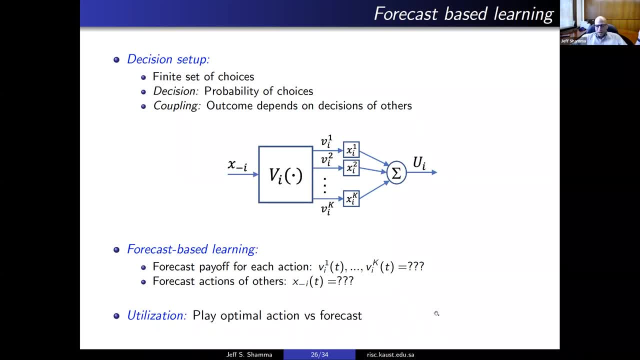 and then know how to optimally allocate my resources based on forecasts. But this is a curious situation to try to forecast because, remember we said, with uncoupled learning you don't have other incentives. I might not have a model of what others are doing. How do you do forecasting when you don't? 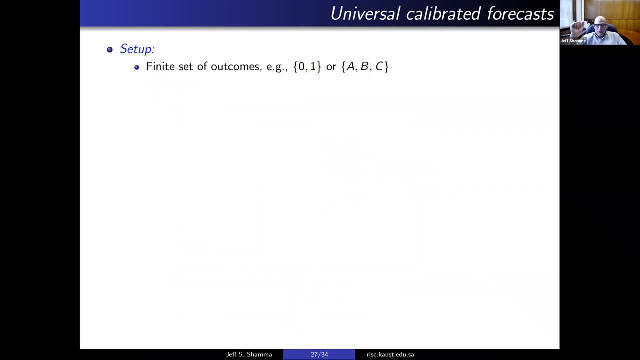 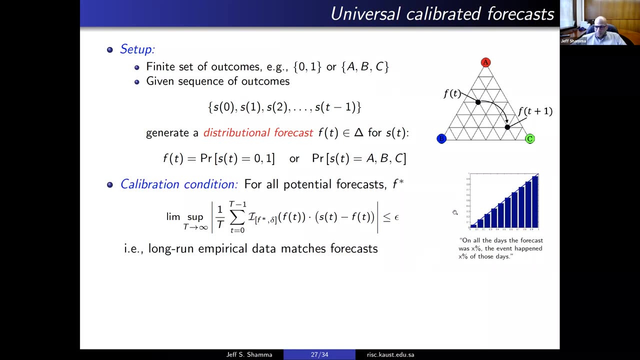 have a model- And actually there's a field for that- of universal forecasting, And let me skip a couple of points here and talk about just this picture. So when the weather service forecasts rain, they don't say it is or isn't going to rain. They'll give a percent chance of rain. 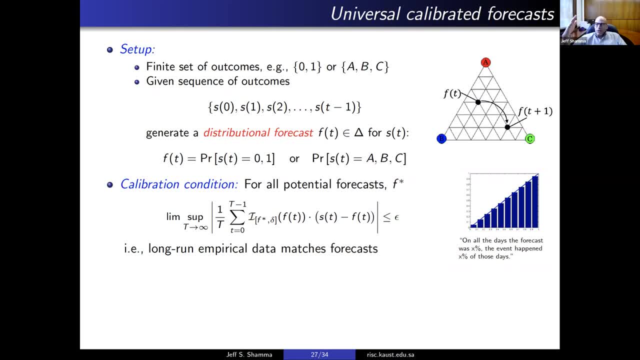 30 percent chance of rain tomorrow. How do you know the forecaster is doing a good job when they're telecasting? What greater incentive that you could offer them? This is your question. How can I know what good job when they never commit to? it will or won't rain. So one way to do that is to use what's. 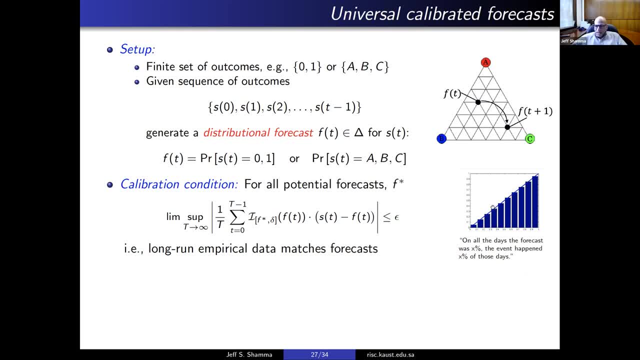 called a calibration condition, And so let's take all of the days that a forecaster said 30% and keep a tally. And in the long run, what fraction of days did it actually rain? And if, in the long run, it's around 30%, well, they did a good job. Well, not in general. 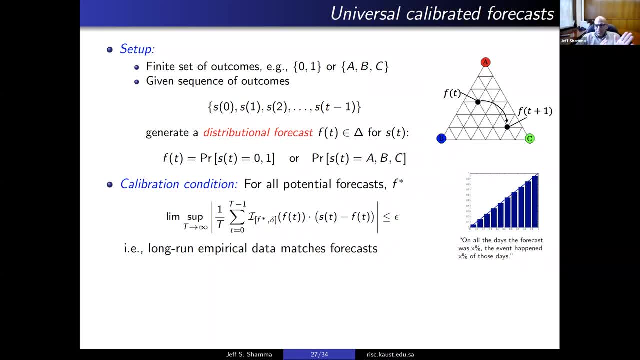 they did a good job. They did a good job when they said 30. But let's test them again. when they say 40%, Let's take all of the days when the forecaster said 40% chance of rain and do a tally, build this histogram And if, in the long run, 40% of those days it rained, they did a good. 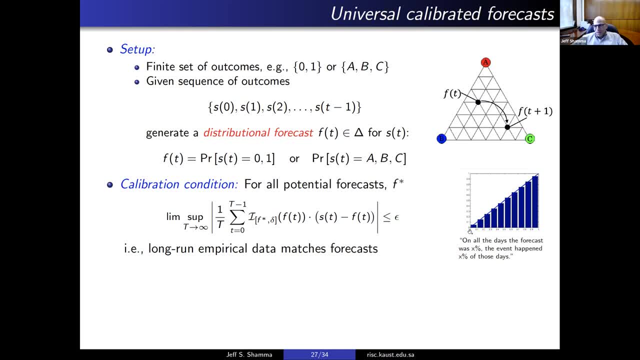 job at 40%, And let's test them at a set of percentages: 10,, 20,, 30,, 40. And if the weather service does a good job for all of these different tests, then we will say it is a good weather. 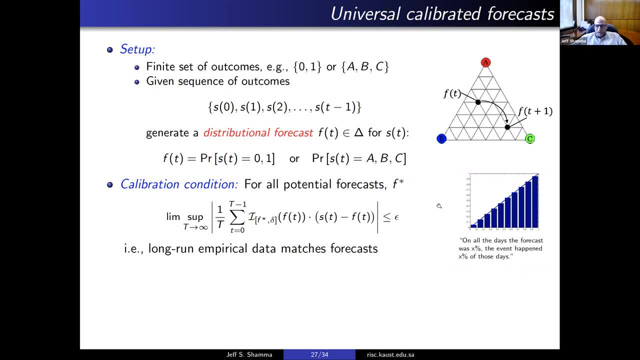 forecaster, It's a calibrated forecast. It turns out that you don't have to know anything about the weather to do calibrated forecasting And there exists universal calibrated forecasting algorithms that, whatever the sequence is, you're going to forecast percentages, likelihoods of outcomes, and you can always get it right. 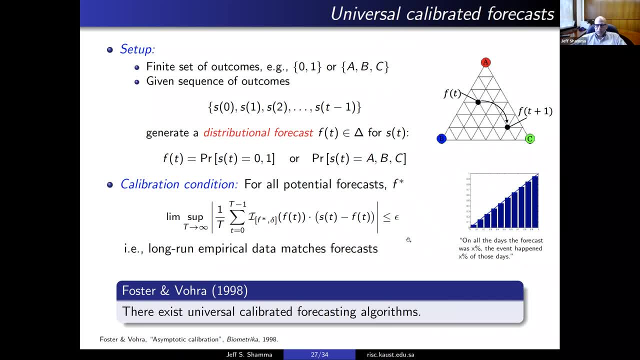 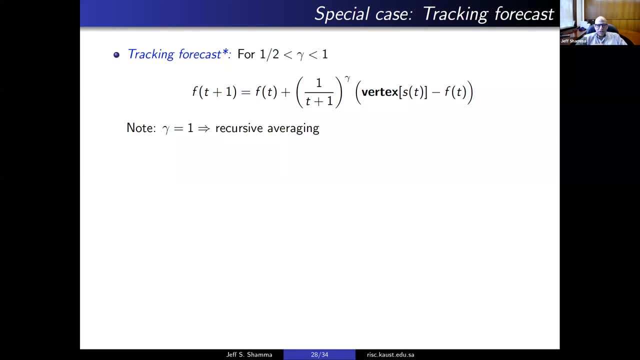 so to speak, using this calibration tools. Those calibration tools tend to be computationally and memory inefficient, but they're universal And what we're going to do here is we're going to do a bit of a trade-off And this is a very, very simple forecasting. And if you've seen recursive averaging before, 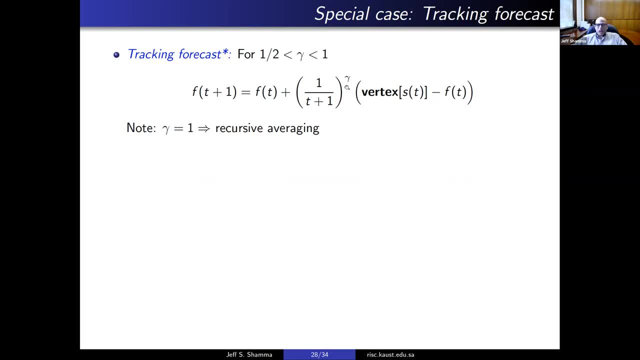 it looks exactly like recursive averaging, except there's a fractional exponent here. Okay, to keep a running histogram with this exponent. And it turns out that this very simple forecast is not universal, but it works on subsets of processes. So again, I don't have 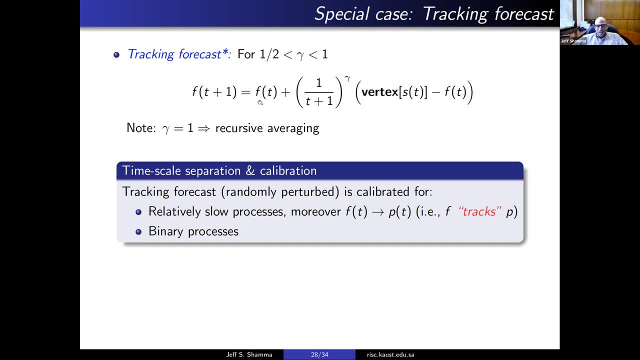 a model. but what is the subset of processes? This forecast works on processes that move slower than my forecast. Remember we talked about this timescale separation. If I can move faster, if my forecast can move faster than the process, then I can eventually figure out that process. 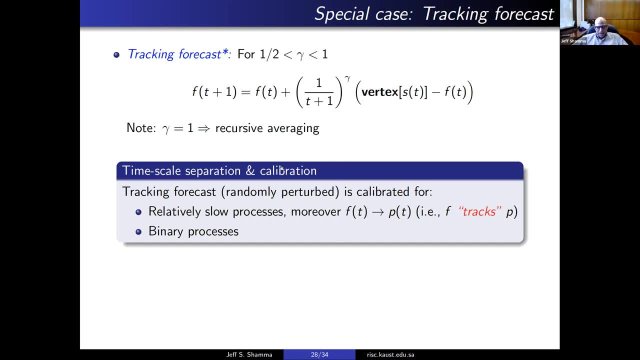 and do accurate forecasting. It's not universal, but that's what we're calling here. This is also calibrated, but it only works for slower processes and some fine prints as well, and other situations. So now I'm in a position. if my opponent is slower than I am, I can forecast. 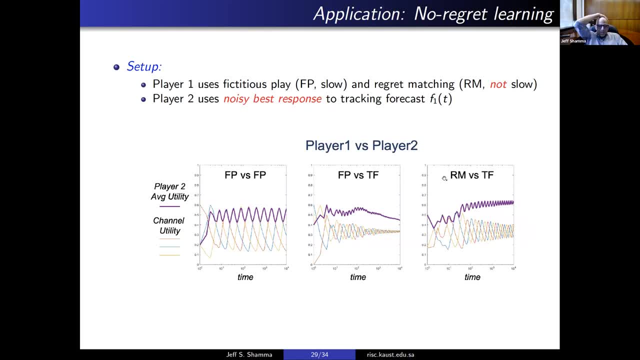 what they're going to do. And here we see a handful of simulations that illustrate this kind of forecasting in what's called a no regret scenario. So you may have heard the term no regret, I won't elaborate. but remember we have a finite set of channels, One naive strategy. 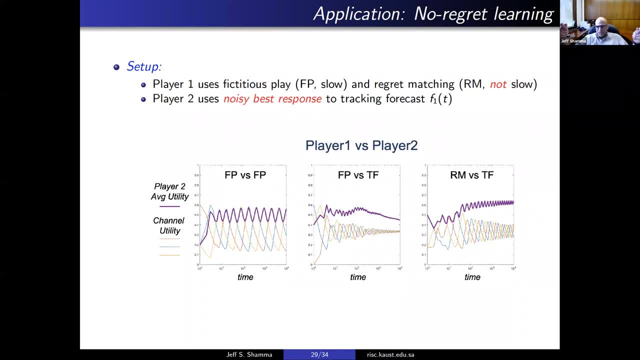 is to use just one of our resources and never use anything. Allocate everything to one channel, No regret, means that our actual long run payoff is going to be better than had we just used one channel and stuck with it. And so here we see, using two. 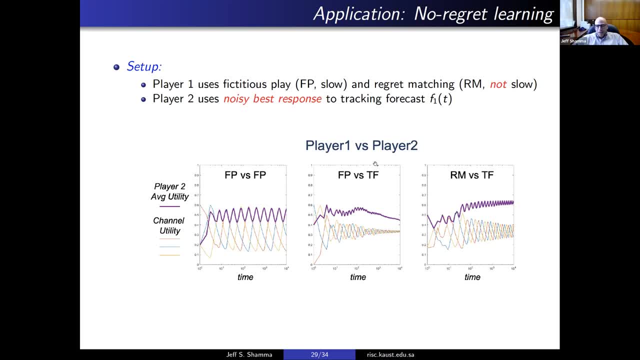 simple forecasting algorithms. but here we see I'm using a more sophisticated forecasting algorithm. I still have no regret, but actually my long run payoff is less. I can be too clever for my own good, because this is a reactionary environment. When I was able to forecast, 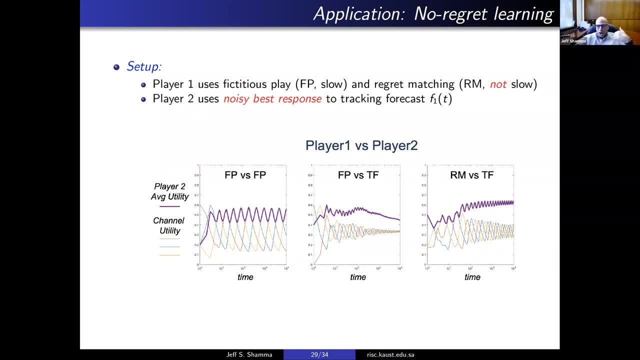 them better. they actually changed their strategy And now my long-term payoff is not as good as it used to be. In both cases you have no regrets, And if you've seen kind of more familiar with no regret algorithms, one of the points I'd like to mention here is that you can have regret for 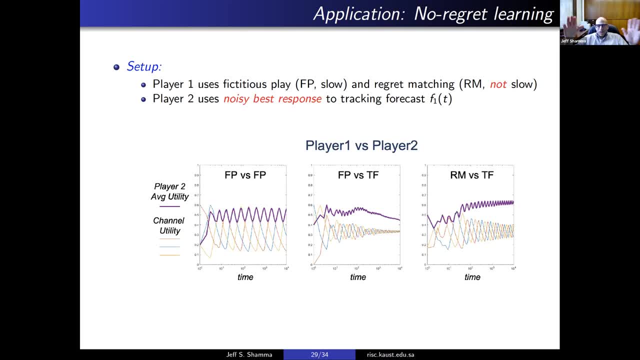 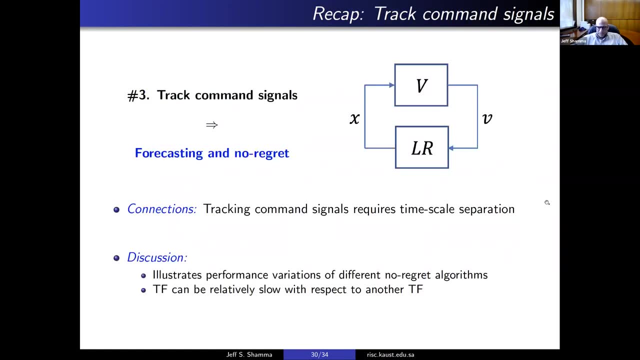 using a no regret algorithm in a reactive environment. One no regret algorithm might outperform another in a reactive environment, So both of them have no regret. And what enabled this was a timescale separation on being able to forecast my process, forecast my environment, faster than my environment actually moves. 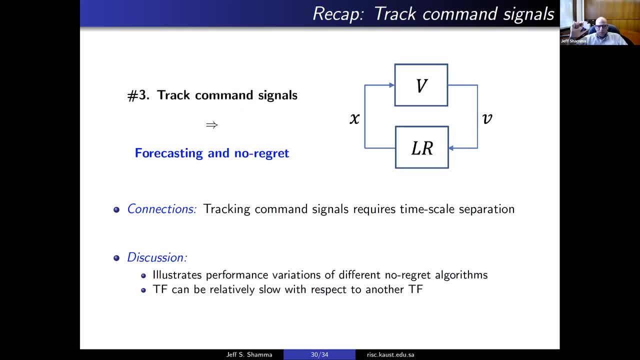 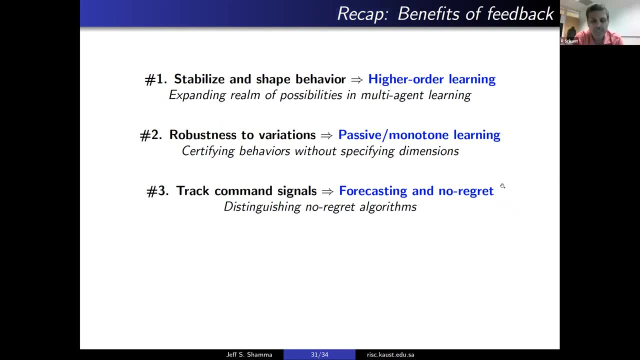 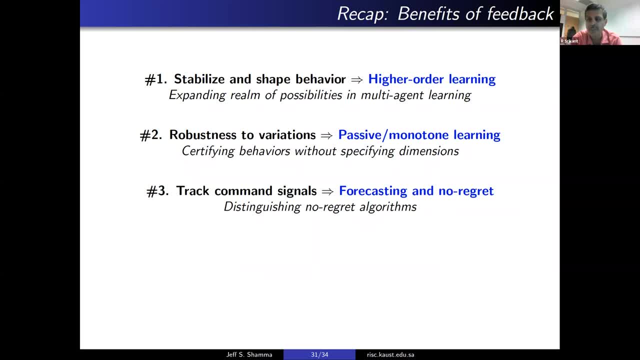 about the timescales that you need to know, about the timescales that you need to know about the algorithms. I mean, or is the, I guess, like, if you look at singular perturbation theory and control, So that's what's happening here Exactly. It's like, suppose you're using a running average. 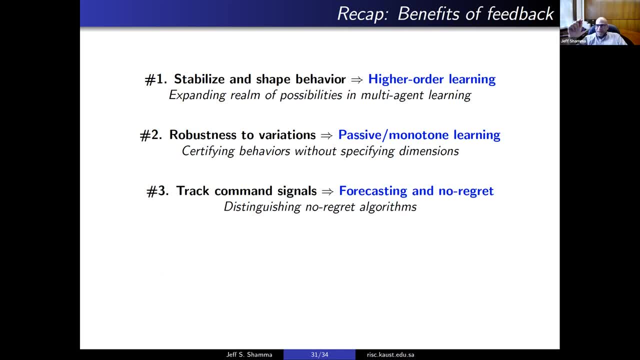 and I'm using this running average that has that exponent, then over time my step size will be arbitrarily larger than yours. So if you're using a vanilla no regret algorithm that does averaging, I'll do this kind of bigger time step averaging And now you have exactly as. 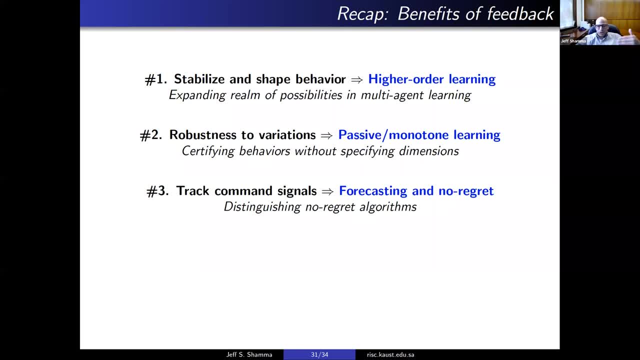 singular perturbation apply to two-time scale stochastic approximation. That's exactly the analysis. Okay, thanks, Okay, so we talked about these three benefits of feedback, Stabilizing and shaping behavior. that led to higher order learning and it let us better understand what. 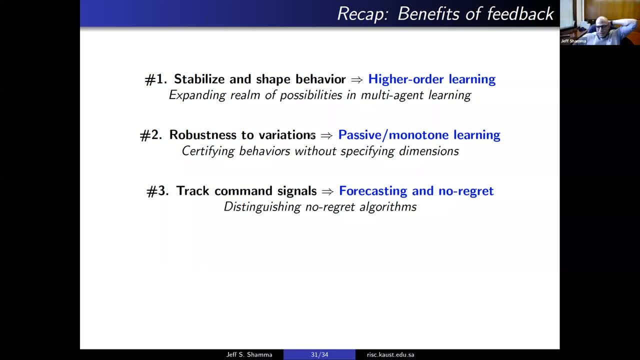 is or isn't possible in multi-agent learning, Robustness to variations made a connection to passive or monotone learning, and that led us to start to talk about the behavior of learning rules without imposing the robust behavior of learning rules, without imposing the dimension. 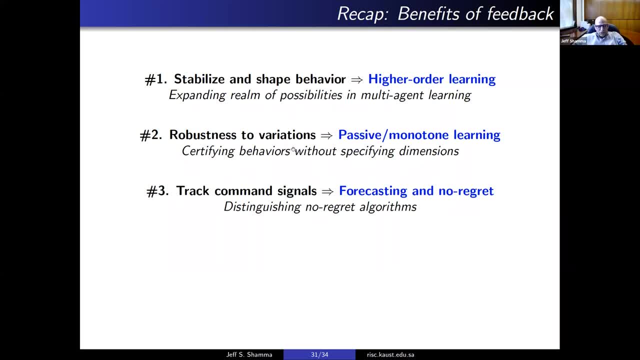 of the underlying entities And then tracking command signals has this built-in time scale separation, and that led us to look at forecasting approaches to learning and understanding what happens when you have a time scale separation, but also leading. this is more of a question than an. 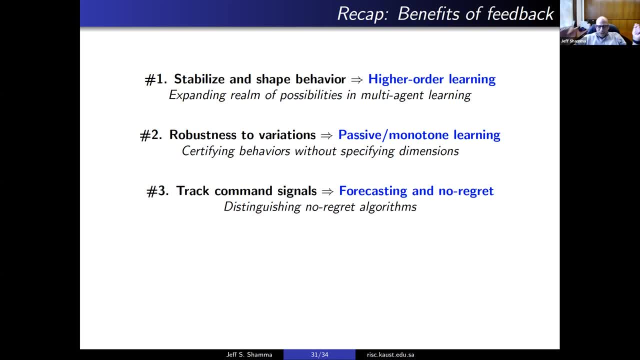 answer Two: can I regret using a no regret algorithm? So these are all things that controls can do, and before we get too excited, it's important to talk about the limitations of controls and what controls cannot do, And so here I'm going to talk about a waterbed effect. 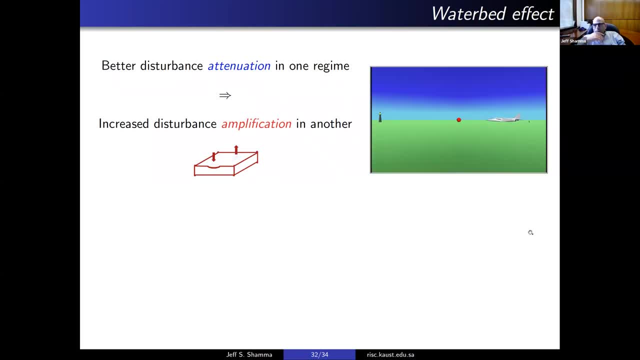 and what I'll illustrate here is again following the bouncing ball. there's a wind disturbance on this aircraft, and so it's able to follow the bouncing ball pretty well when the wind disturbance is at a- you know, a certain level of difficulty, And so it's able to follow the bouncing ball pretty. 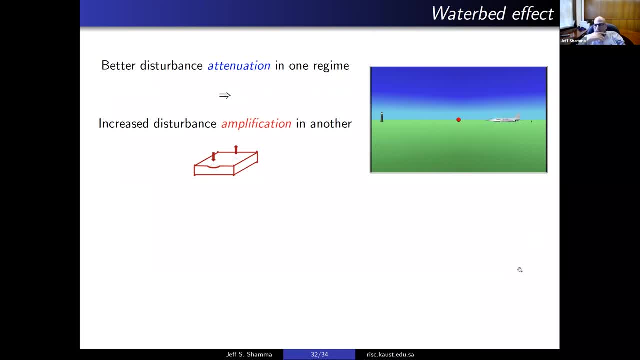 well, when the wind disturbance is at a specific frequency. But if I change the frequency of the wind disturbance, it cannot follow the bouncing ball, it cannot maintain altitude at all. Okay, so how come it does it at one frequency and not at another frequency? Well, the more the other. 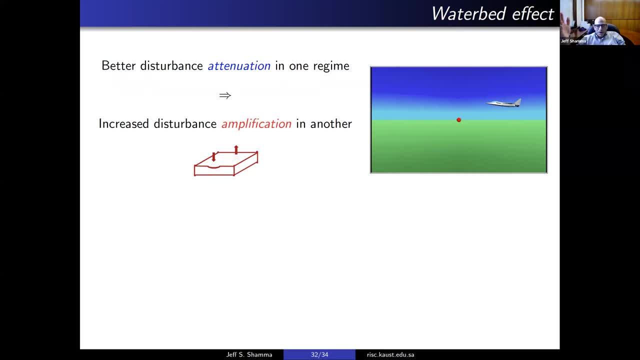 question is: is that there's a built-in waterbed effect in that the better I reject disturbances at one frequency, the worse I'll reject disturbances at another frequency. You can't have it both ways, Okay. So good performance at one frequency will lead to worse performance at other frequencies. This is a 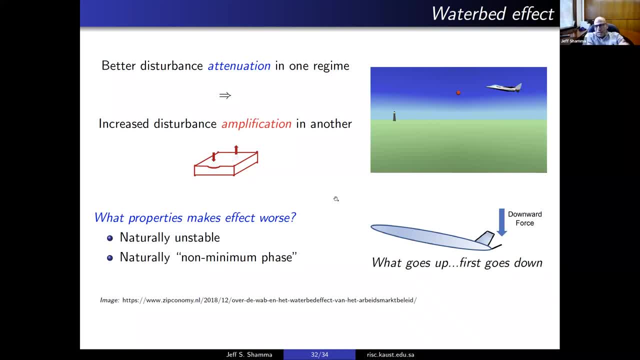 so-called waterbed effect. And there are some features that make waterbed effects even worse. And one feature is when systems are called non-minimum phase- And I'm not giving the technical definition here, but I'll give an intuitive definition- is that when, suppose I? 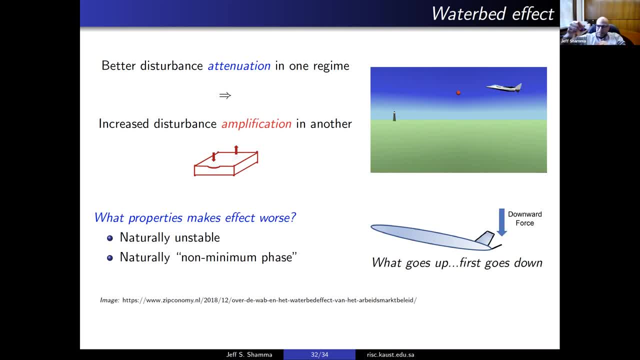 want to make the aircraft go up, then I have to lift the tail. But when you initially lift the tail, the aircraft will go up, And so I have to lift the tail. And so I have to lift the tail, And the first effect is that the aircraft goes down. For an aircraft to go up, it has to first go down. 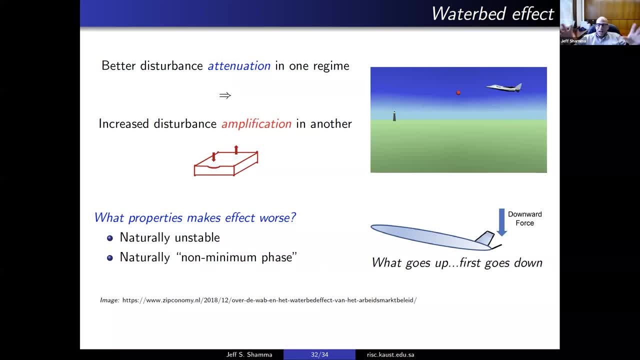 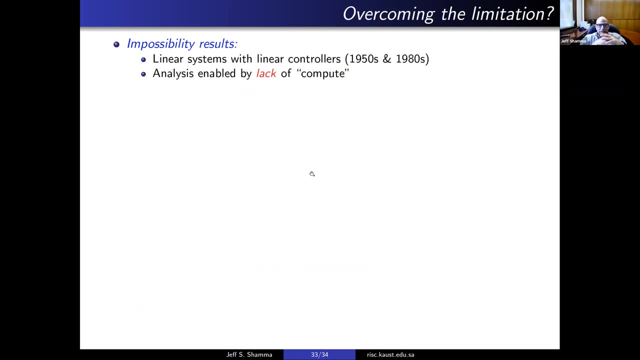 This is like a non-minimum phase behavior. If a system has a non-minimum phase behavior, then the waterbed effect which was there is actually even worse. So the better I do one frequency, the even worse I will do at other frequencies. So what causes the waterbed effect? 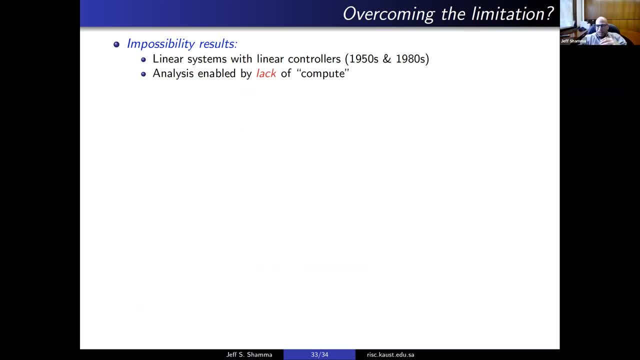 Is it due to, a kind of say, a lack of sophistication in the controller, And so there's a lot of analysis that said, if I have a linear system and use linear controllers, then you're going to have a waterbed effect. That was in the 50s. There was pioneering work in the 80s here in Illinois. 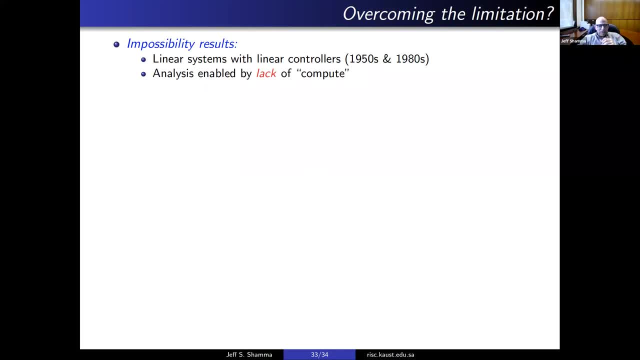 that generalized that to multivariable systems and again established and quantified for multivariable systems this waterbed effect, And this is motivated by, say, a lack of ability to do computations as to understand what are these trade-offs when it's limited on. 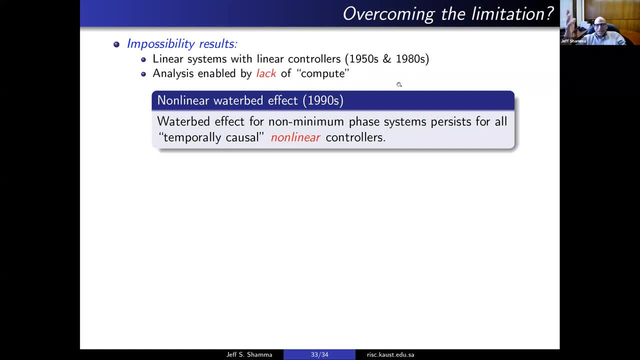 how sophisticated a controller I can use. But there's actually a nonlinear waterbed effect. that was established in the 90s And it says, even if you use a nonlinear controller, that you will have a waterbed effect. The only restriction on your nonlinear controller is that it can't tell. 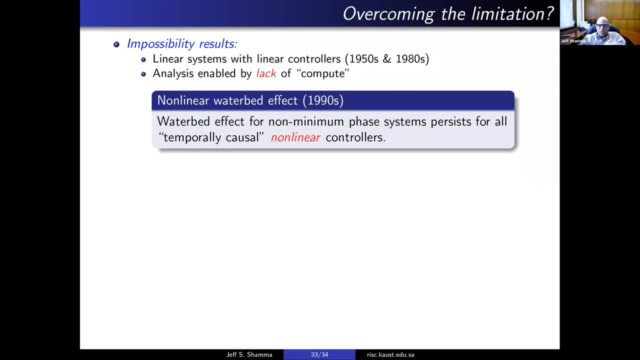 the future. The action that it takes today is a function of the measurements that it's taken today and in the past. The action that it takes today cannot be a function of tomorrow's measurement. So if you have a causal controller, a temporally causal controller, so this, for example, could be: 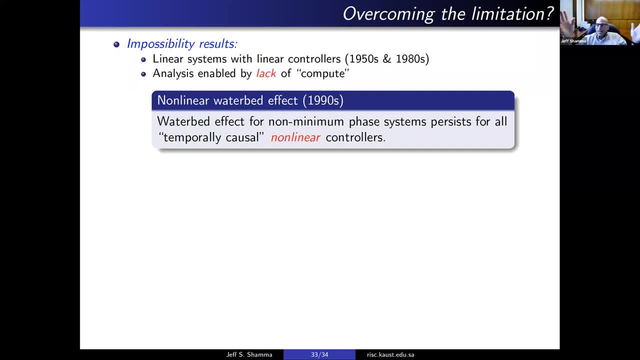 as sophisticated as you want of a neural net, it cannot overcome the waterbed effect. If it does good disturbance rejection in one region, it will do poor disturbance rejection in another region. And to now reference Stein's lecture from 1989, he didn't call it the waterbed effect. 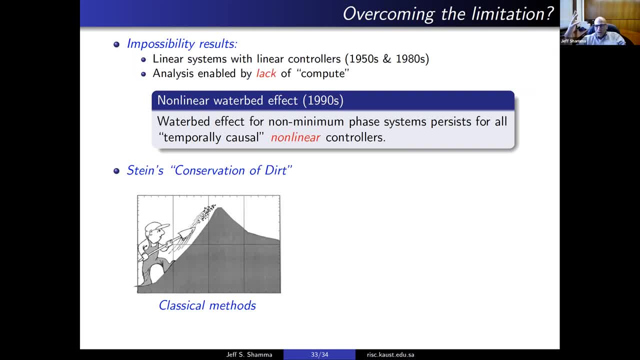 At the time he called it co-efficient. He called it conservation of dirt. You can't get rid of dirt. You can move it from one place to another And if you use good, old-fashioned methods, this is what conservation of dirt looks. 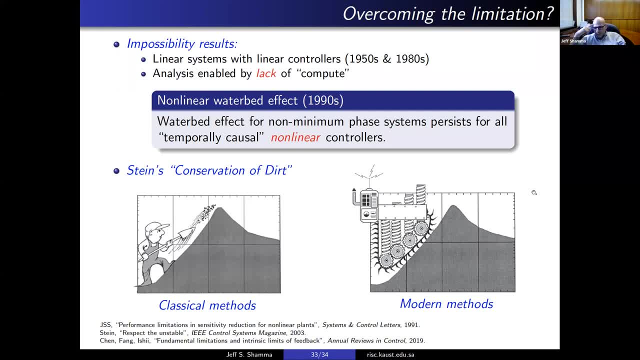 like If you use sophisticated methods. this is what conservation of dirt looks like, But you still have the dirt. You cannot get rid of it. And again, using very, very sophisticated learning, controllers cannot bypass a waterbed effect. So this is something that controls cannot do. 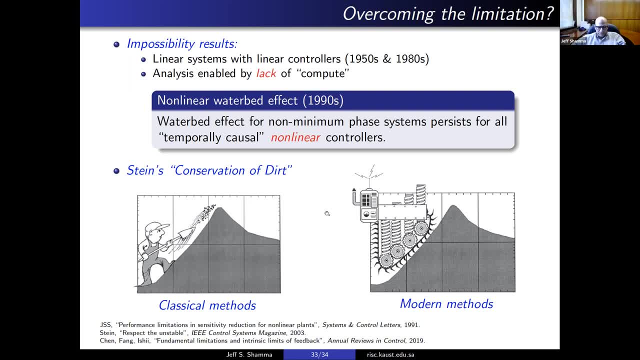 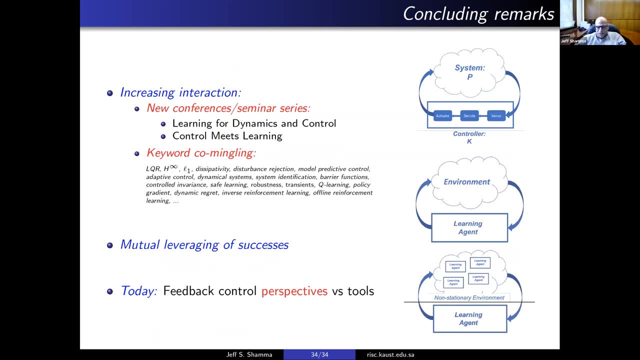 but it's something that any causal system cannot do, And okay, so that brings me to the concluding remarks. You're seeing a lot of interaction, and this colloquium has brought it, and there were some other colloquia that were being held. 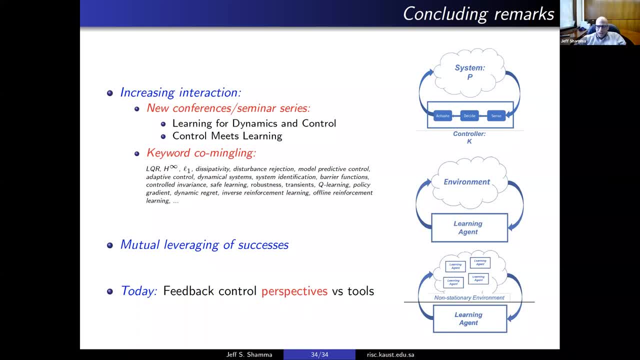 through C3DTI that also brings together these communities of learning and controls. There's now a conference called Learning and Controls. There's a seminar series called Controls Meets Learning. You're seeing a commingling of keywords. You'll see papers that talk about learning and 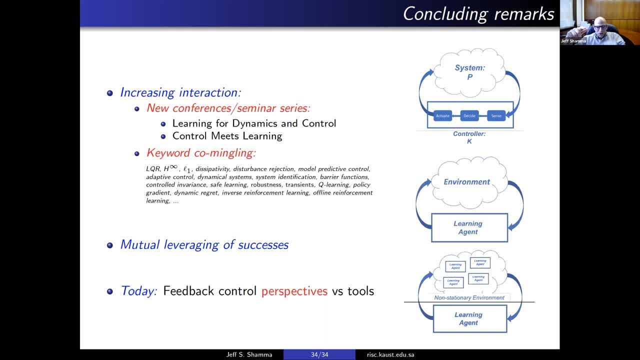 control. You'll see papers that talk about no-regret approaches to LQG. That's all kind of jargon, but the point is that that jargon didn't mix 10 years ago and now you're finding more mixing. What's bound to happen is a leveraging of success in each community, and I think it's. 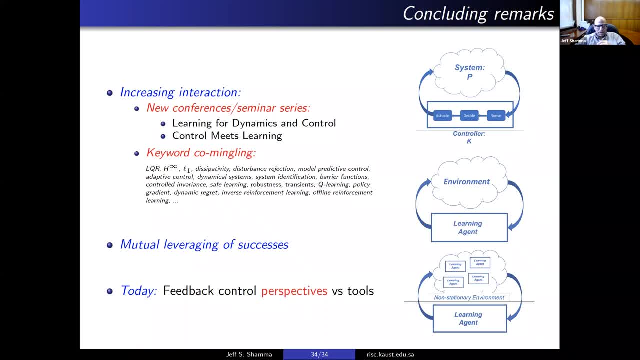 very exciting time to be watching these kinds of results unfold. I did talk about what controls can do what it can't do. This wasn't meant to be a presentation of tools, but rather it's a presentation of a perspective of how we can do this, And I think it's a very exciting time to 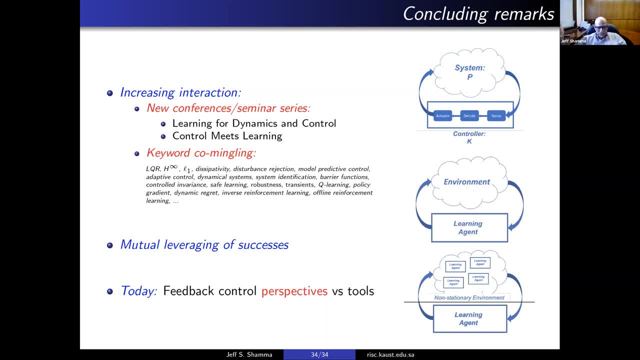 see how a control researcher might think about learning, and so it's inside the mind of a controls researcher, And so with that, thank you very much. Thank you, Jeff. That was a wonderful talk. Some of you may know, Jeff was invited to give a talk at 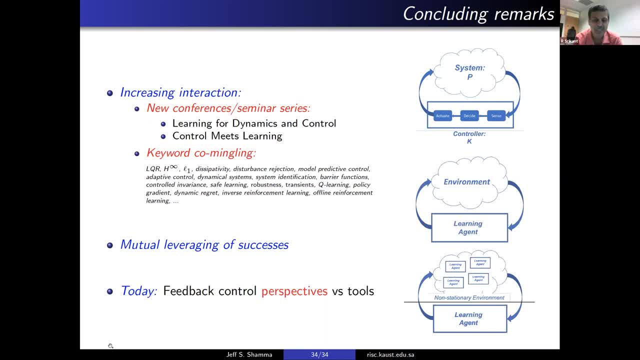 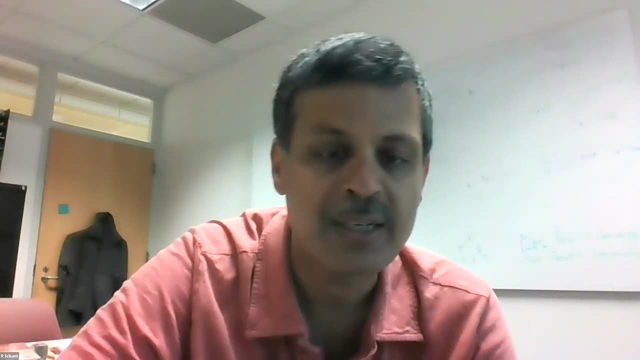 the main machine learning conference in Europe, and I guess machine learning people are very, very interested in understanding what feedback control does and what control theorists have to say, and this is a wonderful perspective, combining basic control theory and multi-agent control and so on. So if you have any other questions, 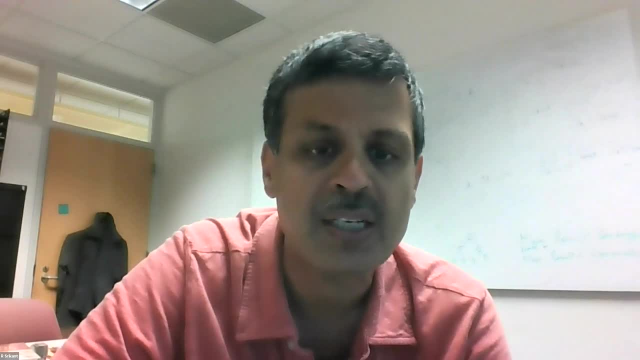 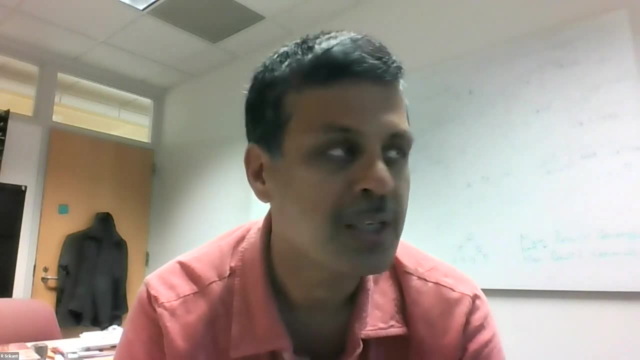 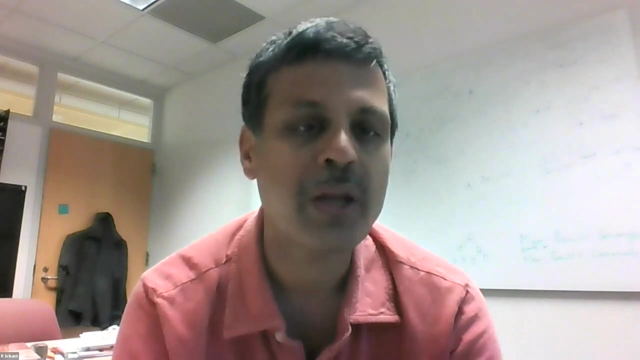 okay, I guess this is the previous question that's still here. I guess one question that I have is: there's been a lot of interest in what is called multi-agent reinforcement learning, and I guess I don't know if people are unaware of this or not, but people seem to assume at least some. 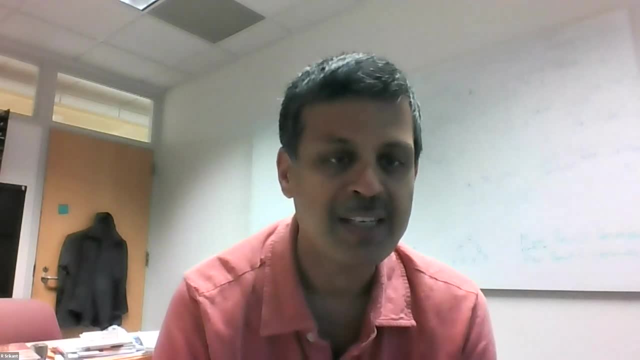 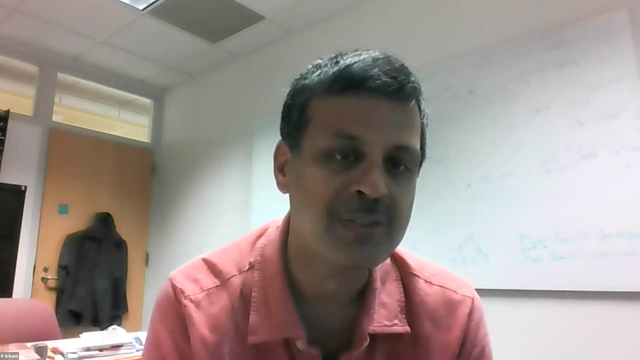 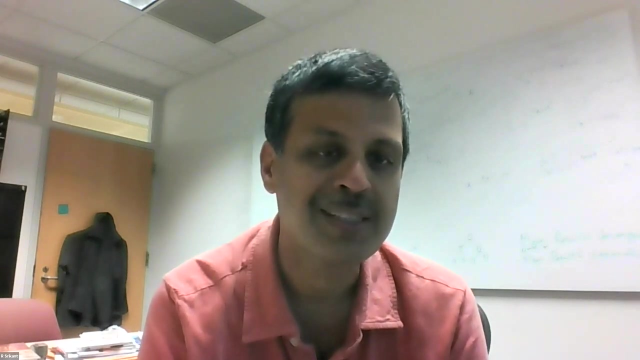 of the talks that I see or the papers that I see, are trying to design controllers where different agents have different measurements. I mean so this is central system, state X, and I have Y1 and you have Y2 and somebody else. But we know from the basic Wittsenhausen counter example that there 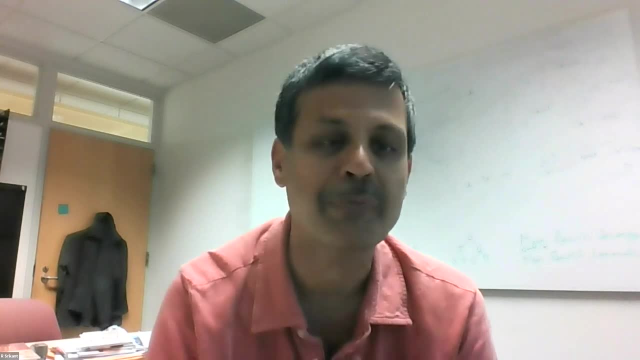 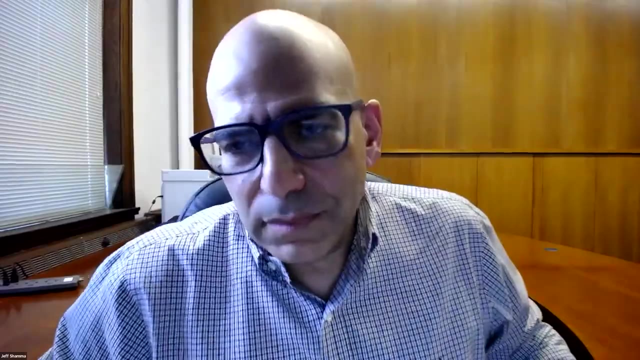 is, solutions to this are just extremely difficult to find, Even from a computational perspective- this famous paper by Tsitsiglis and Papadimitriou. So are people unaware of this? Are they just interested in just finding some local minimum using policy gradient and they're okay with that? 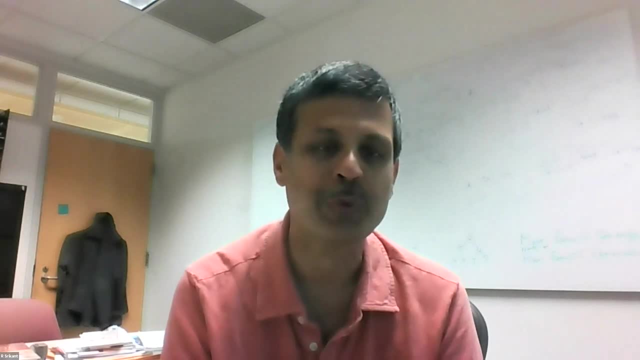 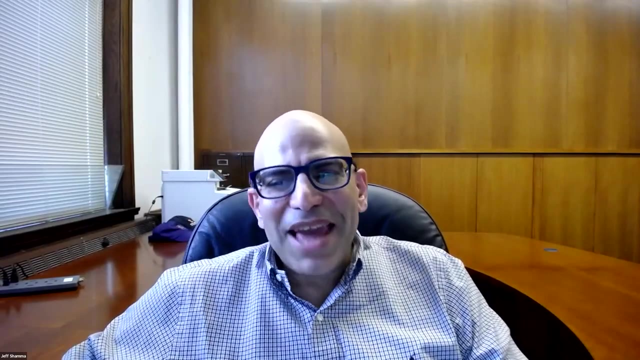 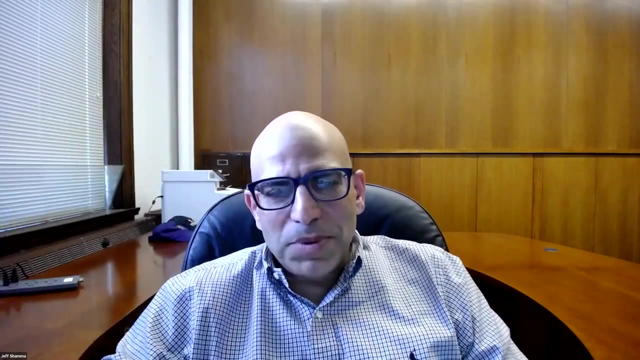 I haven't been able to get a proper answer to this question, and I was just curious what you thought of it. It depends on the people and who's aware of what, and also the angle that they're coming in. For example, let's take this issue of uncoupled dynamics, And so it was an obstacle. We were able. 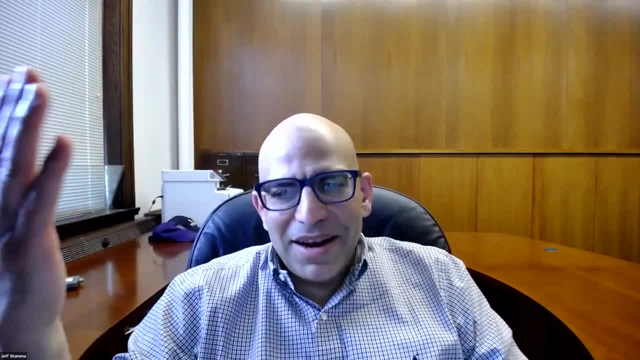 to overcome the obstacle using memory. but the point is that, is that an issue? Whether or not that's an issue? if you're mindful of it, it's not an issue. If you're mindful of it, it's not an issue. 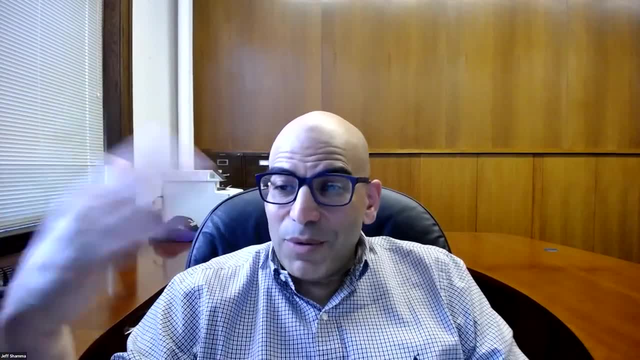 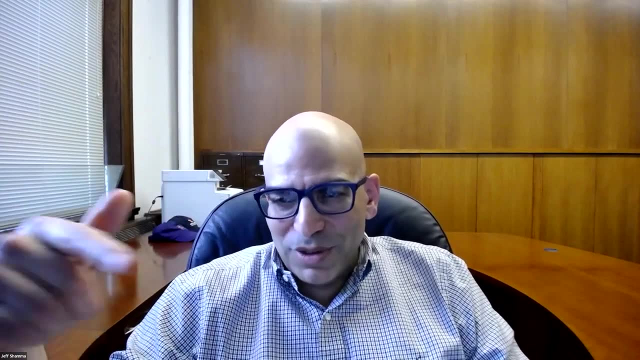 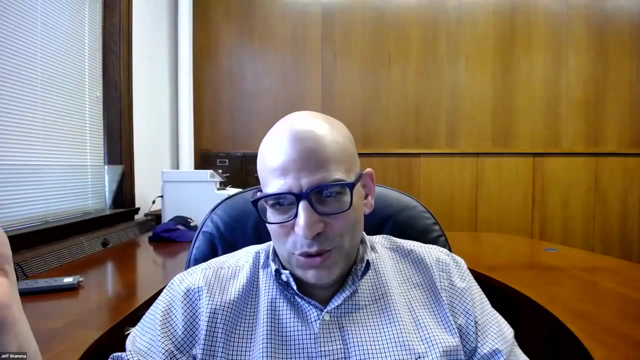 If you're modeling human decision making, multi-agent human decision making, it remains an issue. If it's engineered systems, then whether or not I know your utility function or the details of utility function, it's other considerations. So do we have the energy to communicate? 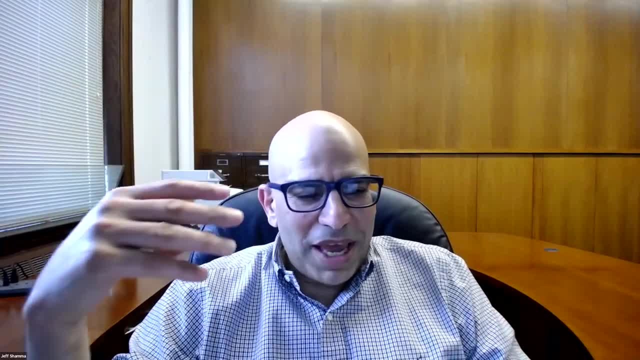 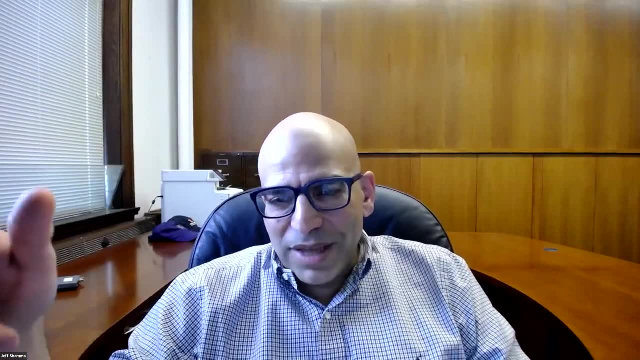 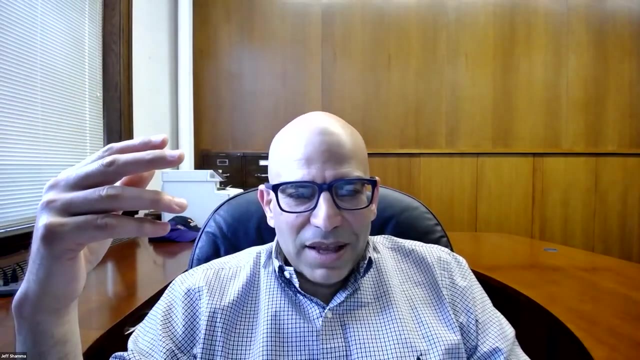 to share that information? Are we in a communication-denied environment? I have the energy, but not the channel. Is our environment too complicated? For example, what we talked about commuting, or this also happens- say in routing and communications that I can go from A to B. 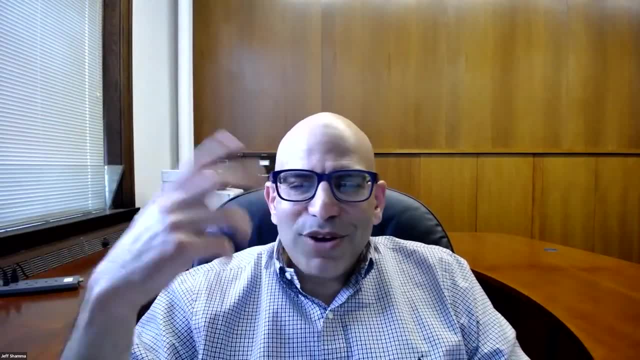 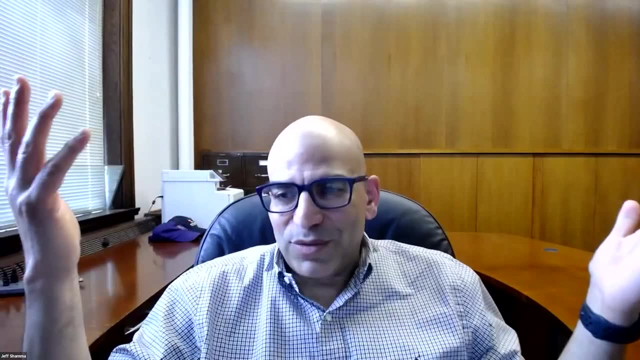 and measure how much time it took. But I do not have a closed form expression of how much time will it take as a function of the cars and the time of day and the weather. I don't have this, this function, So it could be that I don't even know my own utility function. But the point is 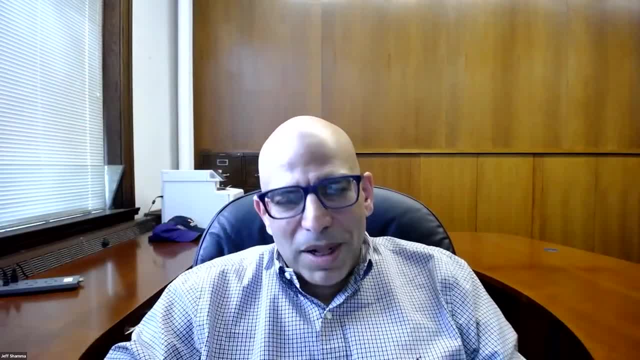 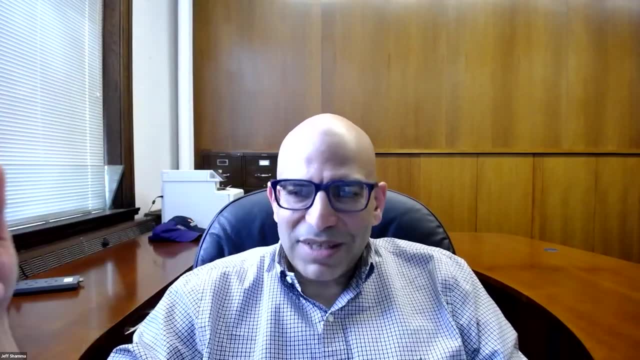 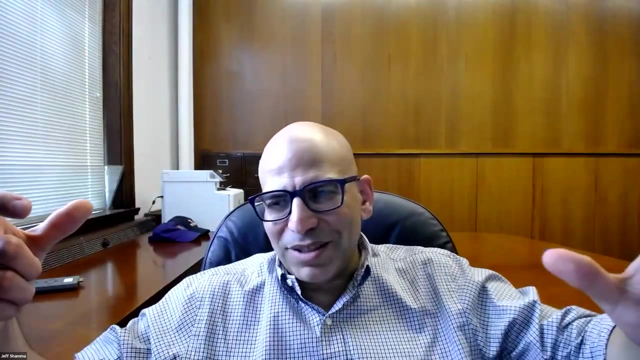 that it's different considerations. So now for multi-agent reinforcement learning. there's been a lot of work from the game theory perspective. There's been a lot of work in the CS perspective along the lines of if I take a single-agent learning algorithm and plop it into a multi-agent, 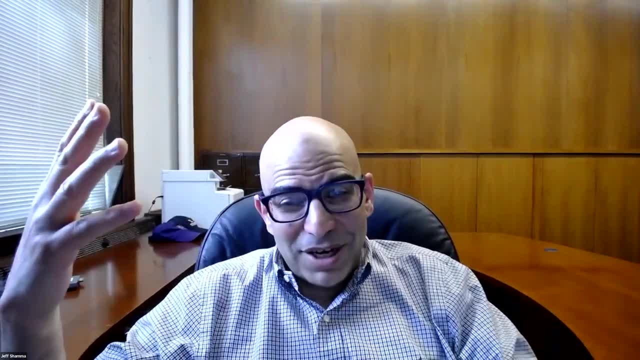 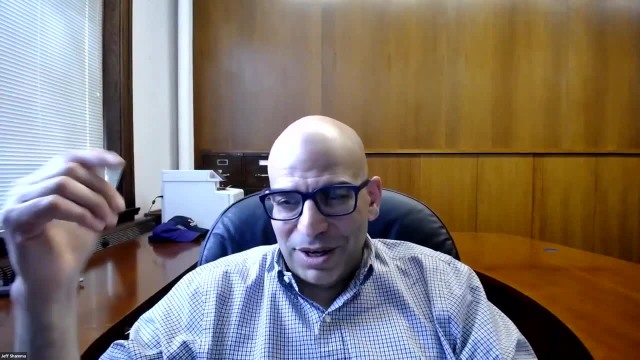 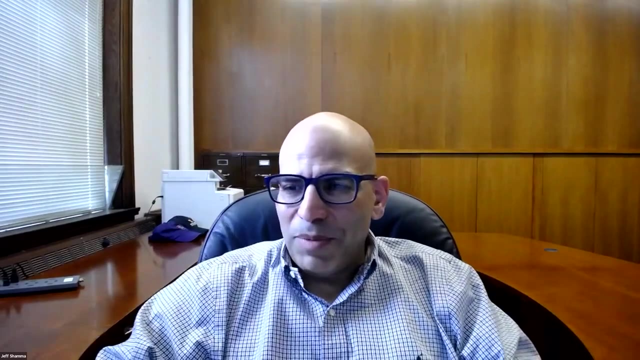 setting what can go right, What can go wrong. But if it's an engineered system, we can cheat. And then what's the penalty for cheating? It's engineering considerations, Again. communications, energy, stealth, complexity, they all impact, But we're not. 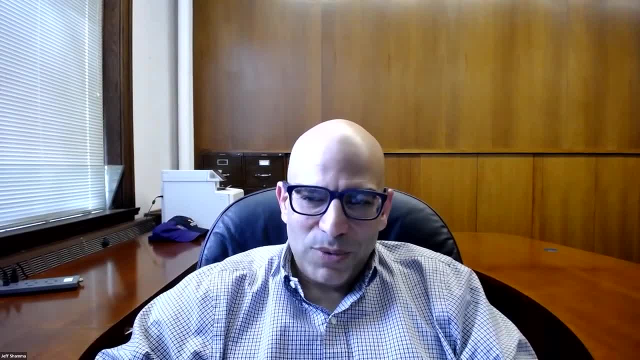 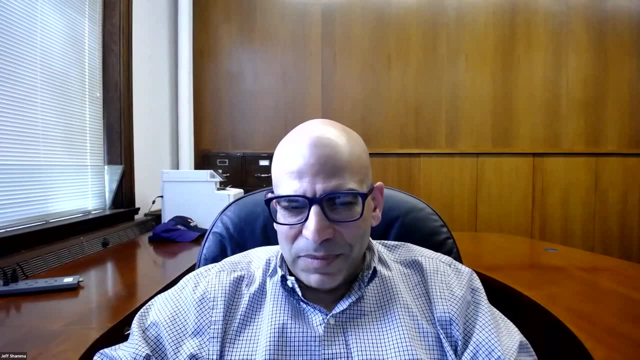 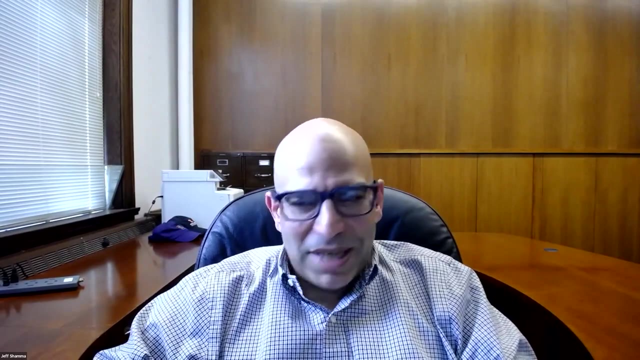 taking it as a constraint. It doesn't have the same constraint as when it's human in the loop. So I think that there is a pretty good awareness- maybe not at depth, but when the more recent literature I've seen on multi-agent reinforcement learning seems to be taking the cheating approach. 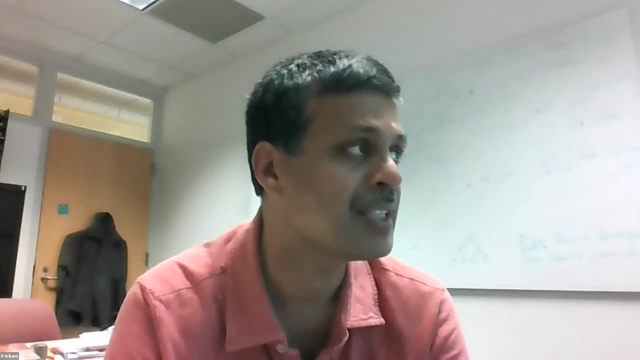 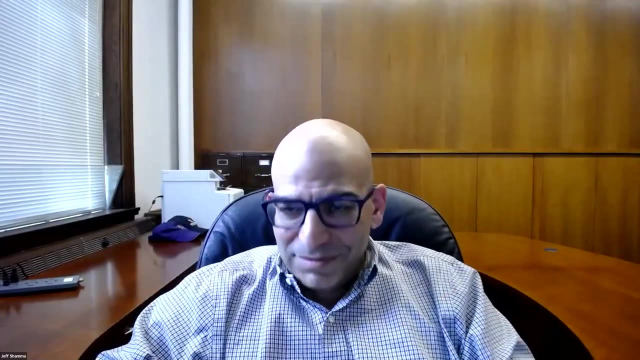 and what's the cost of cheating? Okay, I see, Okay, That's an interesting way to think about it. Instead of trying to understand when it is not possible, you can just say: you can engineer things to make it possible And how much time does it take. And how much time does it take to? 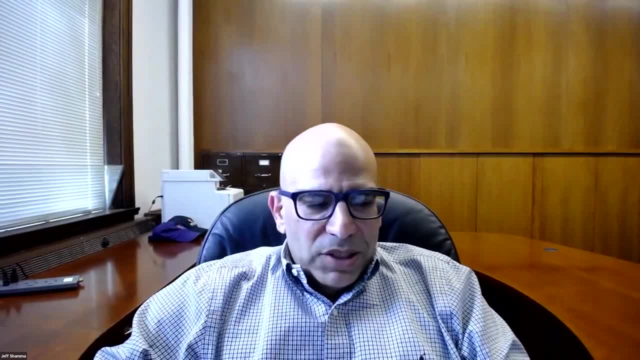 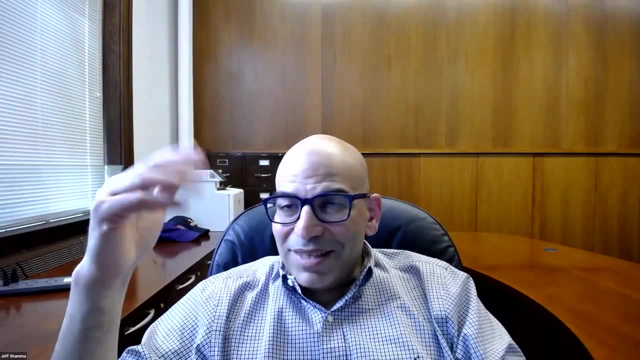 how much does it cost? That's a good way to think about it. Okay, Right. So from the game theory perspective, it's brought up in very differently that you have something called Nash equilibrium, for example. It's an equilibrium where there's no dynamics. 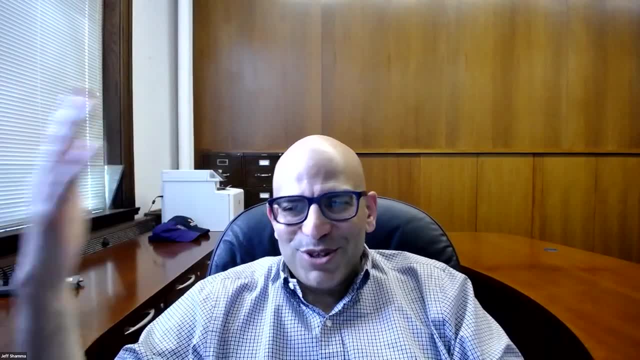 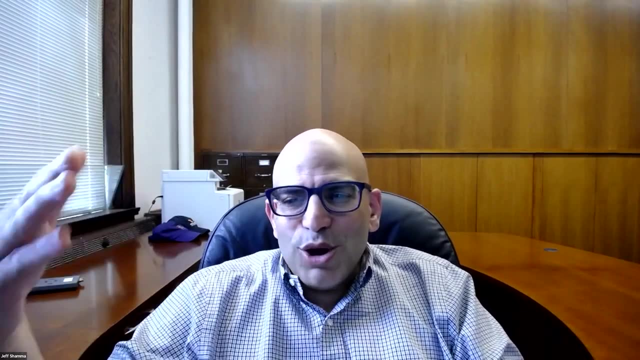 which is a very kind of curious way to talk about equilibrium. Usually you start with dynamics and then mention what's the equilibrium. So there the motivation was plausibility arguments: What is a learning story for which Nash equilibrium emerges? But it's not that Nash equilibrium is. 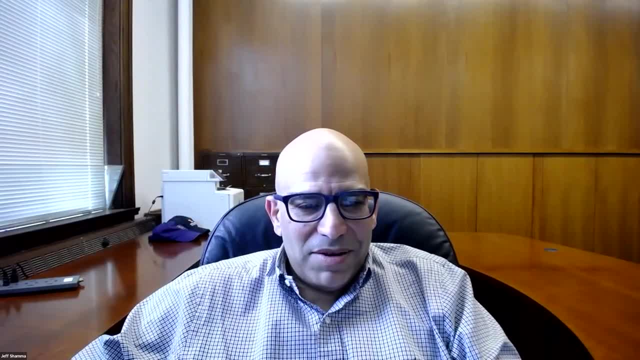 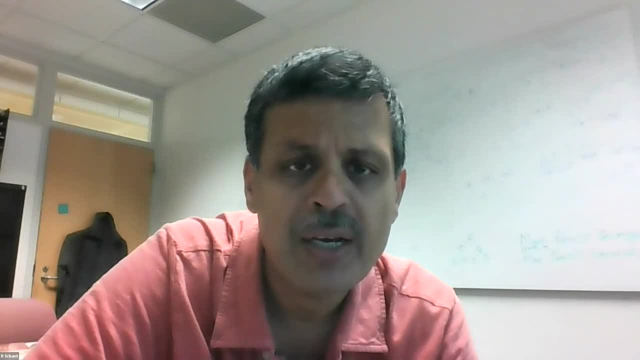 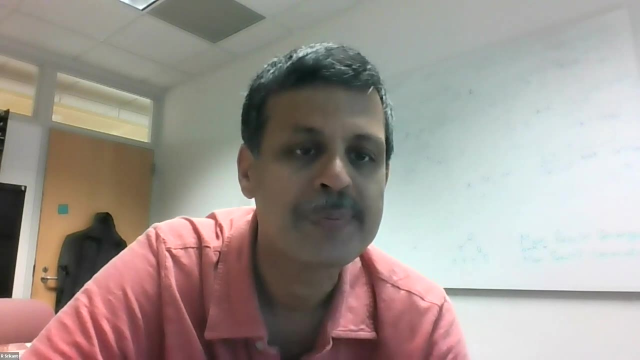 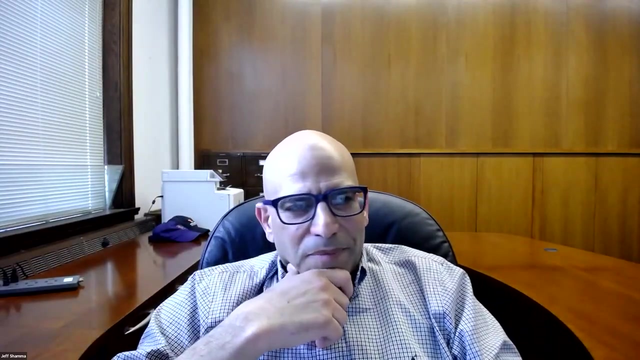 better or worse. It's just a again a backing to that solution concept. Thank you, Is there a question in the Q&A? Can you elaborate on how MDPs slash POMDPs are robustly handled with control, So let me move to use the aircraft example. Okay, And so with the aircraft example. 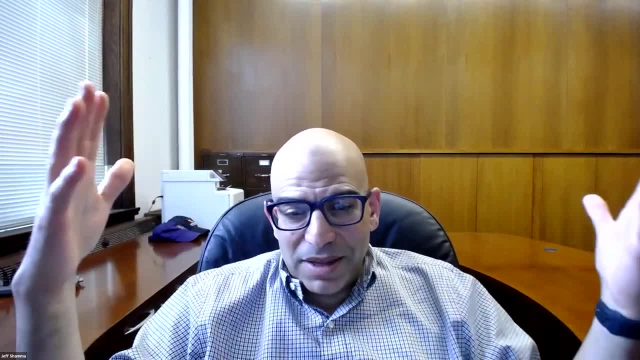 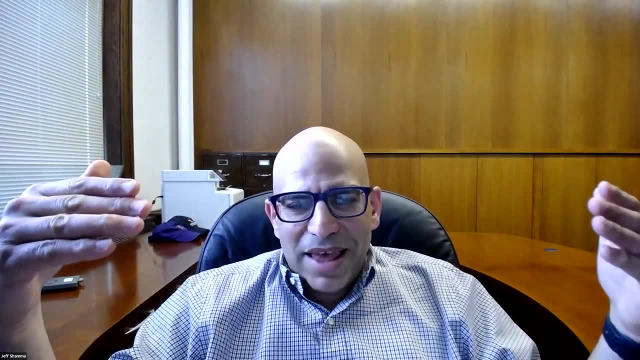 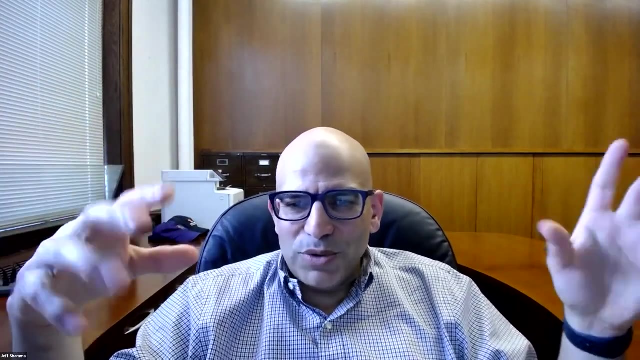 we say that there may be some parasitic like the aircraft frame might be flexible and not rigid. Generally that flexibility only manifests itself when there are certain excitations at a certain frequency. So if you take something and move it around slowly it appears rigid If you start moving it around. 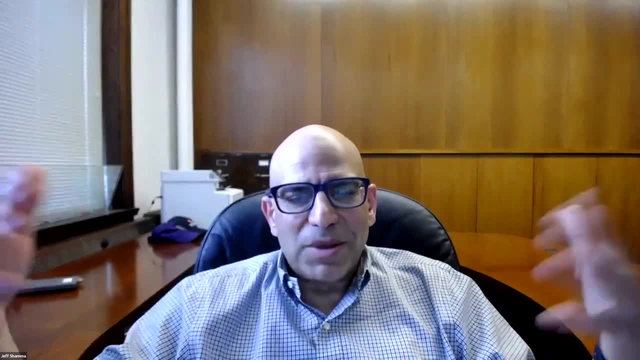 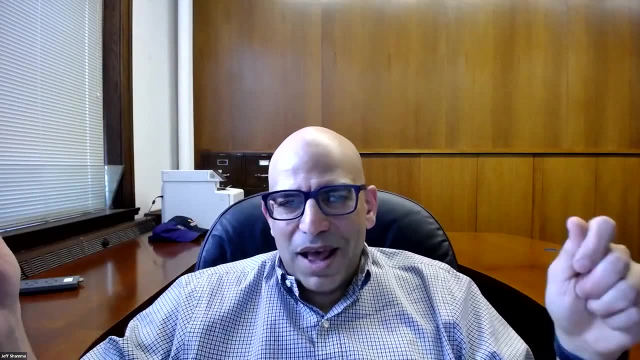 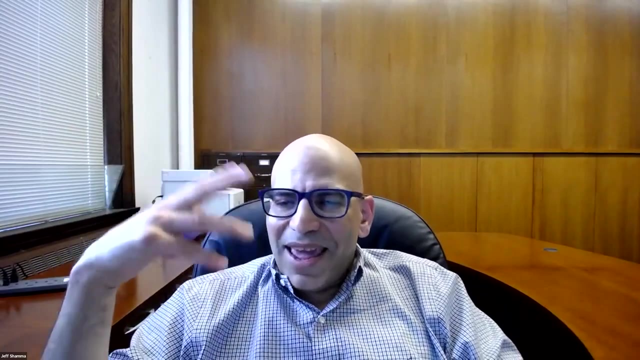 very quickly. then its flexibility becomes apparent. So when you design the control system you put in a self-limiter saying that I will not design my control system in a way that it shakes the system above, say, certain frequencies. Okay, And now there has been kind of efforts over the years to try to bring 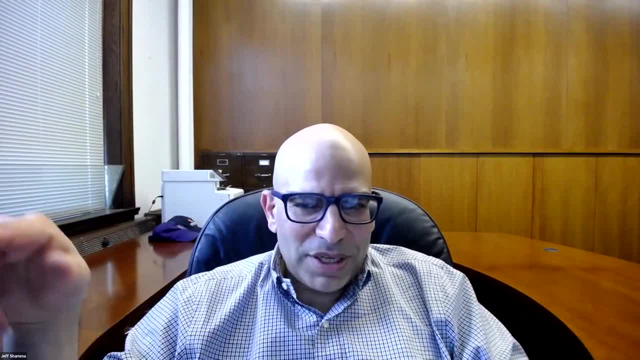 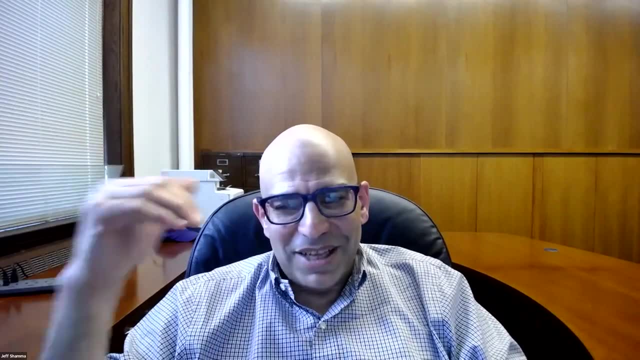 that kind of intuitive descriptions to POMDPs. But I think it hasn't been as clean of analysis, as clean of a setting. So it would be similar ideas that you want to say. I would like to be able to bound somehow the effect of the control system to the POMDPs. So that's kind of what I'm. 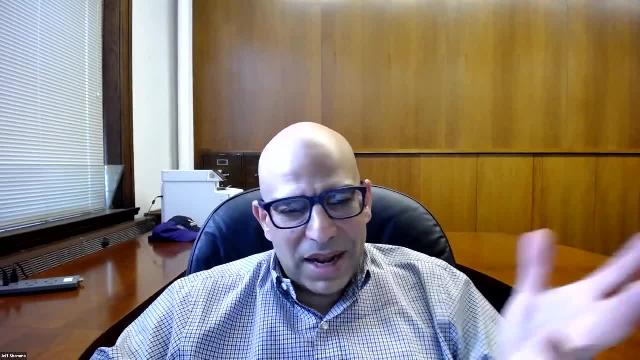 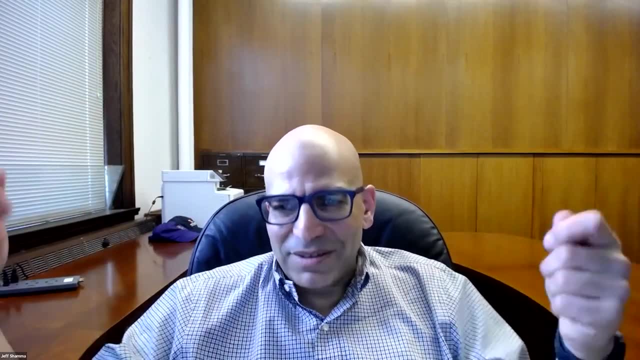 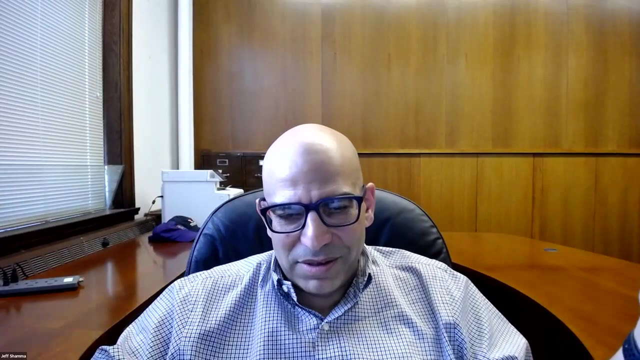 trying to do. I would like to understand the effect of all of these auxiliary states that I didn't model, But I would also like to understand what actions makes those auxiliary states start to act up, if you will, Okay. And with physical systems, they have intuitive notions of what. 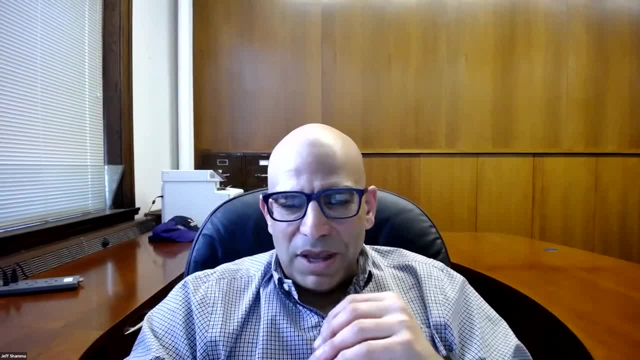 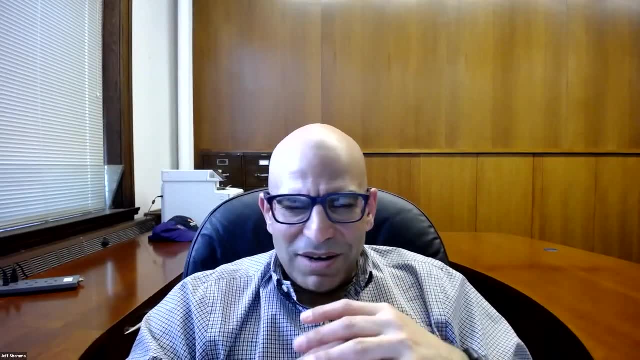 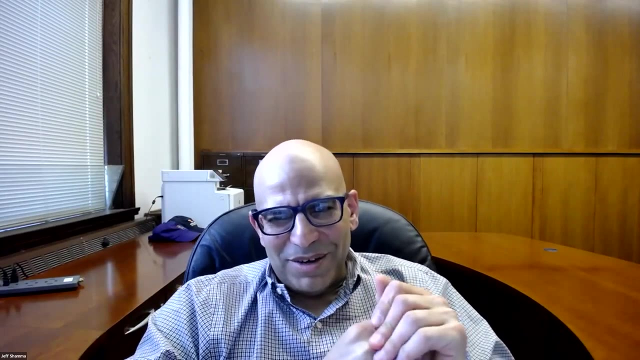 actions I need to avoid to not excite these other parasitic states. With POMDPs it's less so, And there have been attempts over the years. Srikanth, what comes to mind for you? Is there anything that's as clean as with the-. 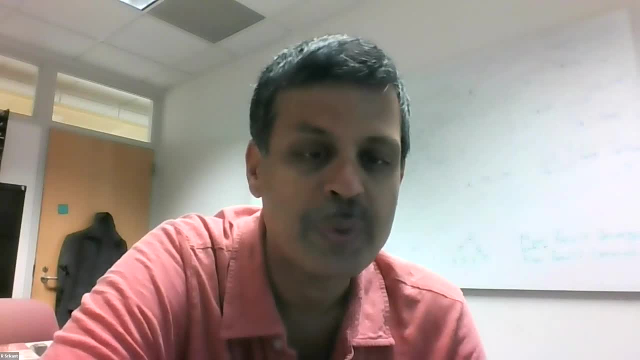 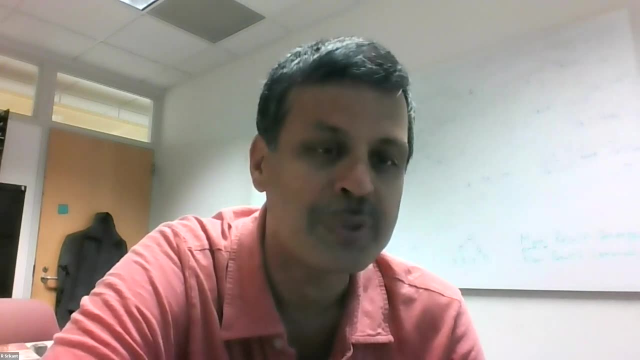 Not that I know of, but I guess that's an interesting. I hadn't thought about it this way. You can think of just the probability distribution from states to observables themselves as part of the unmodeled dynamics and try to see what one can say, whether one can say. 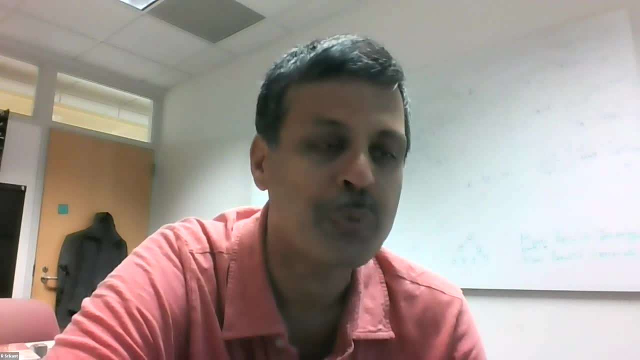 something about it. I don't think anybody has done that, but what you pointed out was an interesting way to think about it, And I think that's an interesting way to think about it- At least points to a possible way to think about it. I don't know if anybody has done it yet. It's. 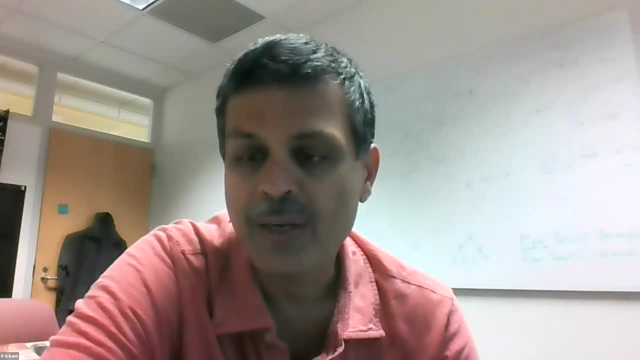 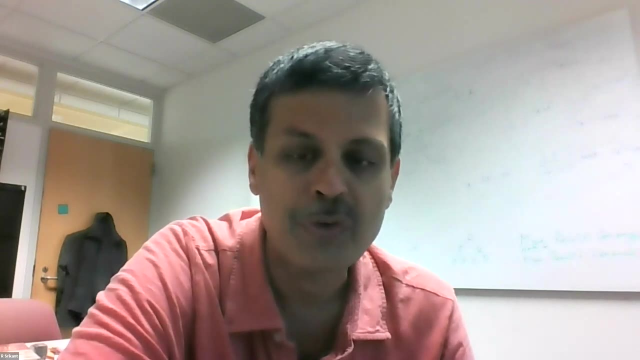 interesting. Yeah Well, I think we are at the top of the hour. Thank you very much. That was a great talk And I will look forward to seeing you and others at next week's colloquium. Bye.